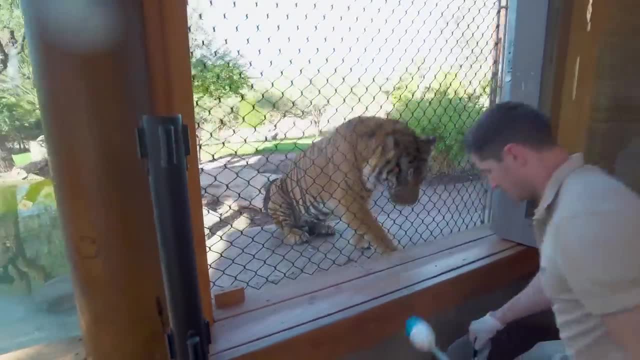 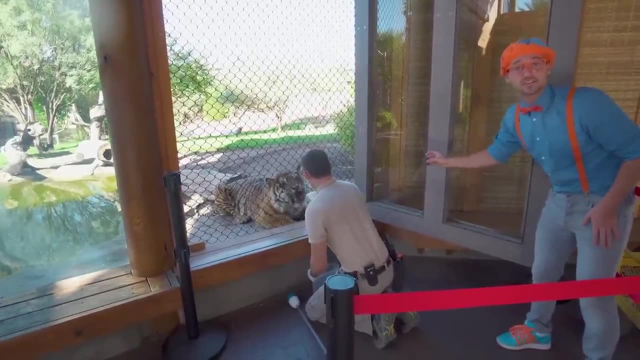 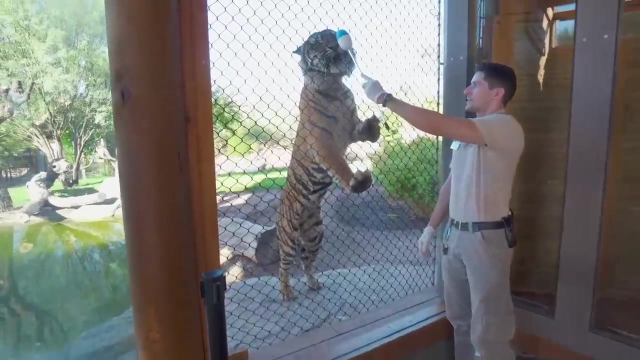 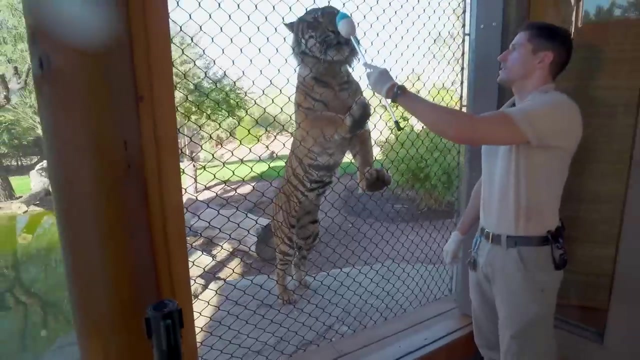 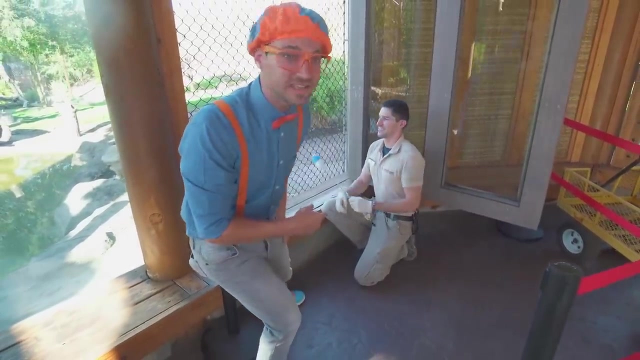 Did you see that? The tiger is doing exactly what he's saying? It looks like they're having so much fun. Target, Good, Target. Ooh, That was really cool. Did you see that? Hey, Will you tell us why we just did that? 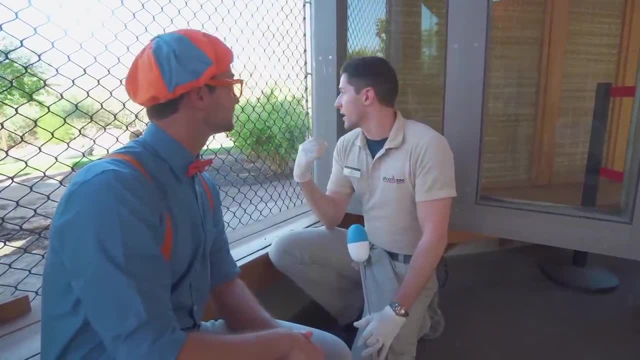 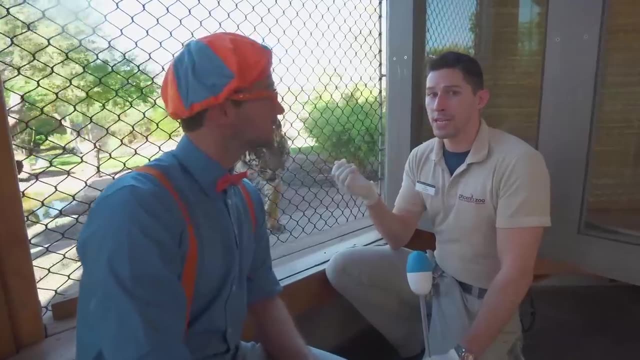 Yeah, So we train our animals so that they have the opportunity to make things easier for them and the staff. So we don't train our animals to do tricks, We do what we call behaviors. So, for example, when I was having Jay target his nose to the end of this pole, 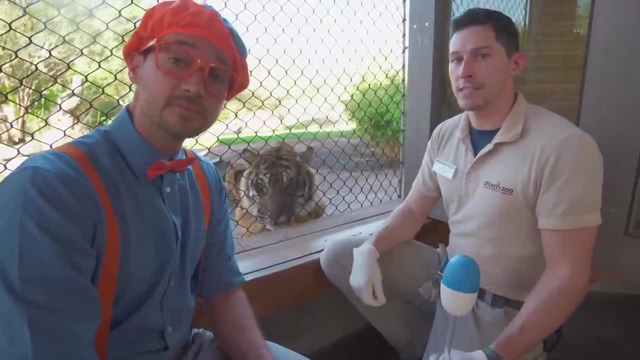 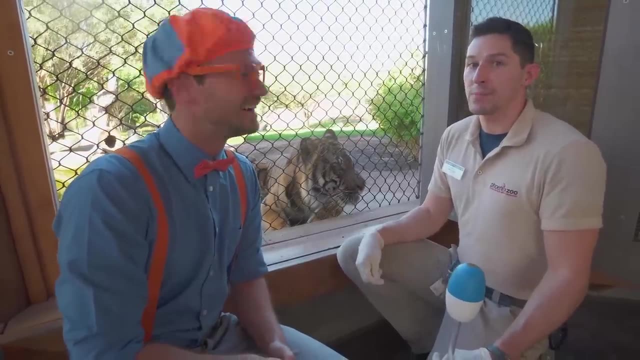 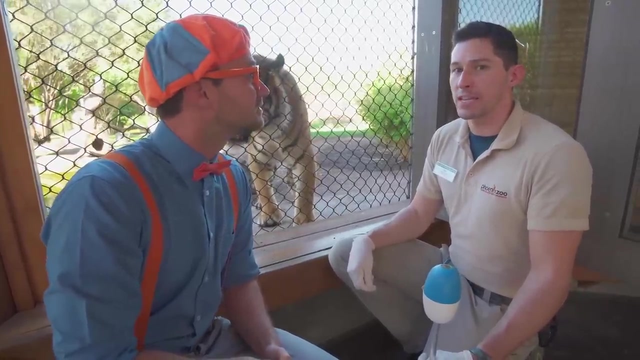 it allowed me to move him to different positions so I could see different parts of his body. Having him stand up is not only impressive to see how big a tiger is, but it gives me the chance to see his underside Because, just like us, they can get injuries like cuts and bruises. so it lets me check up on his body to make sure he's still feeling good. 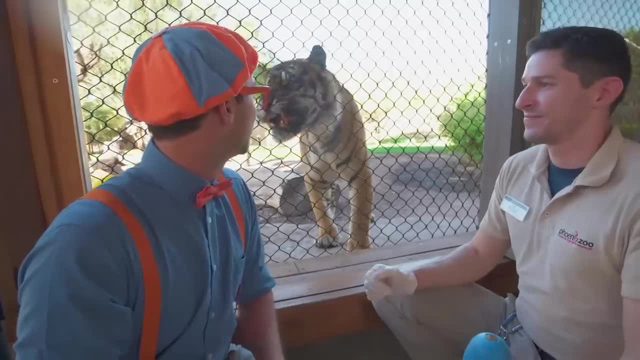 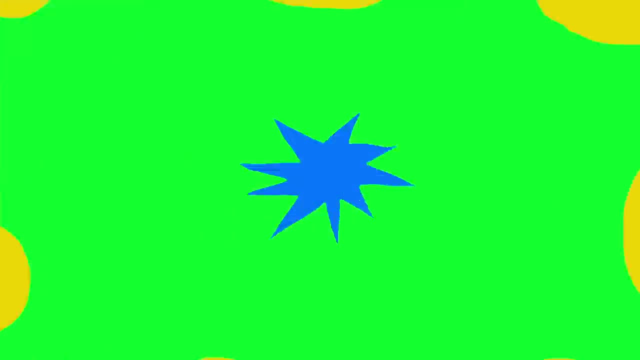 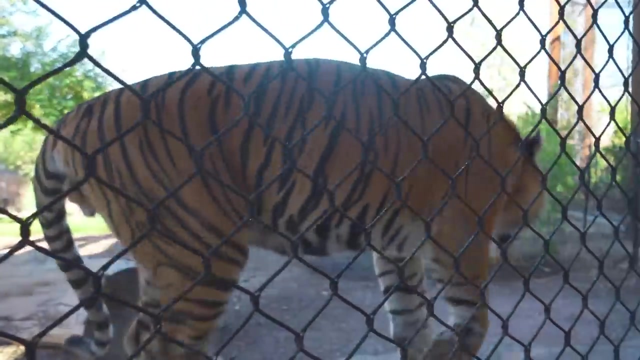 Ooh Well, thank you so much for showing me what you just showed me. You're very welcome. Alright, See you later. Thanks, Let's go see some more stuff. Whoa, Do you see that animal? It's another cat. This is a jaguar. 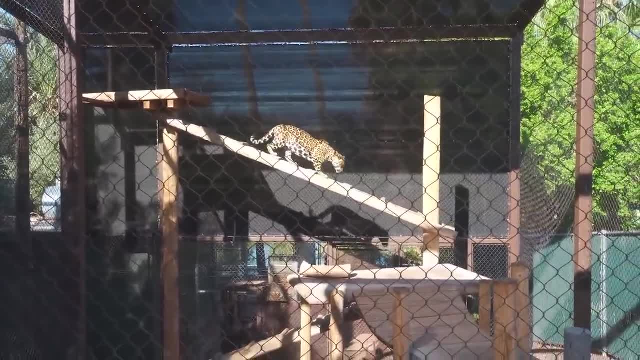 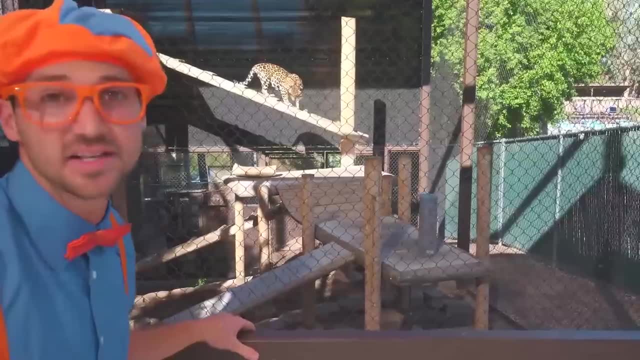 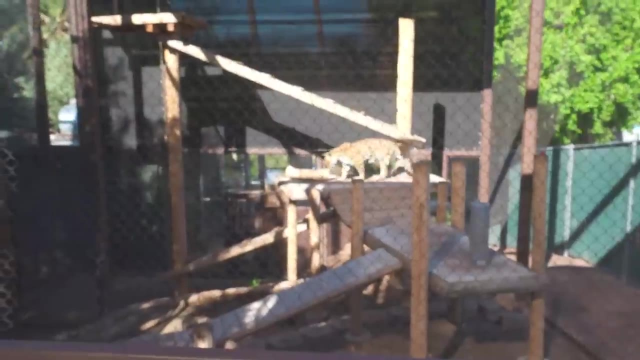 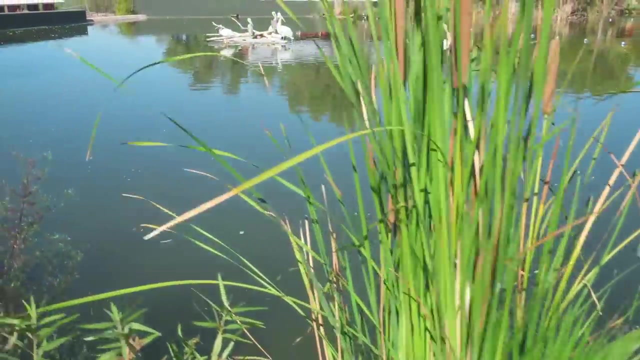 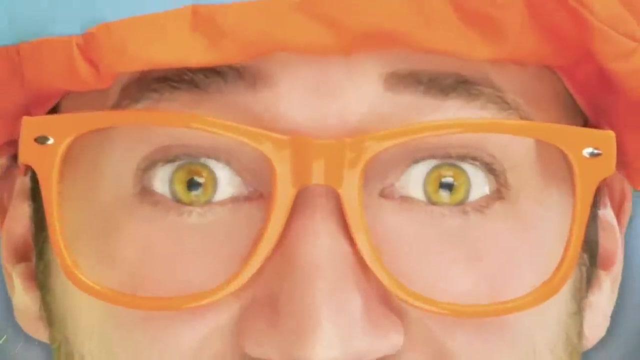 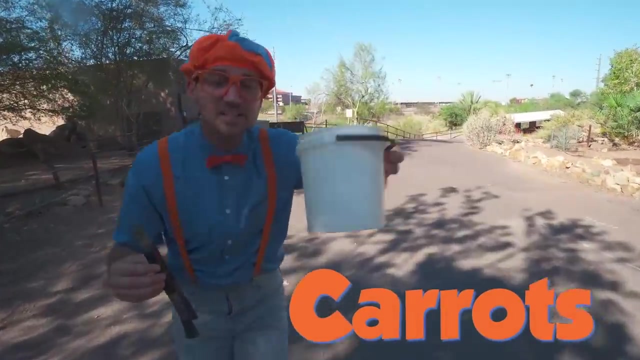 Whoa, Do you see that animal? It's another cat. This is a jaguar. Whoa, Ooh, check it out. I have a pail of carrots and some tongs and we just got told we need to feed the next animal. Come on. 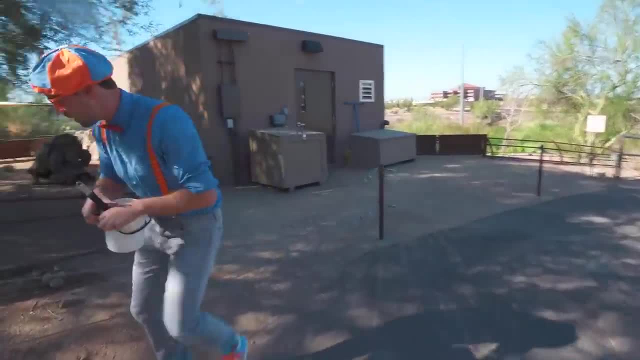 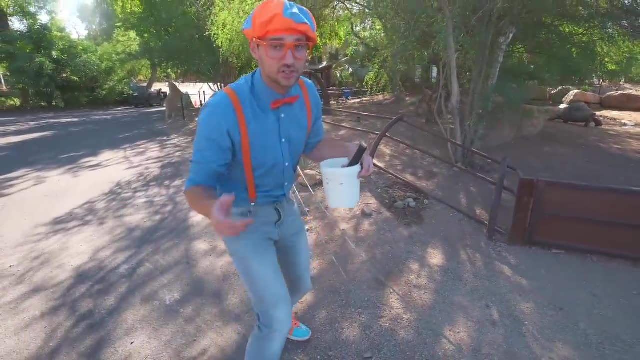 Whoa. Hey Come, geral, Come be my pet. Hey, come in, Gerald. Hey, check it out. These are cables that you have to be on this side of them. But we just got permission to head inside so we can feed the animals. 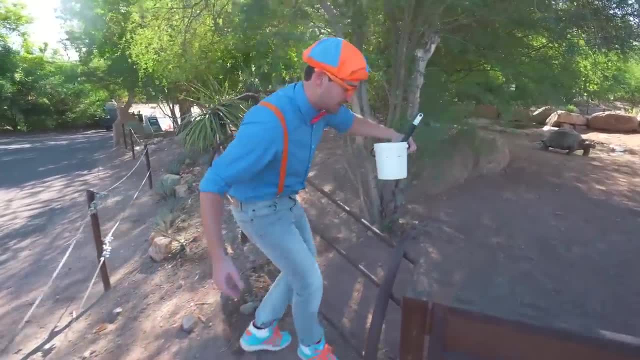 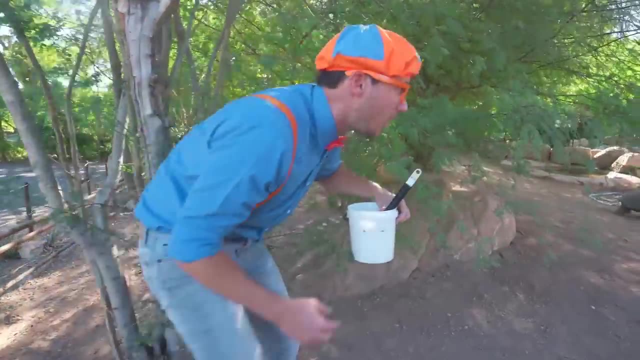 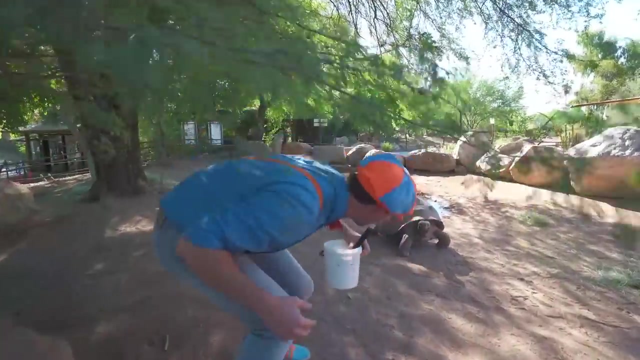 Let's go. Okay, this is a short barrier Interesting. That wasn't too hard to get in. Oh, I see the animal. Look, Let's go through the trees. Whoa, Hey, look Look at the animal. we get to feed. 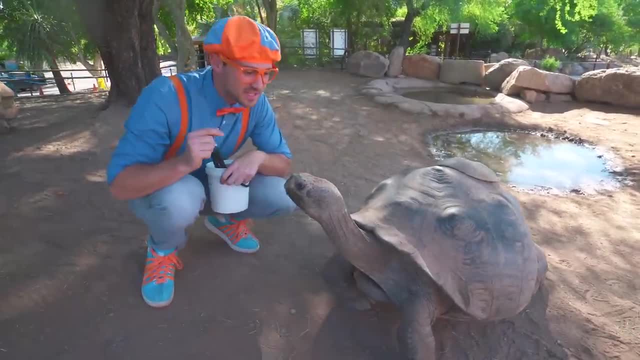 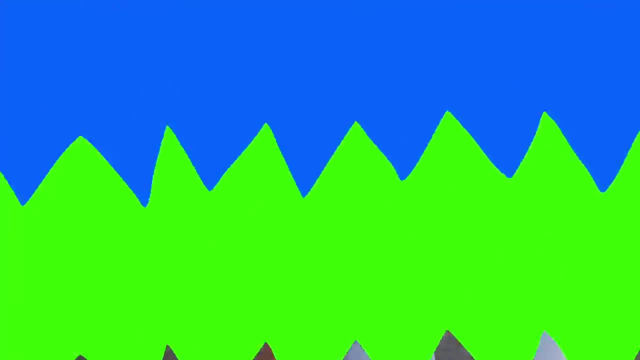 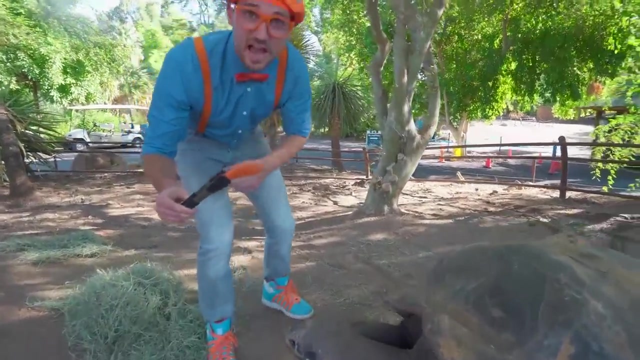 Check it out. Oh, do you know what kind of animal this is? This is a tortoise. Let's feed the tortoises. Yeah, Check this out. This is a carrot, And I'm using tongs because tortoises have really strong jaws. 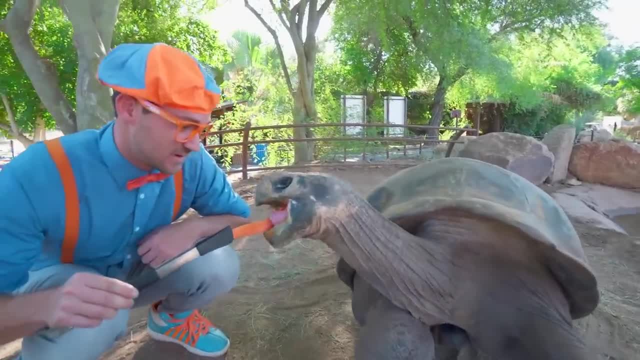 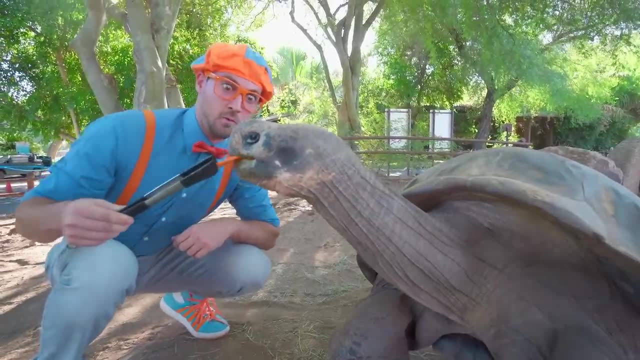 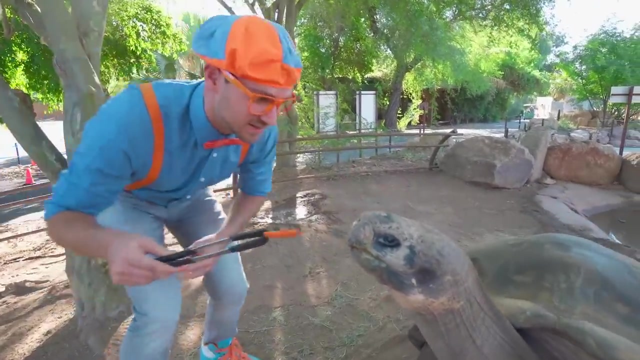 It might bite my finger off. Here you go. Whoa, Oh, whoops, it slipped. Here you go. Whoa, Okay, would you like a little bit more? Yeah, Okay, here you go. Oh, there you go. 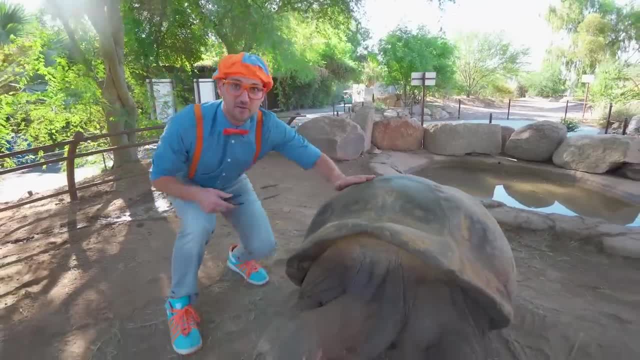 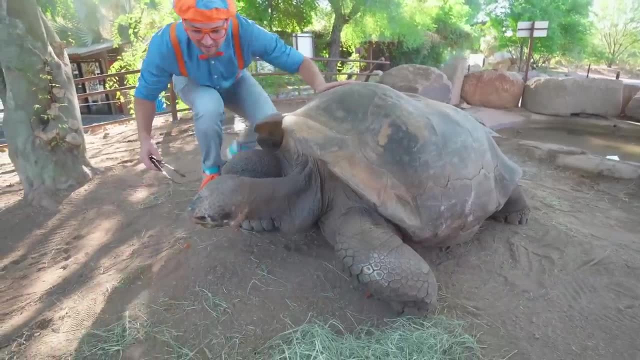 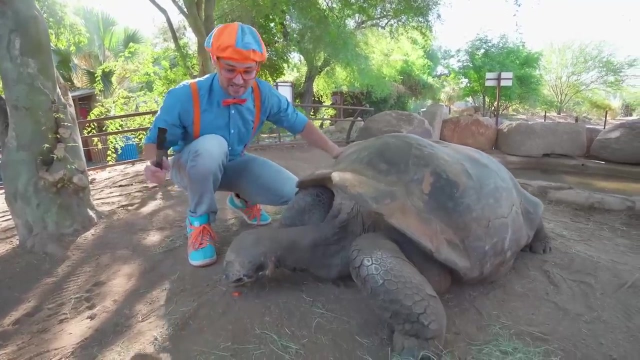 Whoa, This tortoise is about 550 pounds. Whoa, That is really heavy. Hey, And guess how? Let's see how old he is. Oh, he's 66 years old. Oh, that's really old. Oh, hello. 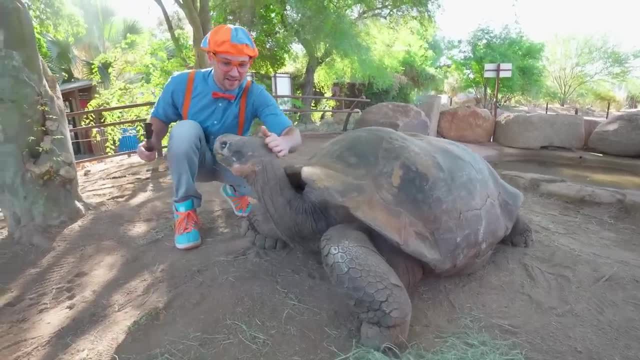 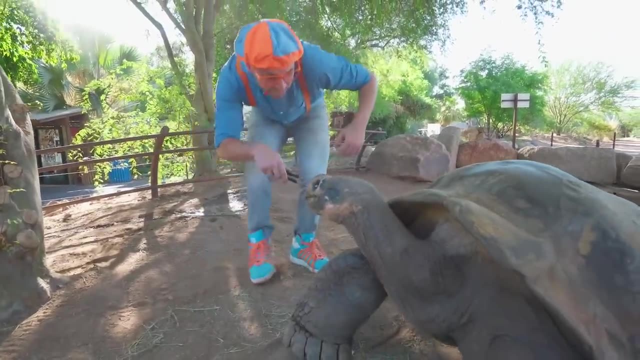 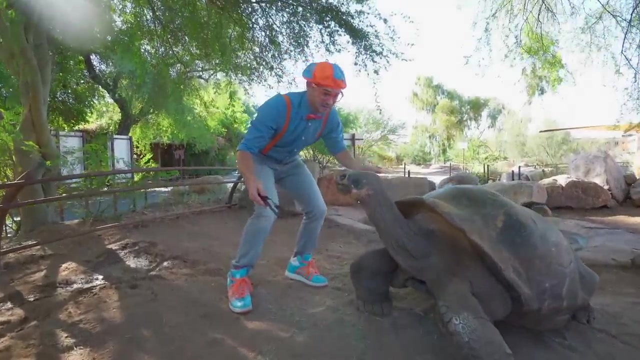 Hey, check this out, I'll pet this tortoise's head. Hello, How are you? Whoa, Whoa, Look, the tortoise is off the ground. Do you see that? Because that allows for all the bugs and everything. 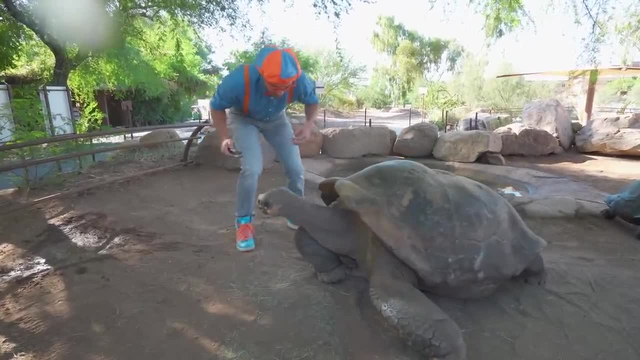 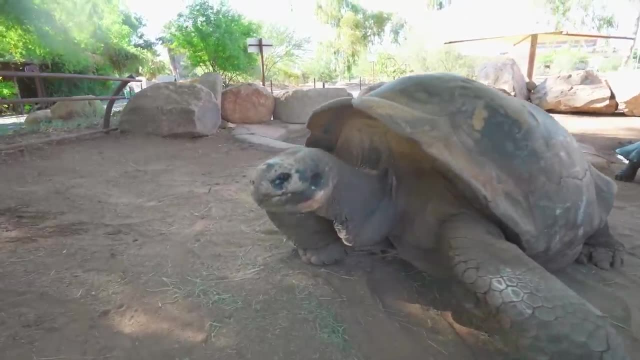 To get away from it's underneath area. Whoa, Okay, let's go get some more carrots. Whoa, Hello, How are you doing? Are you having a good day? Ooh, check it out. See this tortoise. 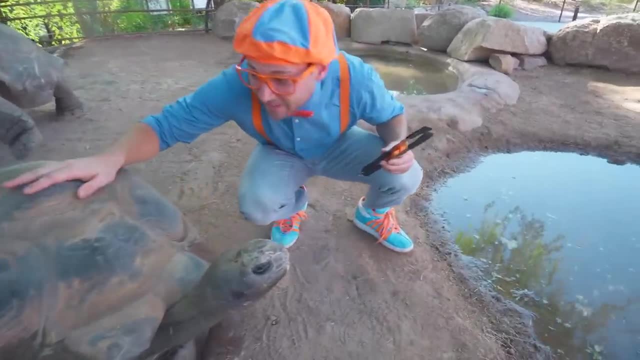 This tortoise is a Galapagos tortoise And it's a female. Oh, Oh, there you go. Oh, and here comes the male. Whoa, Do you see how big he is? Yeah, Yeah, Whoa. 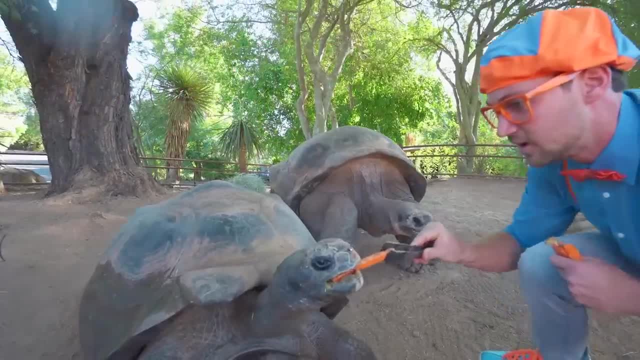 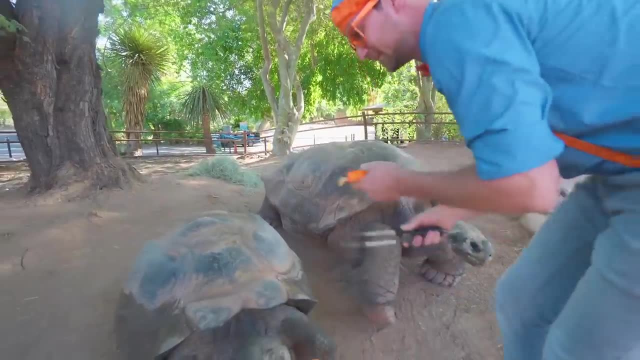 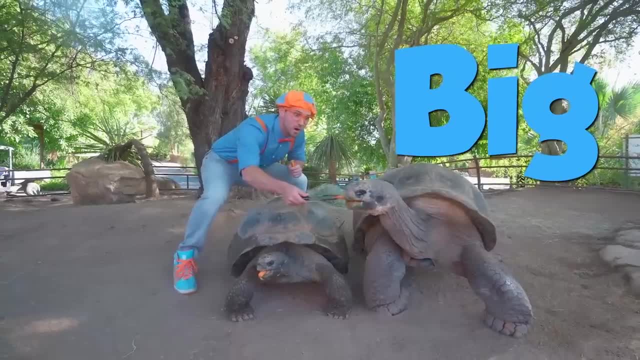 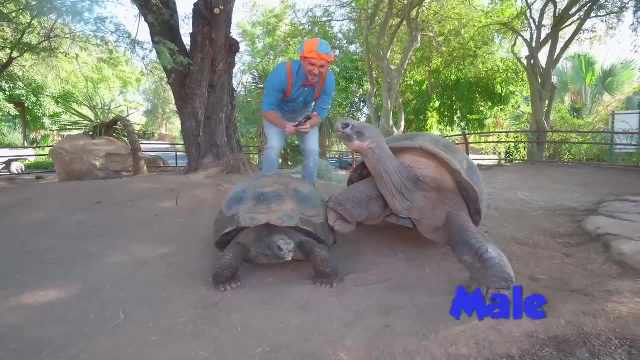 Okay, I'm going to loop right around here. See how this one's a little smaller And this one is bigger. Whoa, This is a female And this is a male. Whoa, Hey, Do you two like each other? 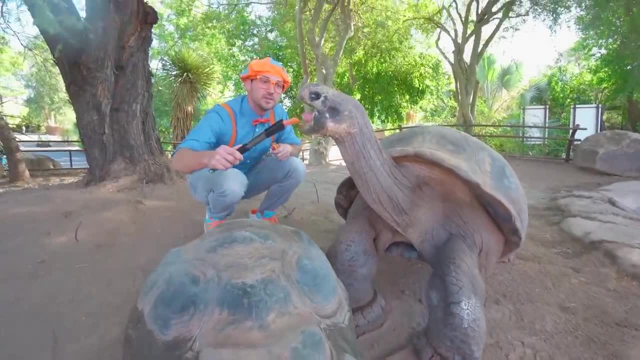 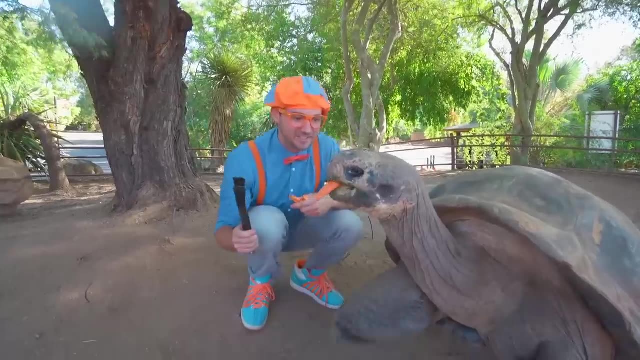 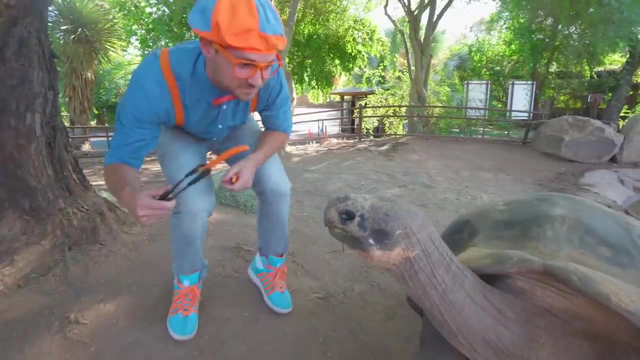 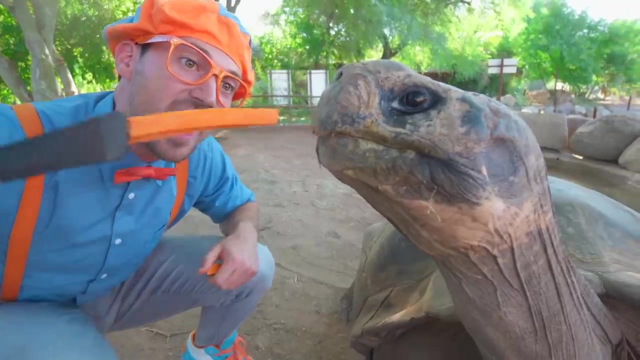 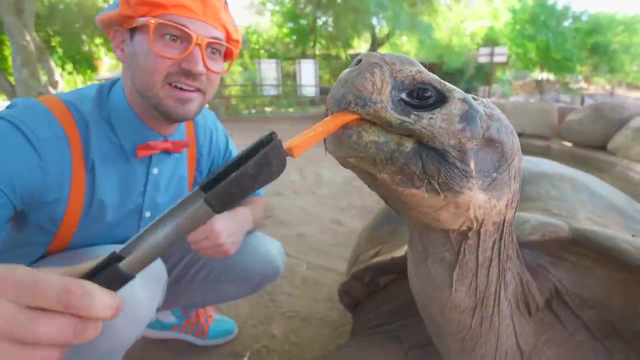 Yeah, You two look like your friends. Whoa, Oh, Whoa, whoa. good job. oh, you dropped it. hey, come a little closer. okay, here you go, all right, open wide. here comes the carrot. whoa, there you go, is that yummy? 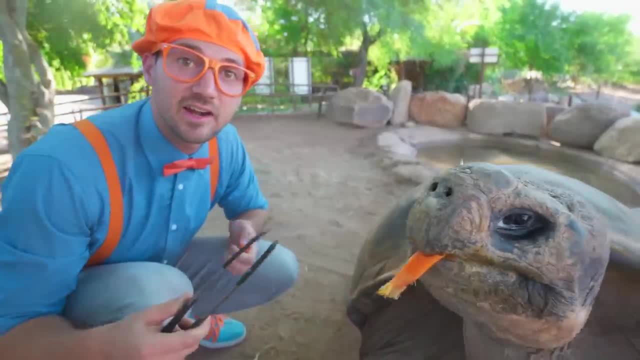 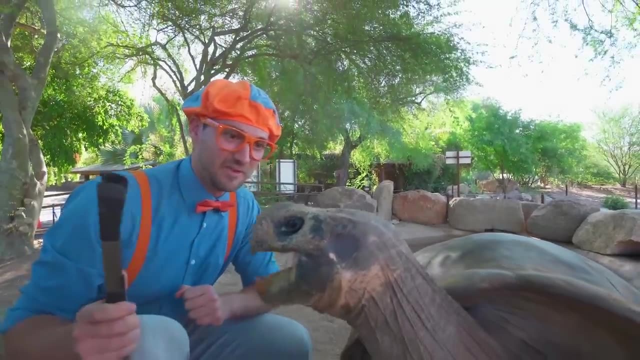 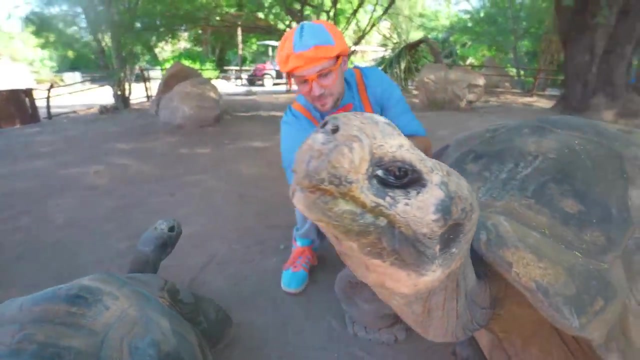 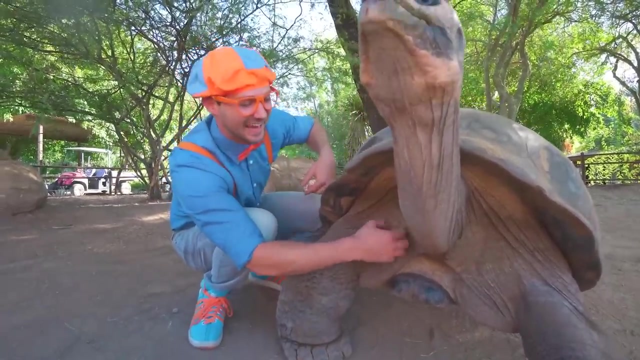 Hey, tortoises, like carrots, just like how I do, and carrots are nice and healthy. there you go, whoa, you have a big mouth. whoa, look, I'm giving this tortoise a scratch. see how does that feel? does that feel good? yeah, do you see how the tortoise is standing? 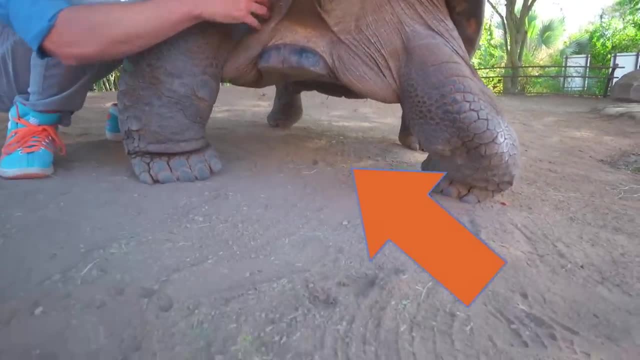 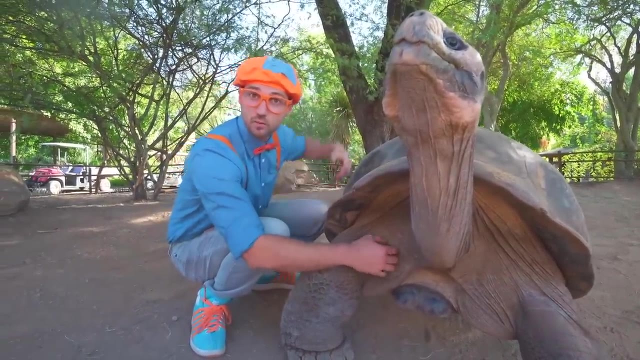 on its legs really high in the air In the wild. they do this because a lot of times they have bugs underneath them and this allows for the finches, which are birds, go go to fly underneath there and then. 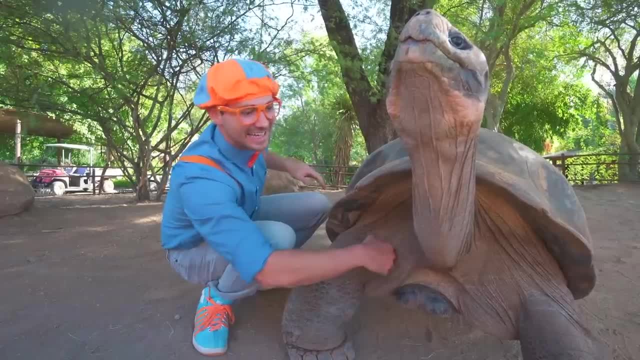 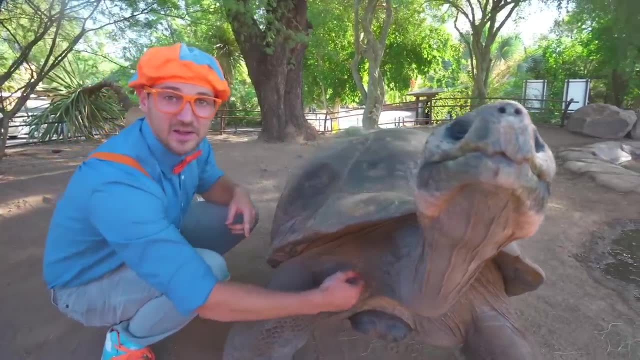 eat all of the bugs underneath this tortoise? yeah, but for now he's standing on his legs because this feels really good. it's kind of like when a grown-up gives you a back scratch. yeah, I like when my mom gives me a back scratch. 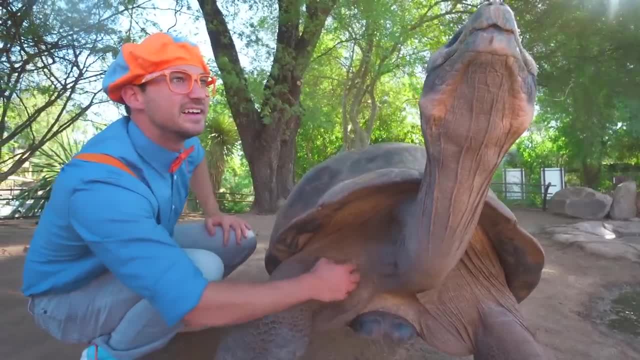 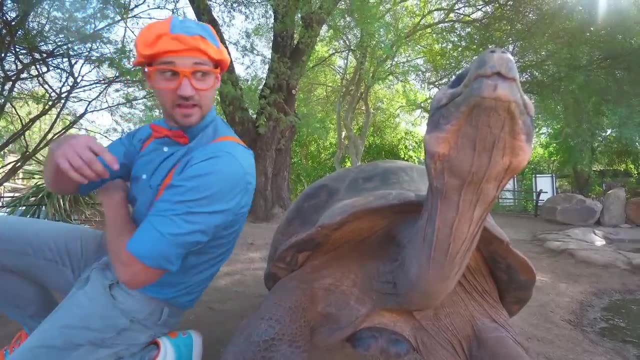 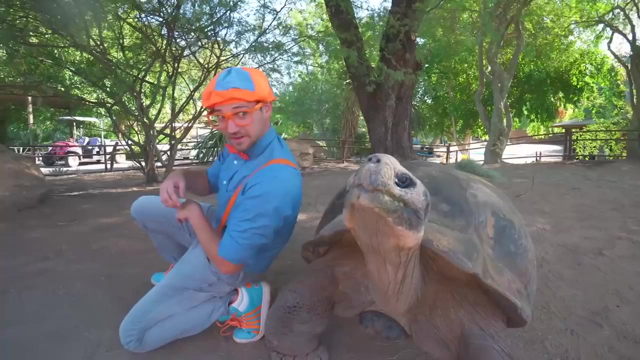 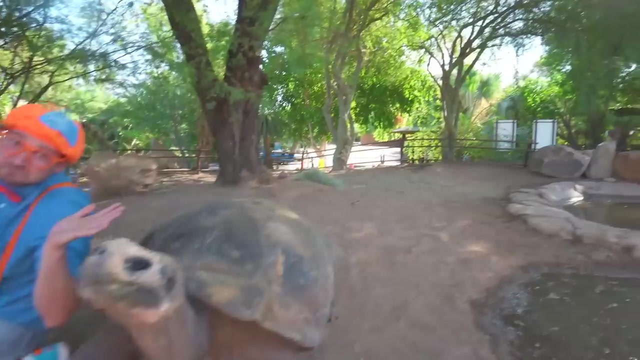 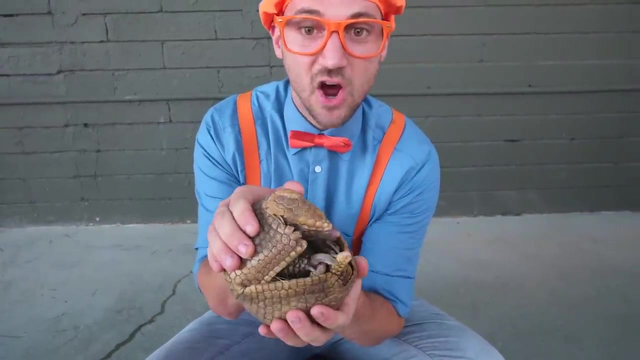 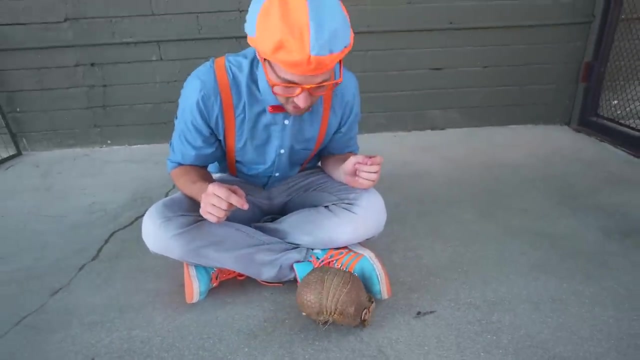 Yeah, how does this feel you like that? yeah, okay, my turn. okay, my turn, I'm ready, I'm ready. Oh no, Ooh, check this out. This is an armadillo. okay, here you go, run free. whoa, look, an armadillo is one. 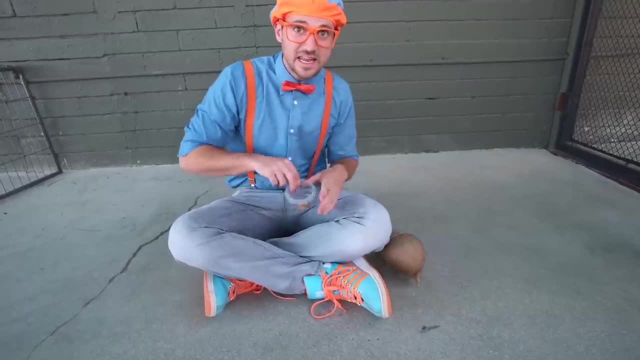 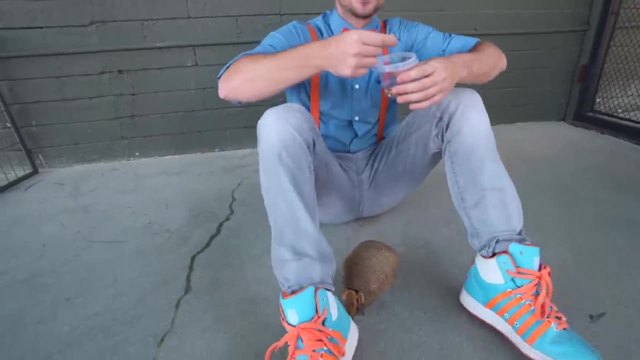 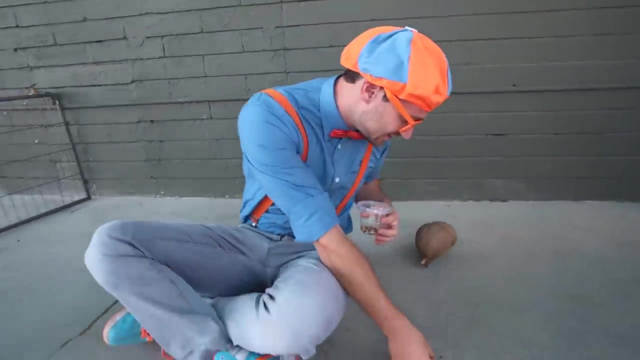 of the ambassador animals at the zoo. that means it's an animal that you can meet face to face. whoa, hey, what are you doing? you want a treat? armadillos love mealworms- here you go. uh-oh, hey, come right over here, here you go. 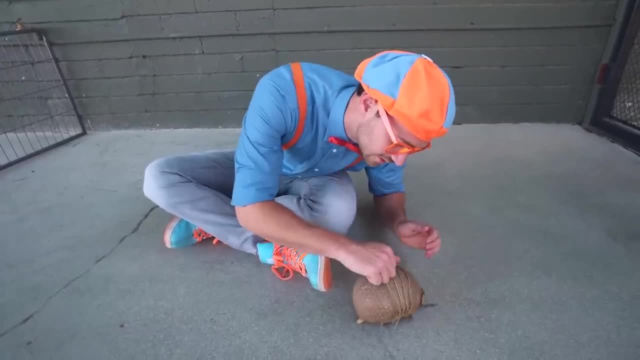 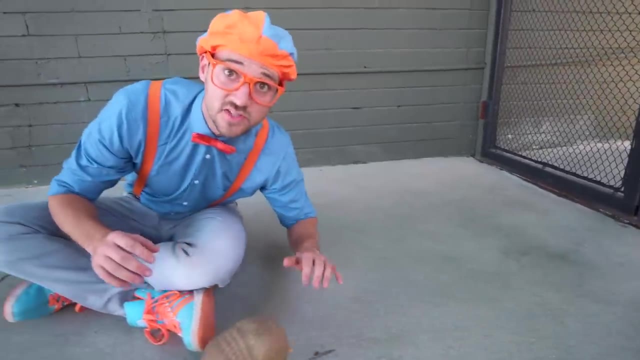 Look, doesn't this armadillo look hard? yeah, it is kind of hard, and it's not a shell, it's bone inside the armadillo's skin. whoa okay, ooh, this is princess buttercup, ooh. 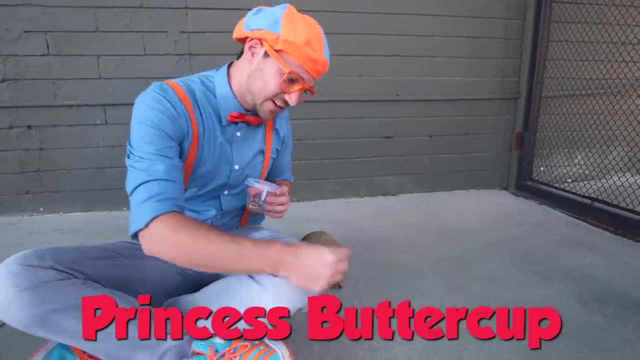 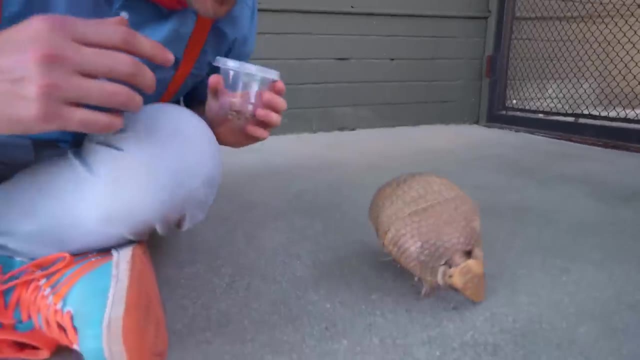 alright, here you go, here you go. princess buttercup: ooh, look at princess buttercup's pretty little nails. whoa, okay, run free. Well, until they get to the bottom of the tree, they'll be ready to go. there they are. 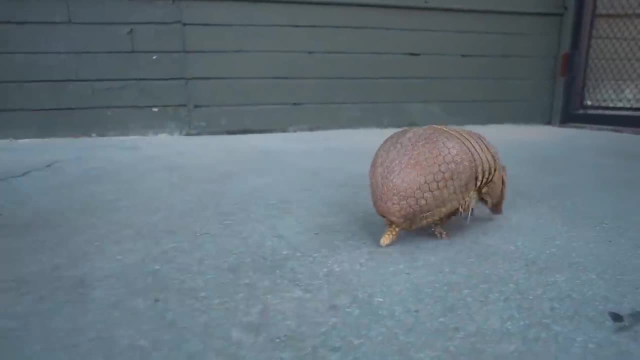 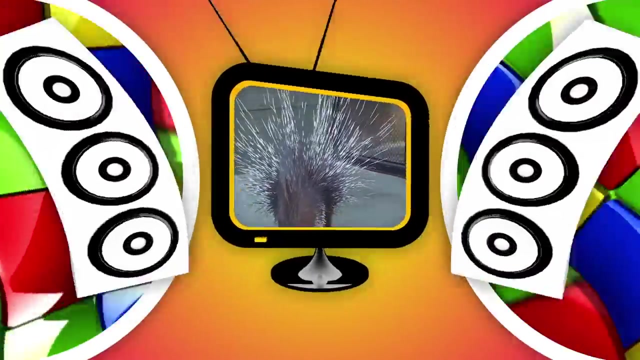 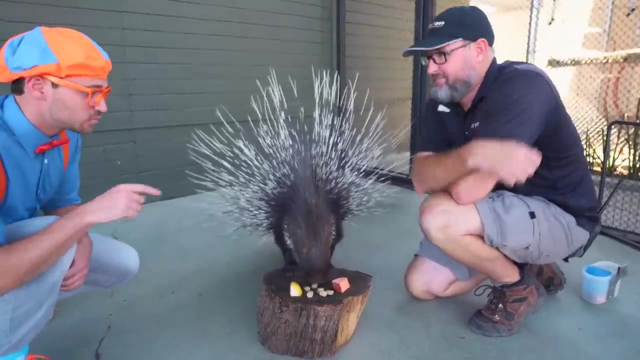 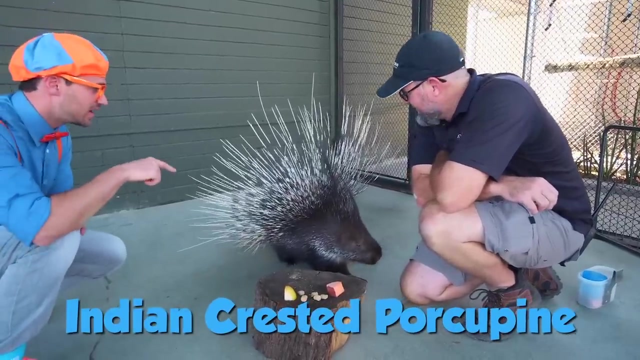 they're doing it. whoa, Run free. Whoa, Look at this animal. What kind of animal is this? This is an Indian crested porcupine. Whoa, Look at all of its spines. Are those spines? 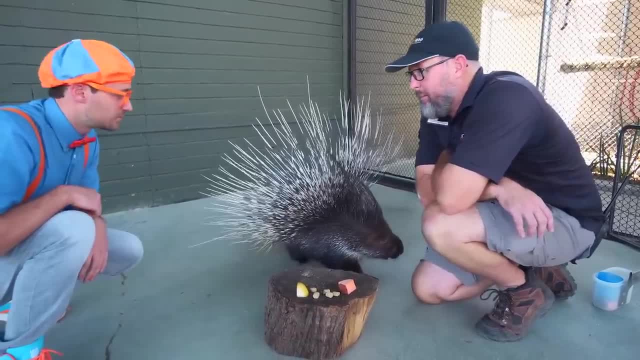 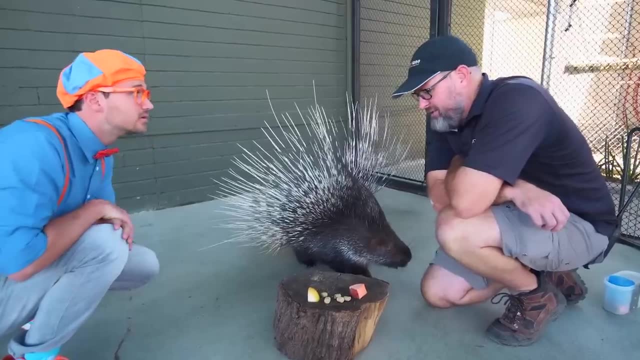 The big ones are just to make her look scary, but the dangerous ones are down by her tail. Oh, okay, down there, Whoa. And what is she doing right now? We're just enjoying some snacks. She likes a lot of plants. 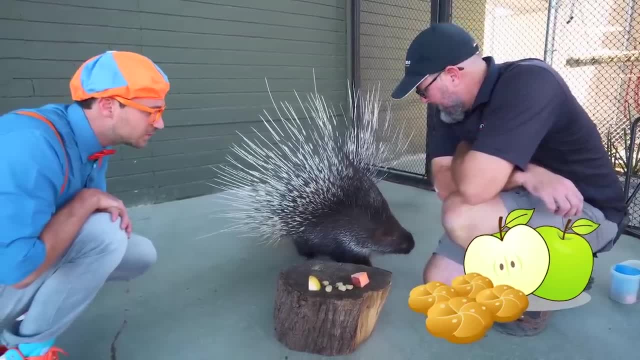 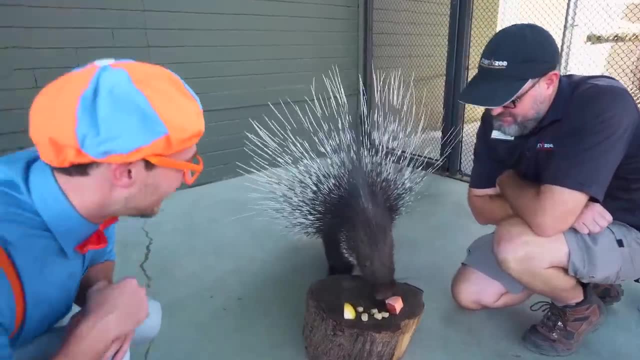 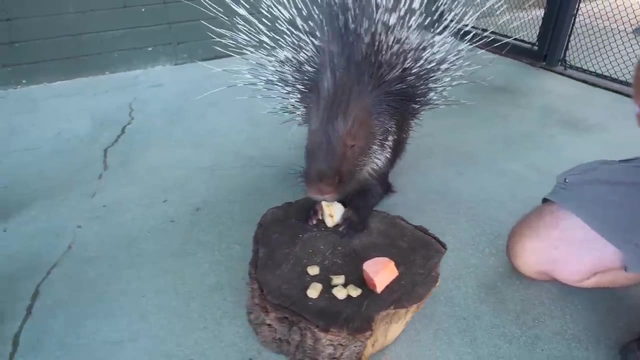 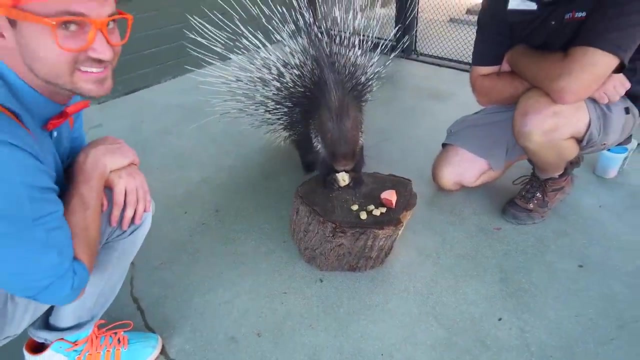 so we've got her some biscuits, some yam and some apple today. Ooh, that sounds pretty tasty actually. Ooh, let's take a closer look at the porcupine. Wow, you don't want to touch this animal on its tail. 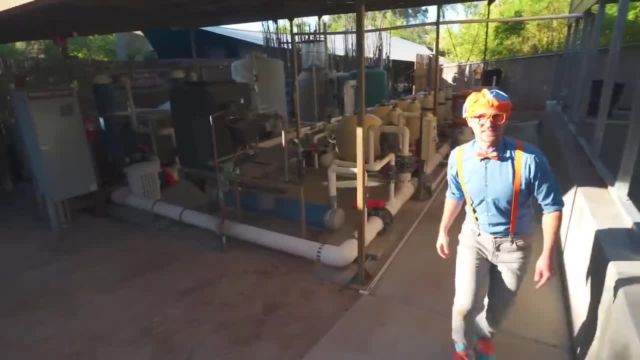 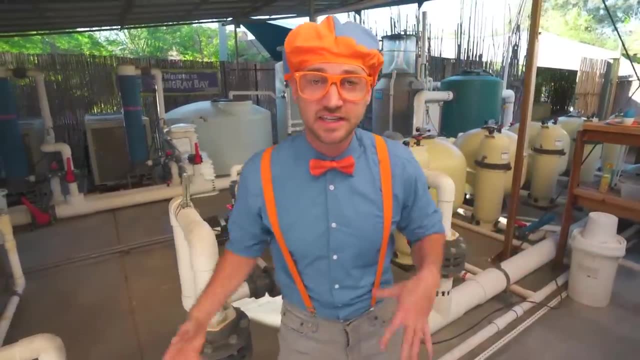 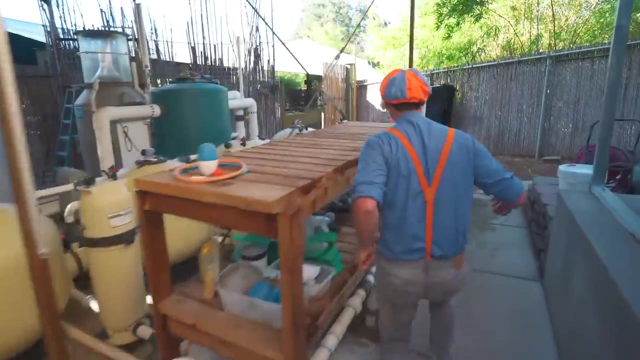 Whoa, check this out. This next area is really cool. Whoa, do you hear that All of these things are working really hard to keep this next area exactly like how the ocean is? Come here, Whoa, look at it. 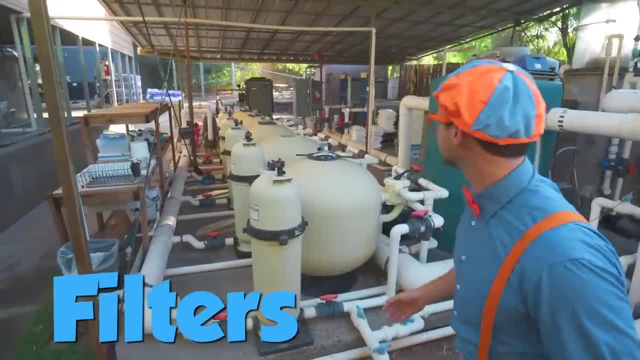 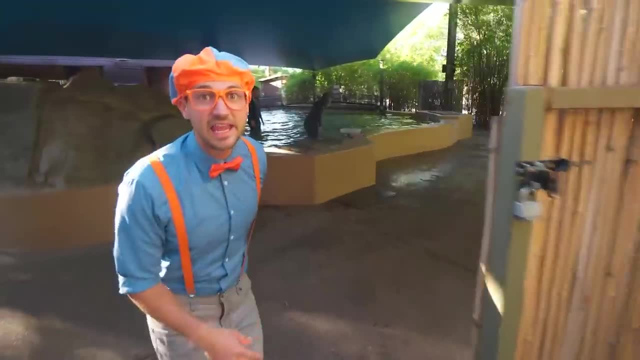 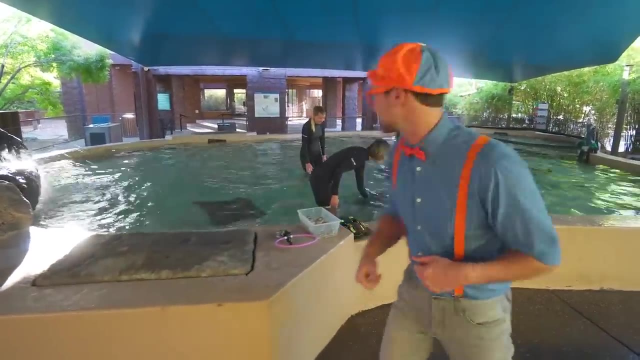 Whoa, there's so many filters and other things. It's so cool. Okay, come over here, Let me show you what it's doing. Yeah, this is stingray bay and they're training the stingrays to do some pretty cool tricks. 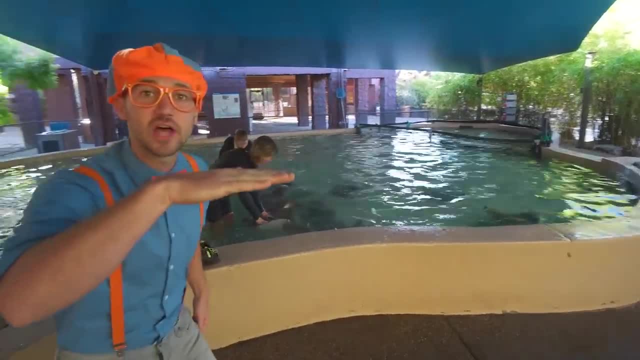 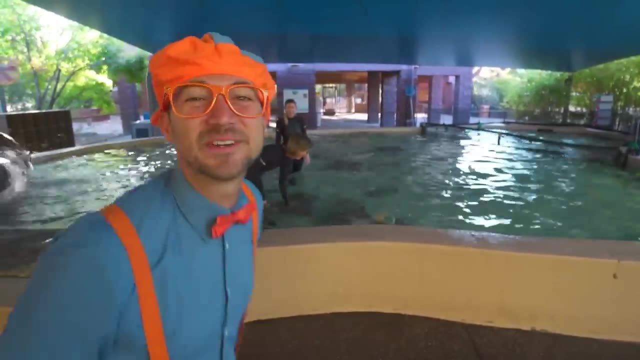 If you come to this zoo, you can use a flat, gentle hand and touch the stingrays on their back, but they're letting me go inside. I'm so excited. Okay, first I need to take off my shoes. One shoe. 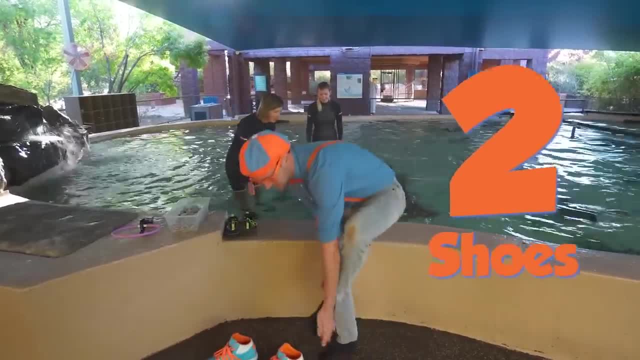 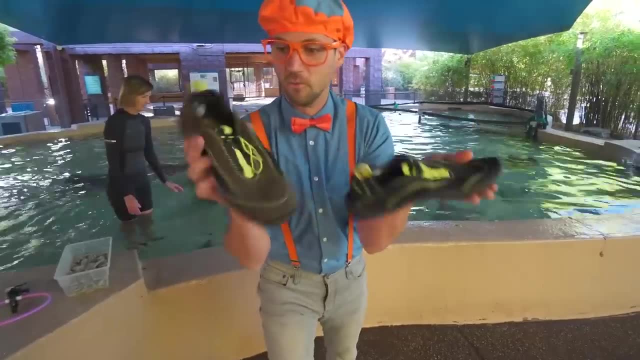 Whoa, two shoes. Okay, let's put those there. Can't forget about the socks, because I'm going to put these on. Whoa, they're like water socks or water shoes. Okay, let's put them on. 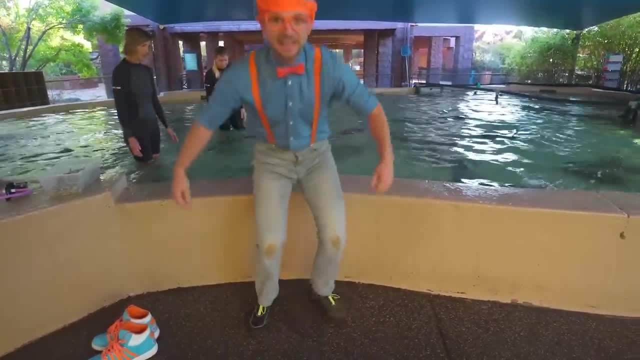 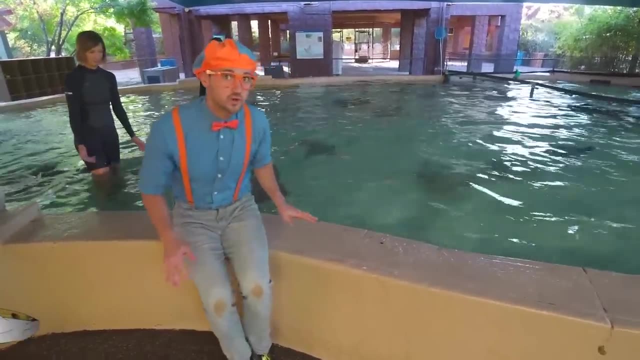 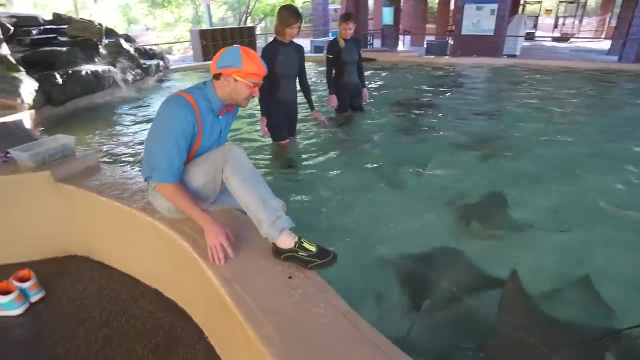 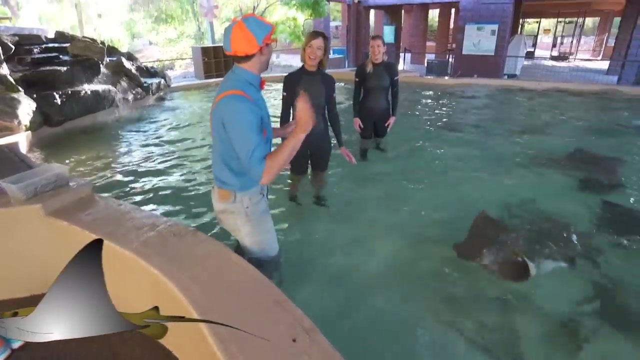 All right, Okay, okay, I'm ready, Here we go. You have to be nice and smooth and slow so you don't scare them. Whoa, the water's nice and cold. Okay, whoa, okay, Hi, How are you? 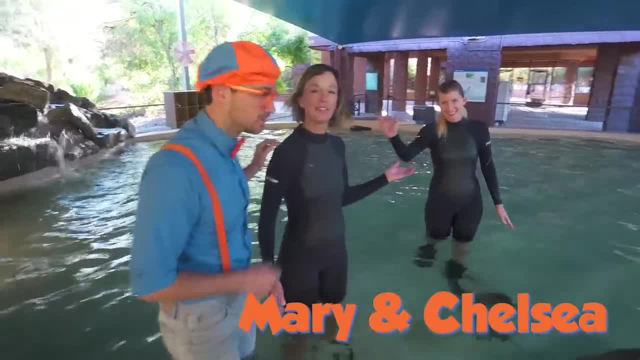 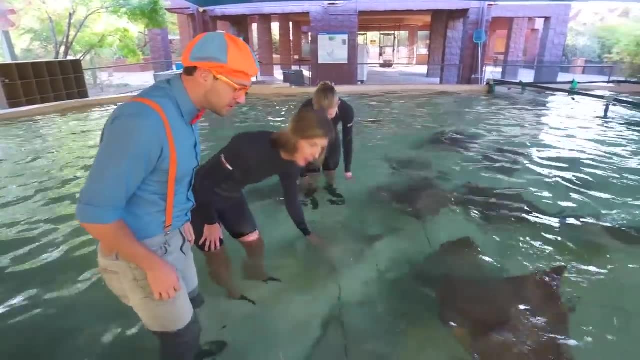 Good, how are you Good? what's your name? My name is Mary and this is Kelsey. We work here at the Phoenix Zoo. Ooh, so what are you doing right now? So, right now, we're giving breakfast to our stingrays. 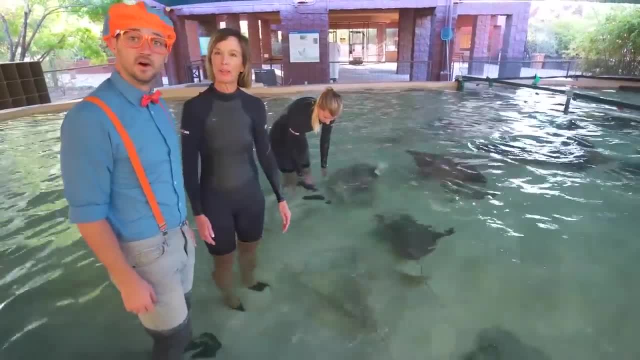 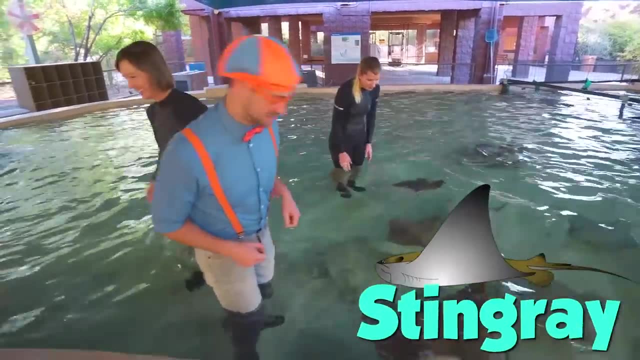 and we're checking them to make sure everybody's healthy and happy this morning. Ooh, that sounds like fun. Can I help? Sure, would you like to feed some? Ooh, yeah, let's feed the stingrays. So they have shrimp and smelt. 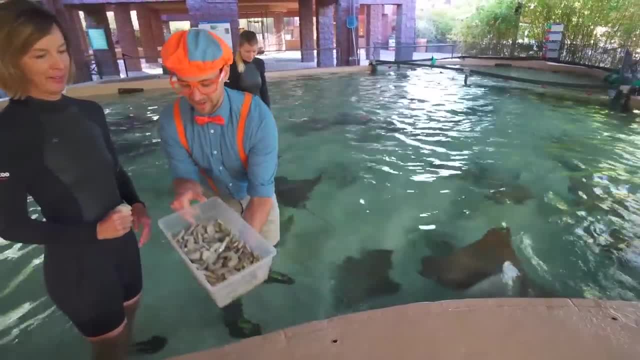 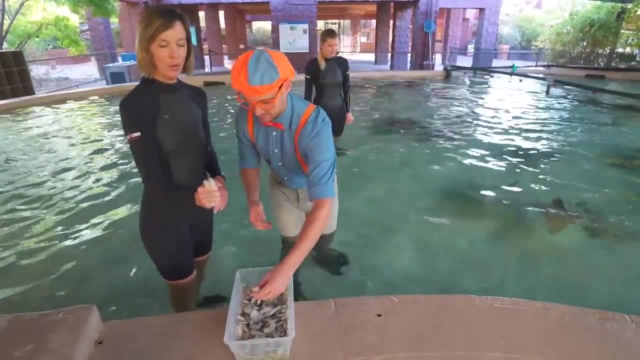 so you can take a couple and you can put it in your hand. Okay, check out the food. Whoa, it looks so tasty. Okay, I put it in my hand. You're gonna hold it like an ice cream cone. 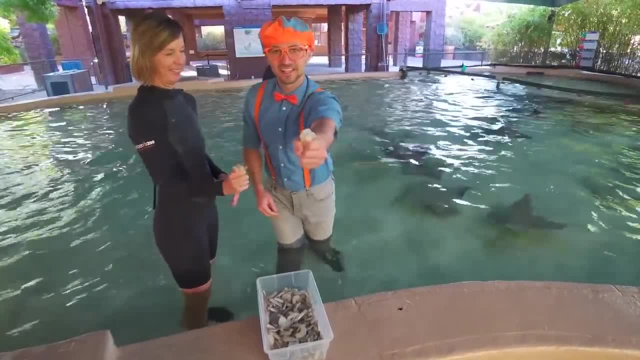 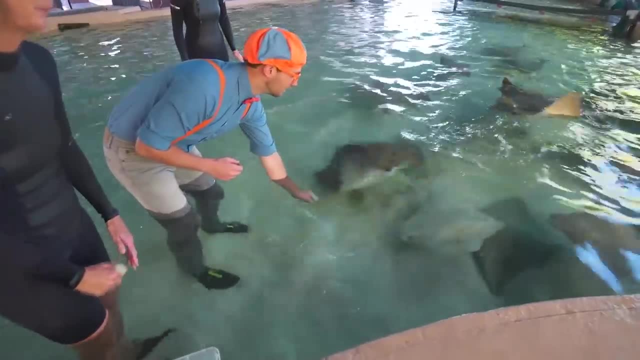 Okay, ooh, I like ice cream. Okay, just like that, Put it nice and deep into the water. They're gonna swim over your hand and they're gonna suck it out of your hand like a vacuum. Okay, Okay, here you go. 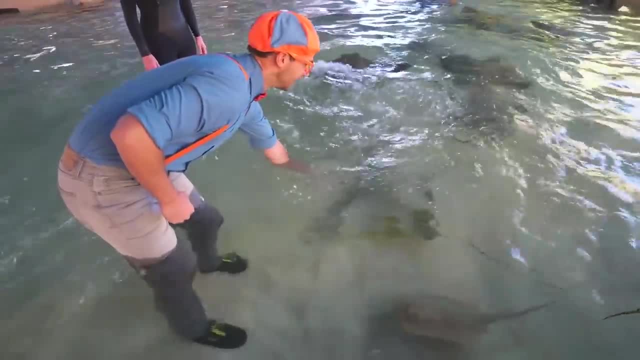 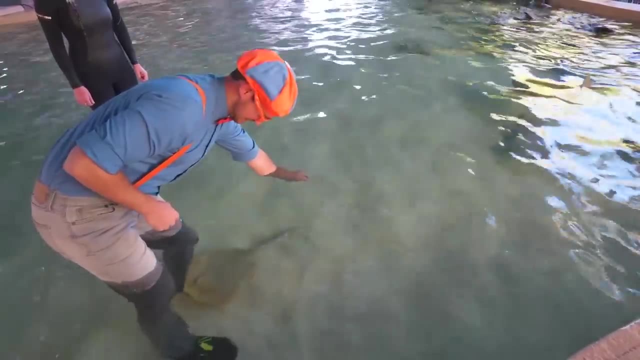 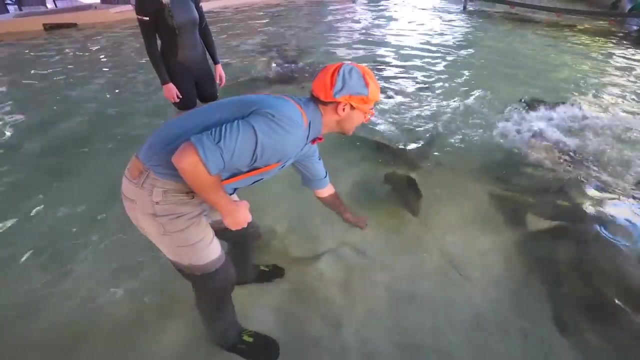 Whoa, whoa, whoa. look at that one. So you've got a blue-spotted ribbon tail sitting on your feet. Whoa, okay, do I go deeper in the water? Let's see what we can do. Come on, guys. 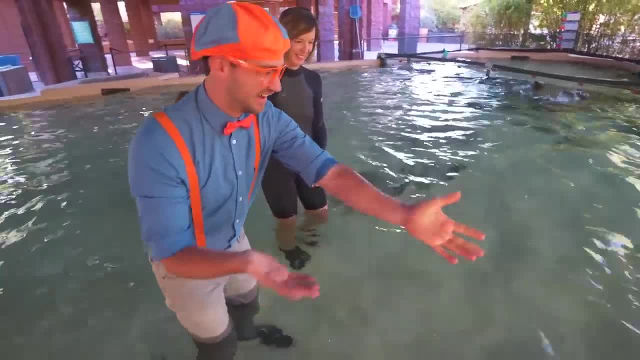 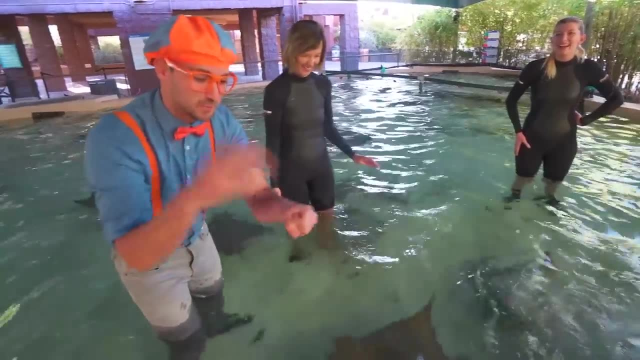 Oh, I did it. Look it's gone. It sucked it right out of my hand. Can I do it again? You can? yeah, Oh, thank you. They sucked the food right out of my hand. It's kind of like: have you ever put a vacuum on your hand? 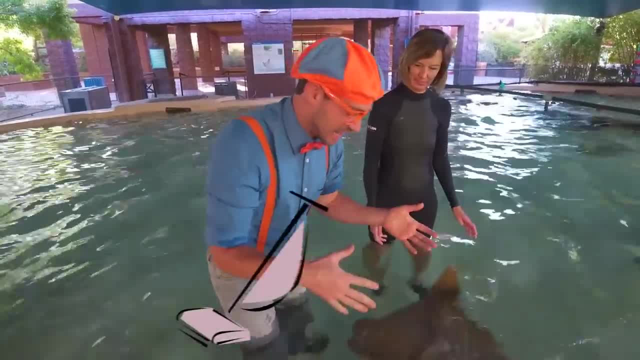 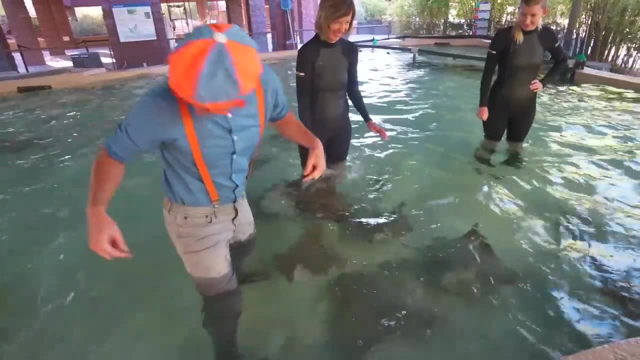 and then the vacuum sucks on your hand. That's kind of how it feels like when it's sucking the food out of your hand. Whoa, that one just swam through my legs. Whoa, look at them. So they're getting used to you now. 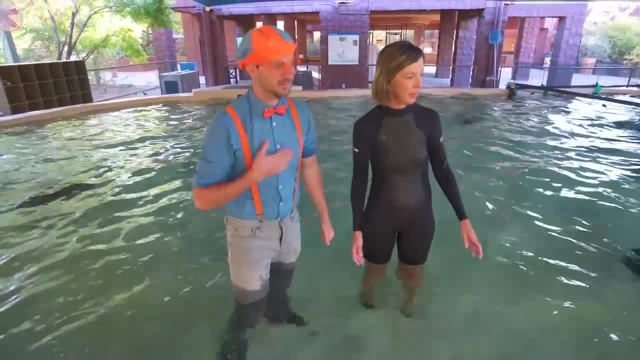 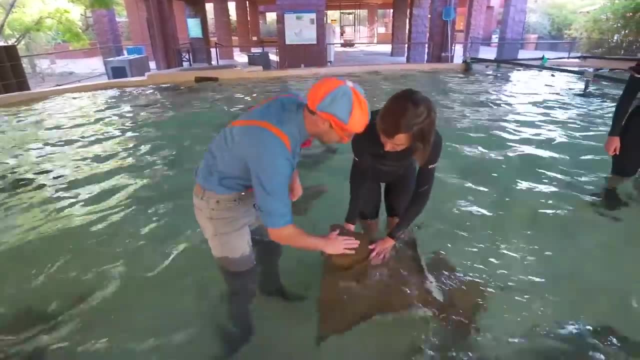 so they can feel who you are by your heartbeat. Okay, They're understanding that you're not going to hurt them, and so they're coming closer and closer as they're getting more and more comfortable with you. Yeah, look at them Hello. 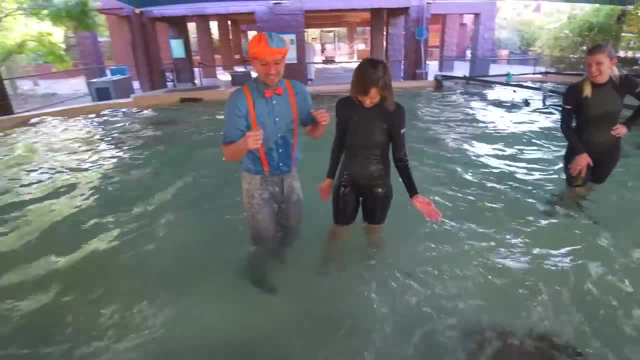 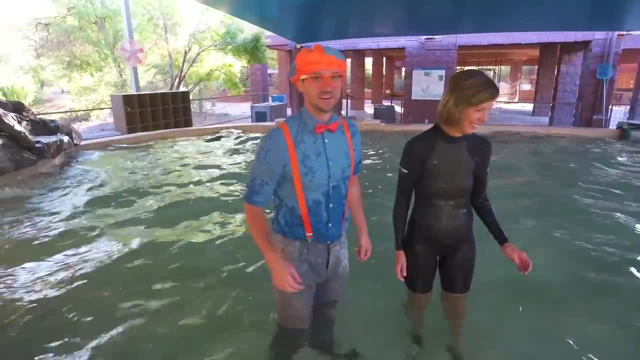 Whoa, Oh, my God, Oh, that scared me. What happened there? They just got a little bit excited. Okay, excited, not scared, Yeah, Okay, because I kind of got scared, But that's okay. They kind of seem really gentle. 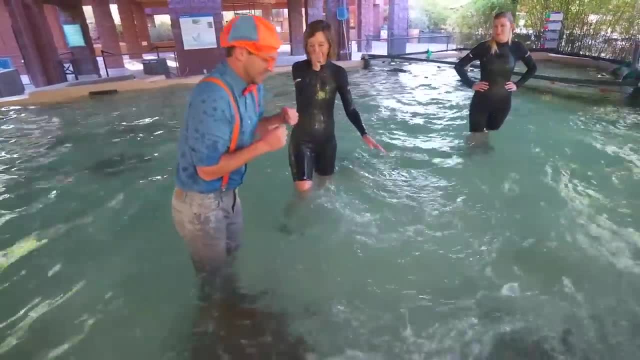 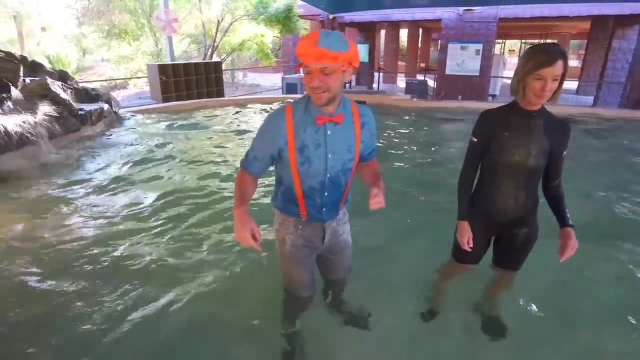 Oh, whoa, whoa, there they go again. Look at how wet I'm getting. All right, let's feed some more. Hello, look at all these stingrays. Whoa, All right, bye-bye, stingrays. 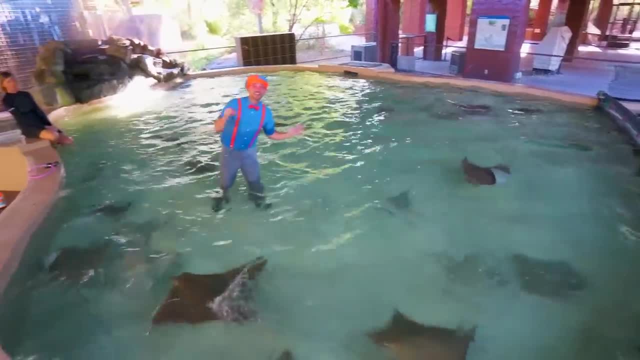 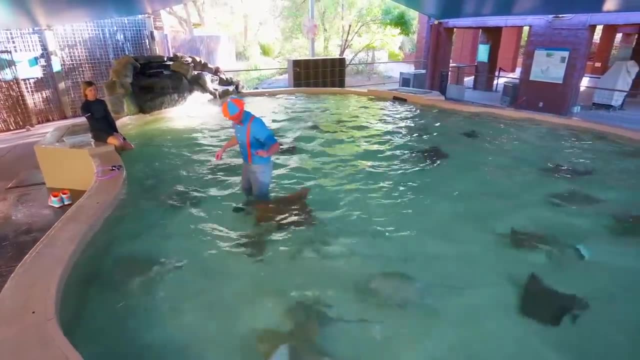 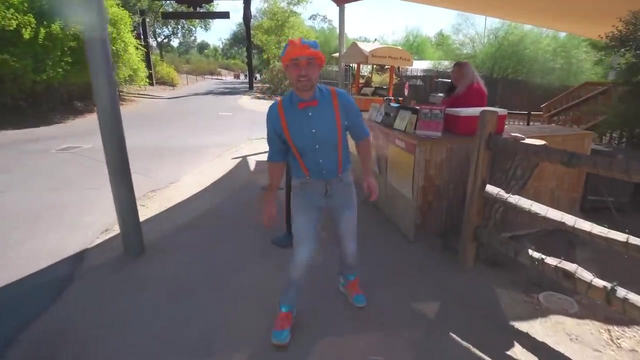 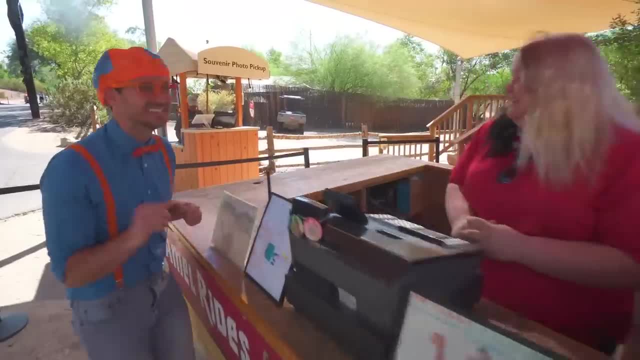 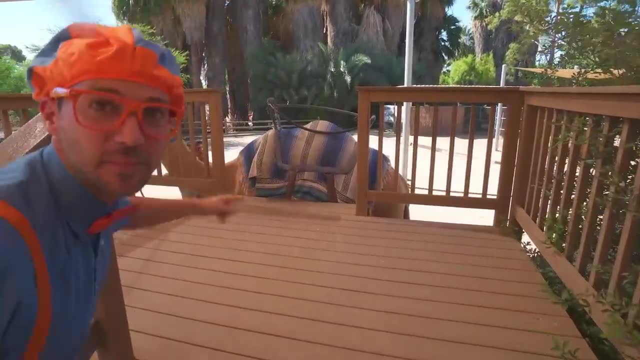 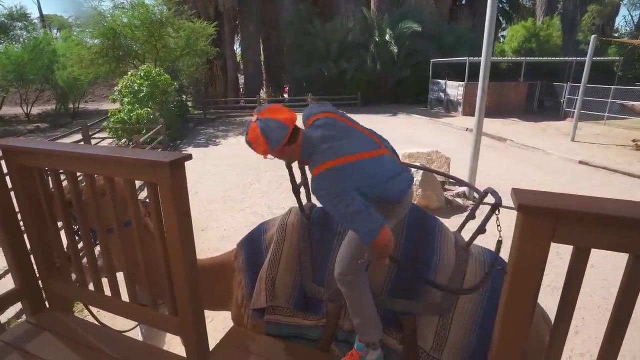 Bye, Bye, Bye, Bye, Bye, Bye, Bye. Whoa, look, This is the top of the camel. See the hump. I'm going to sit on top of it. Whoa, now I'm on top of a camel. 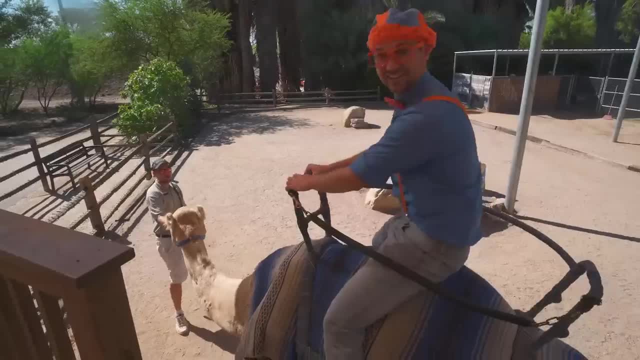 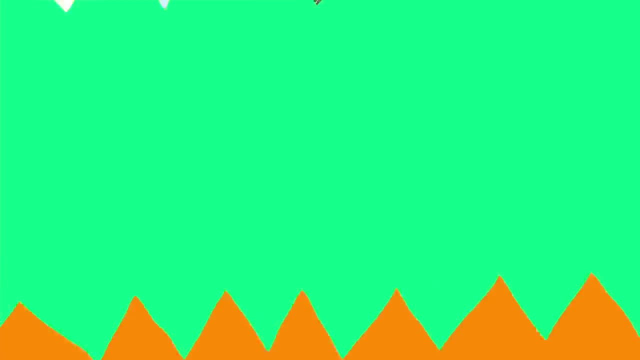 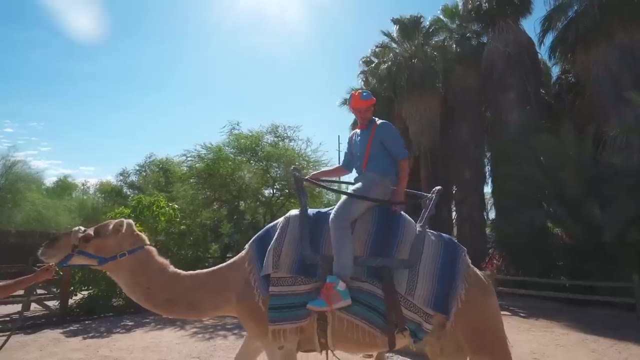 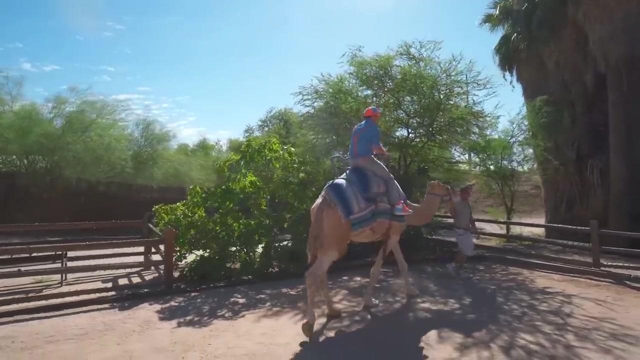 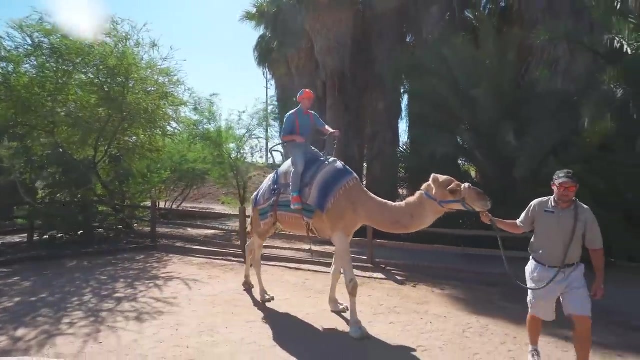 Okay, there we go, Check it out. Wee, Whoa. Hey Look, I'm on the hump of the camel. Whoa, This is a nice camel, This is a dromedary camel. It's really high up here. Whoa, I'm having so much fun. 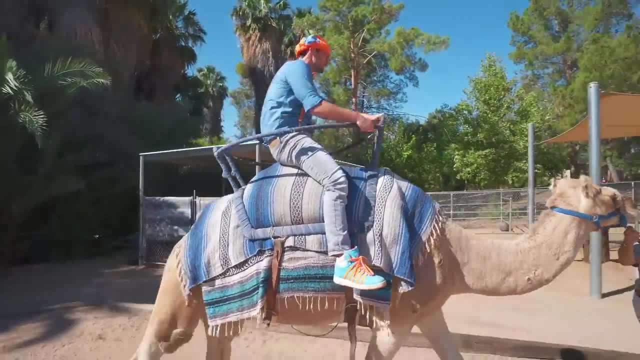 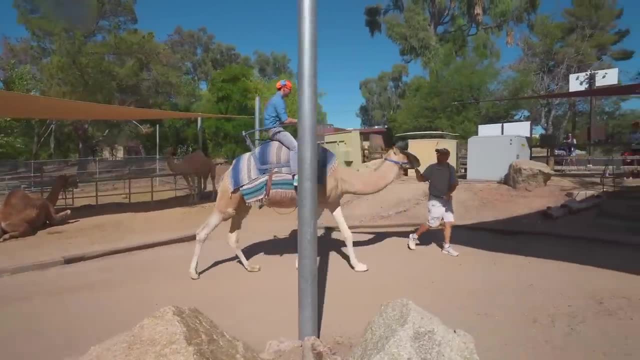 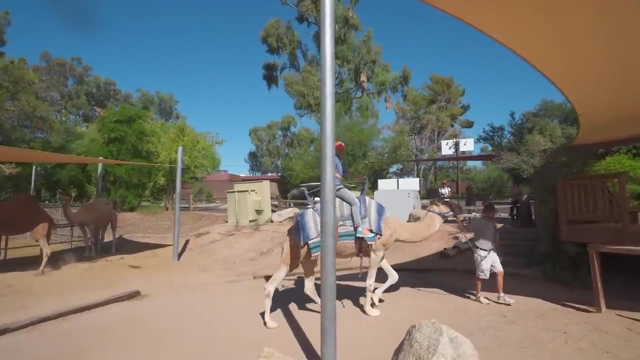 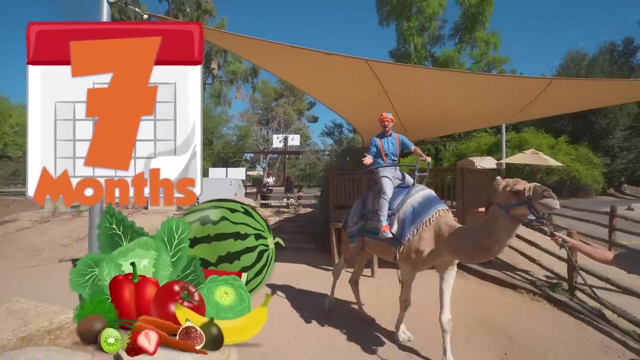 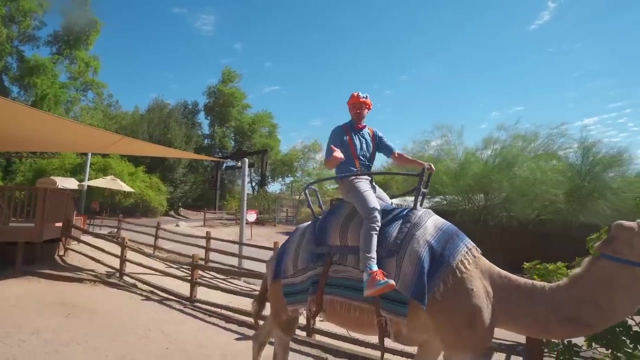 Ho-ho-wee, Hello Whoa, Check it out. See the hump of the camel. They store fat in here And they can actually go about seven months without eating food, Or three to four weeks without drinking any water. That's pretty impressive, huh. 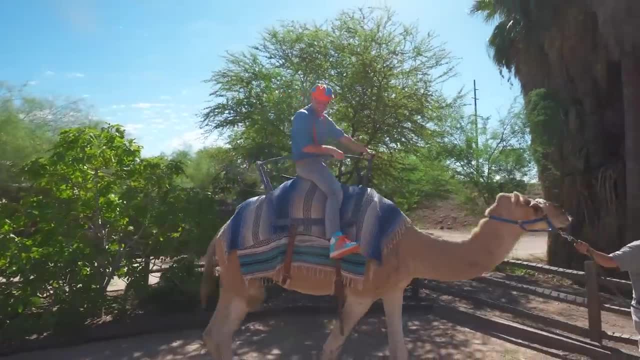 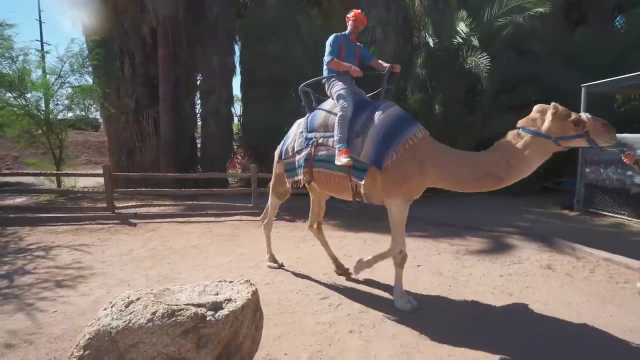 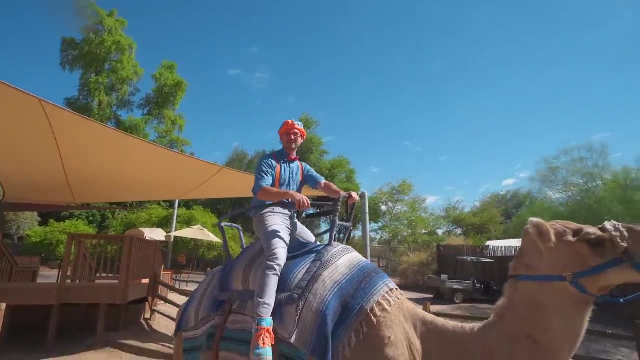 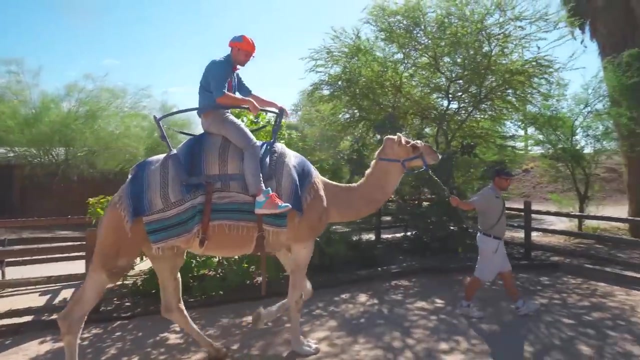 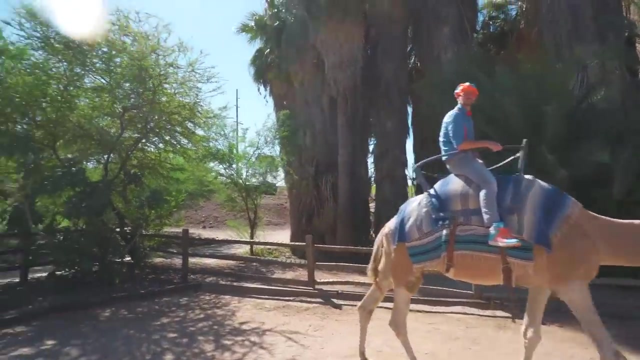 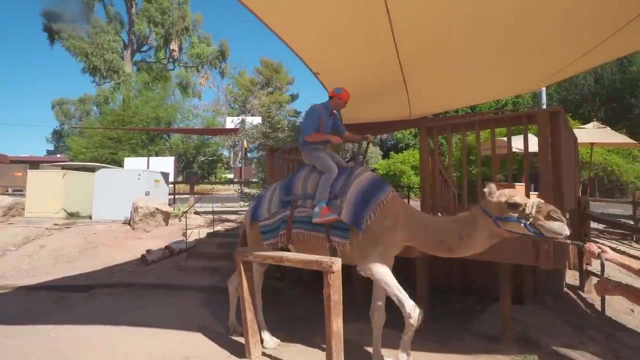 Whoa Whee, Whoa Whoa. It has some pretty long legs. huh, It has four legs And you and I have two. All right, This is pretty fun. Whoa, That was awesome. Thank you very much. 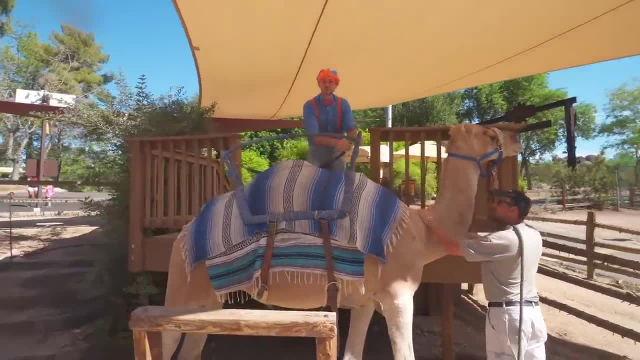 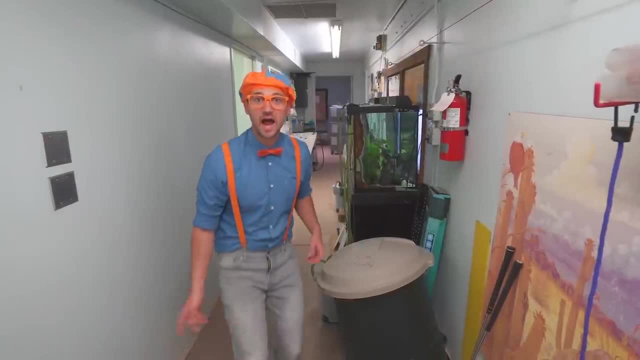 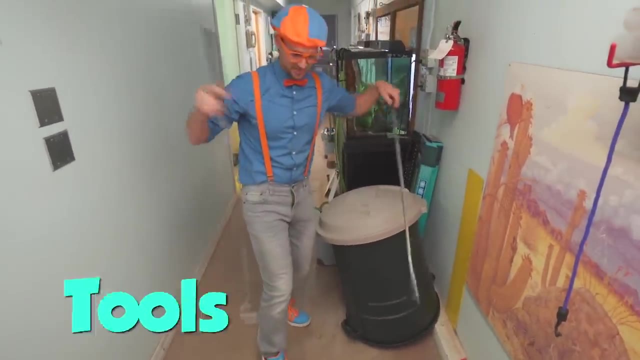 Yeah, you're welcome, All right. Okay, Let's go see some more animals. Whoa. Now we're behind the scenes of the Native Arizona exhibit. Whoa, Check it out. Look Some tools. Hey, What does this look like? 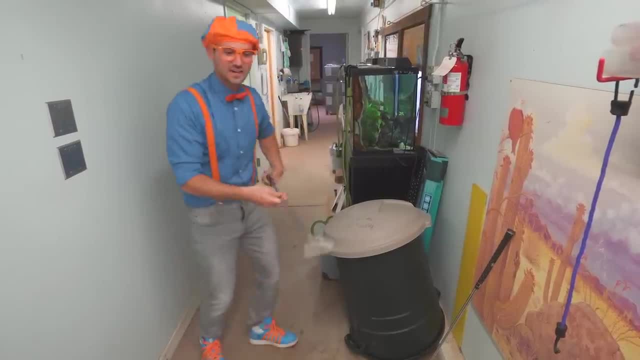 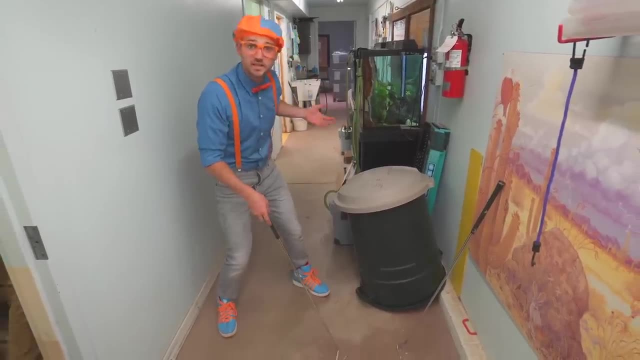 It kind of looks like a gun. It's a golf club, But actually see how it has a hook. It's used to handle certain types of reptiles like a snake. Okay, But I'm not going to use that because I'm not a trained professional. 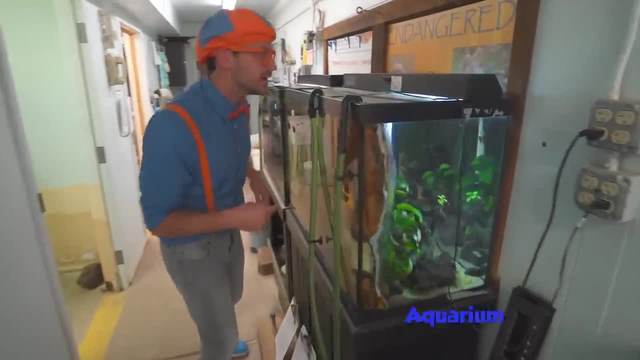 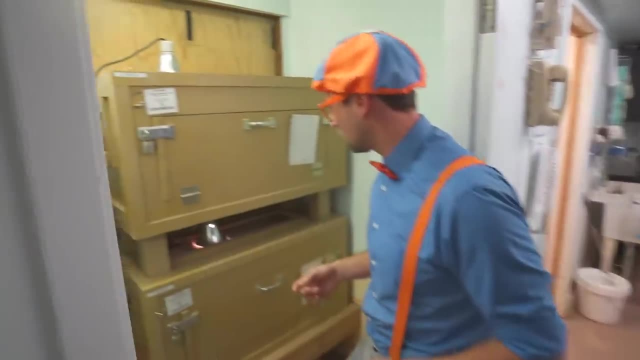 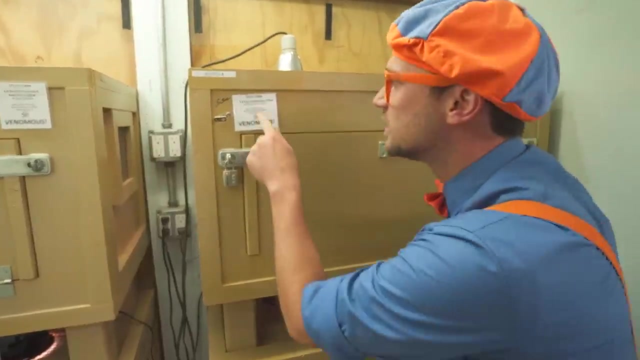 Whoa, Check it out. Wow, Some aquariums. The fish are on the other side. We're behind the scenes. Whoa, Look at this room. Whoa, This is a box And this is where snakes live- Snakes live. Let's read what kind it is. 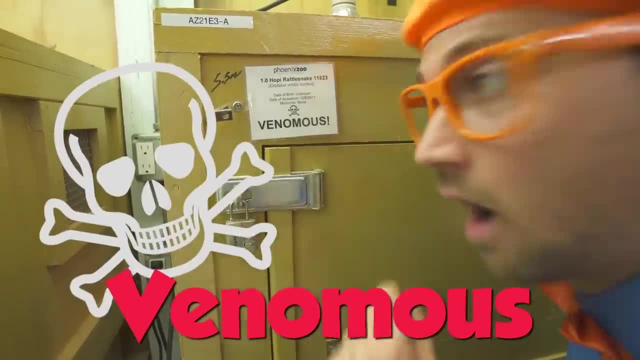 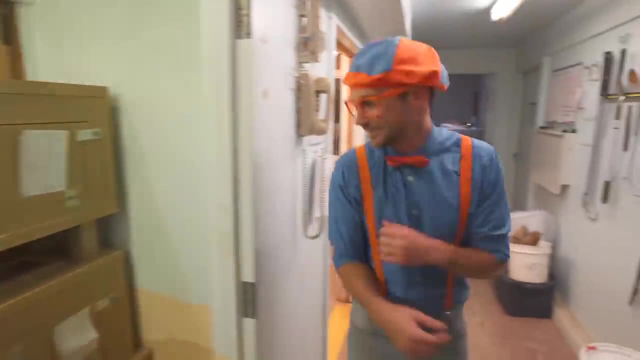 Rattlesnake: Venomous. Okay, I don't think I should handle that one because, like I said, I'm not a trained professional. Let's find a snake that I can handle. Whoa, This room's pretty cool. 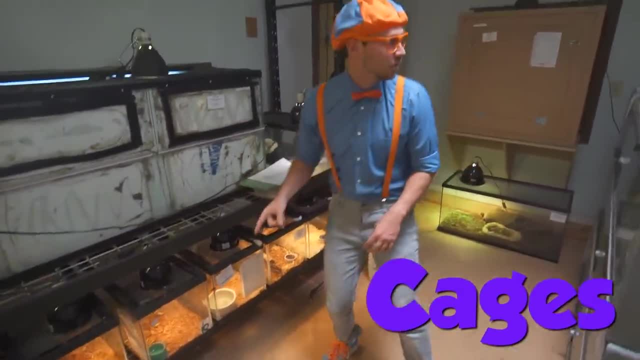 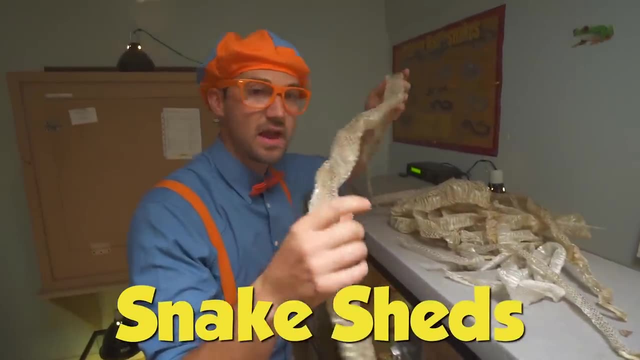 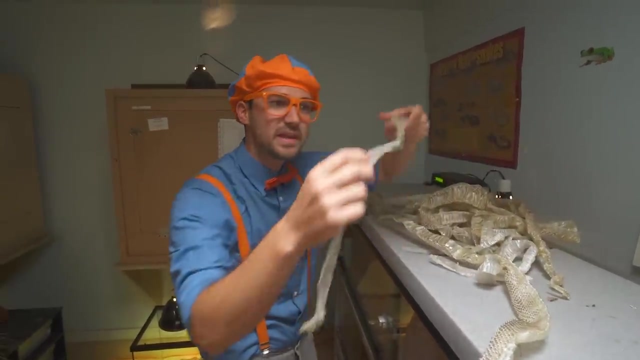 Whoa, There's so many cages right here. Whoa, What are these Snakes? These are snake sheds. Wow, Every snake sheds its skin every couple months. Look at that And they're all in one piece. Look, Doesn't that look like a snake? 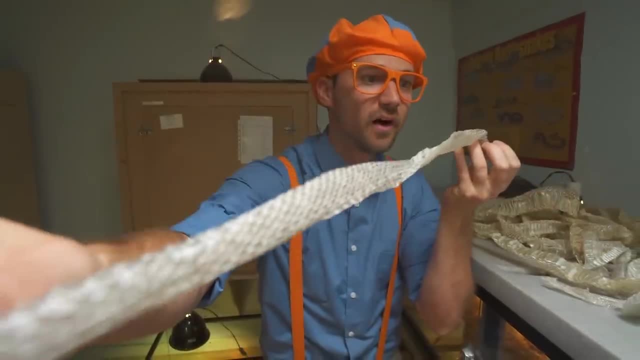 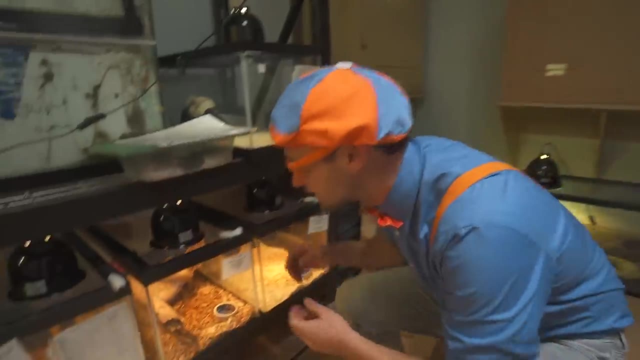 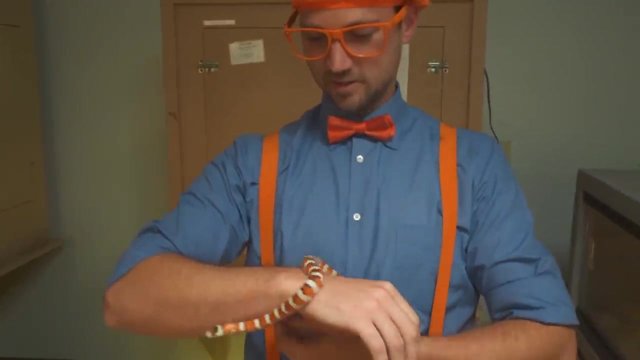 Yeah, That's pretty cool, huh, Okay, Okay, I'll keep these right here. Okay, Yeah, This one looks like a good snake to handle. I'm handling a snake- Whoa, And look at the color of this snake. 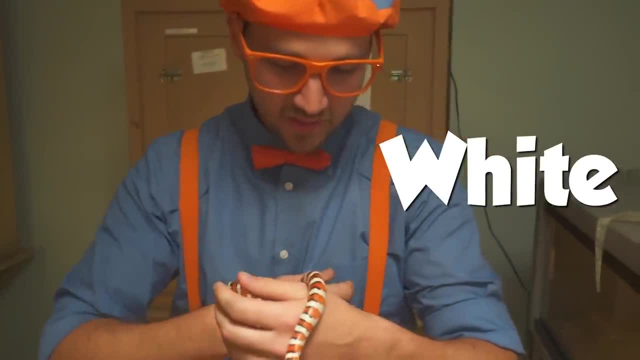 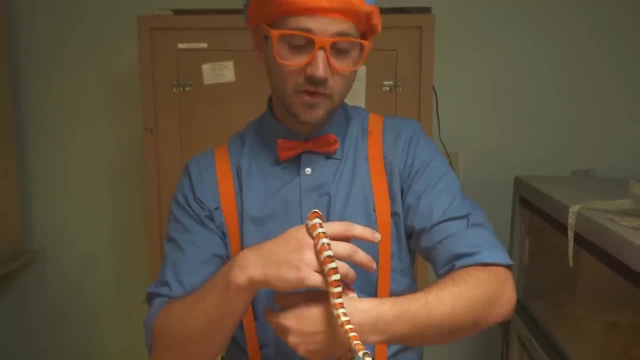 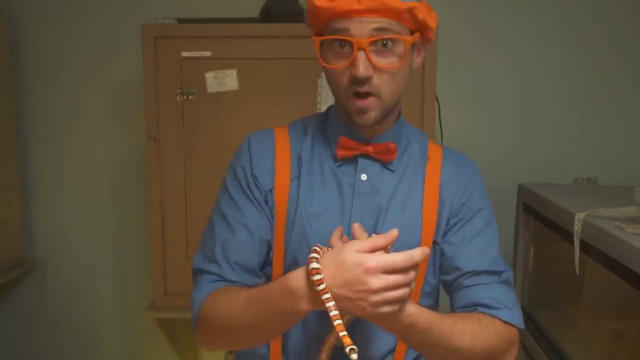 It's orange and white and black. Whoa, I used to be afraid of snakes when I was a child, but now I'm not. But some snakes you definitely don't want to hold. So if you ever see a snake in the wild, just to be safe, you probably shouldn't try and hold it like this. 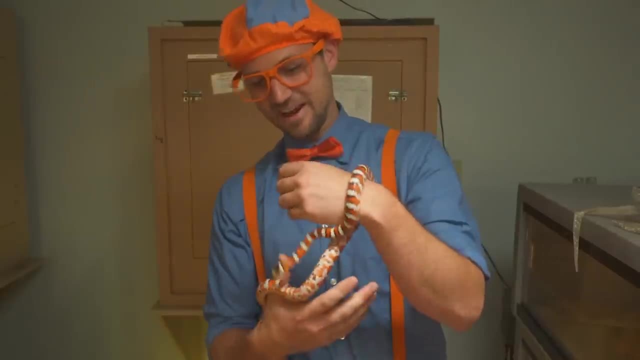 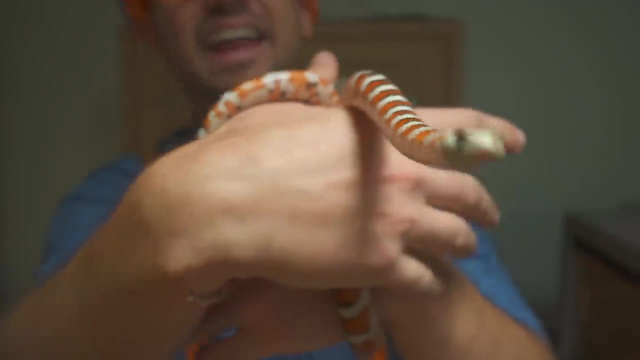 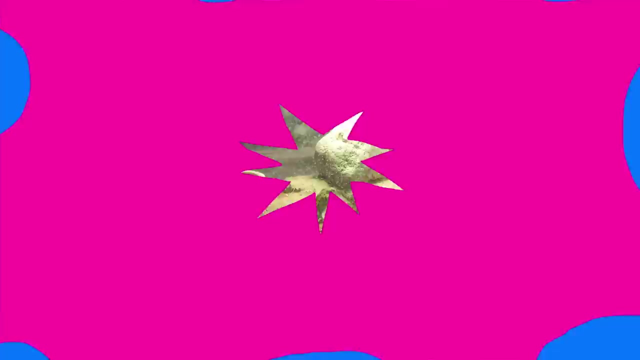 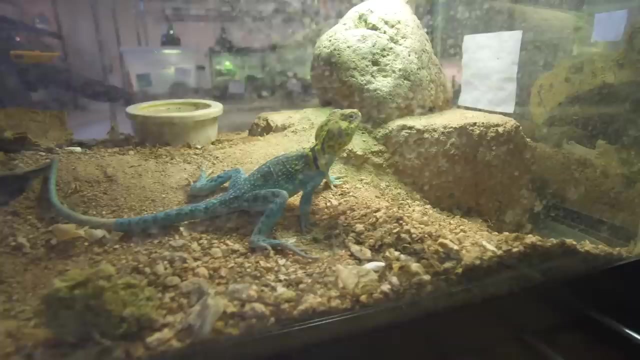 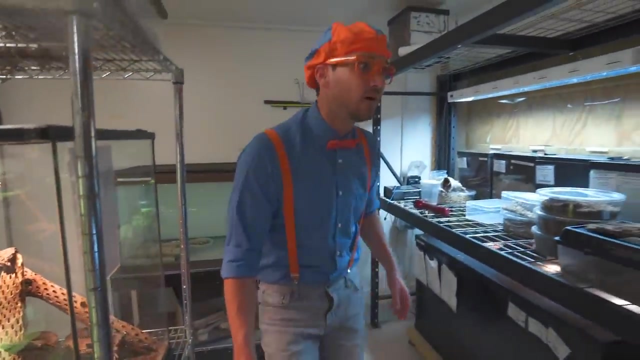 Okay, Whoa, Look, Are you having fun? snake Whee, Hello, Hey, Whoa, Look at it. Whoa, It's so intrigued with the camera. Whoa, Whoa. This is awesome, This is awesome. 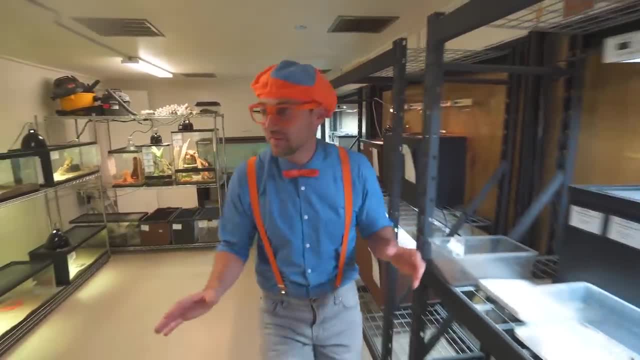 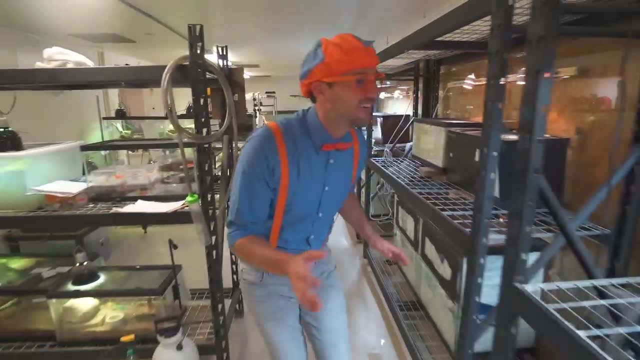 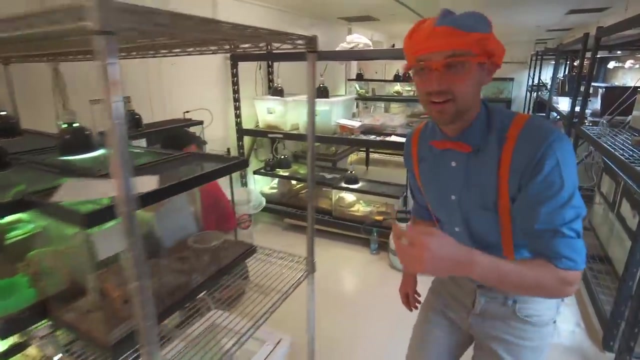 Whoa, This is awesome. This is awesome. Whoa, This is awesome. the scenes of another reptile area. whoa, there's so many cool tanks in here with so many unique creatures. oh hey, oh hey, there's someone over here. come here, whoa. 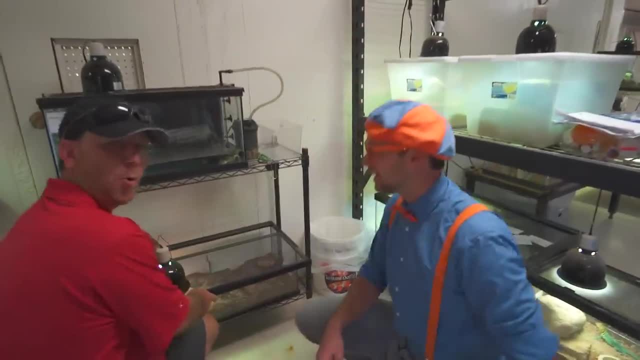 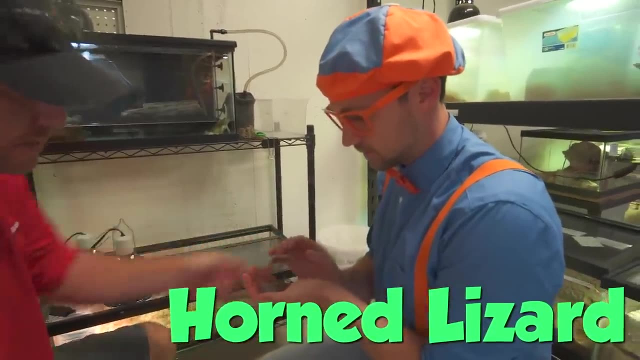 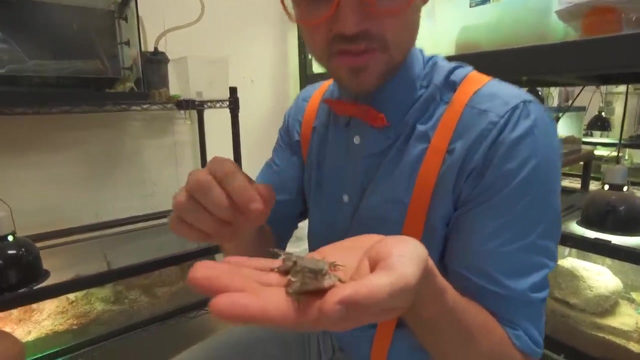 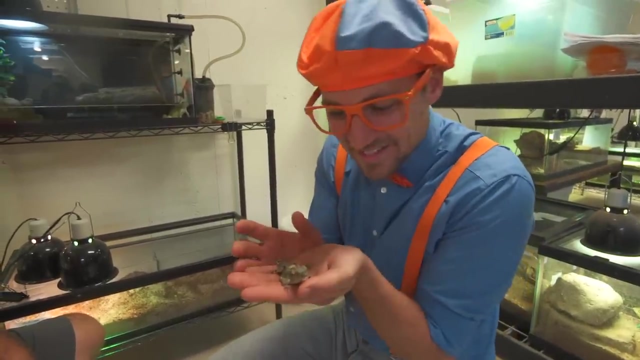 hey, what are you doing? just getting ready to check out one of our horn lizards. you want to hold them? yeah, a horned lizard, that's cool, okay, okay, thank you, whoa. look, this is a horned lizard. check out its horns. Wow, he's so cute. Oh, knees just hanging out. okay, well, thank you very much. 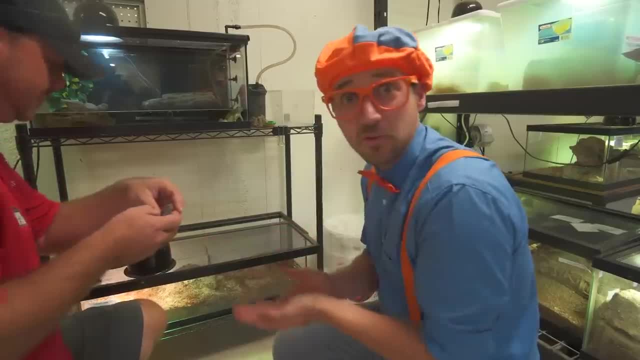 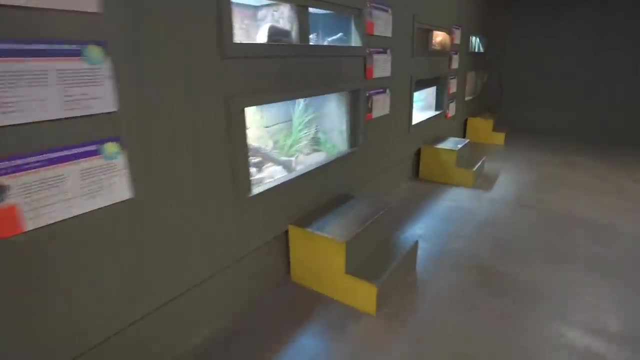 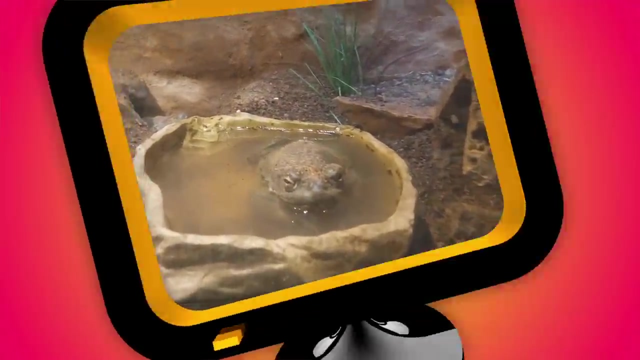 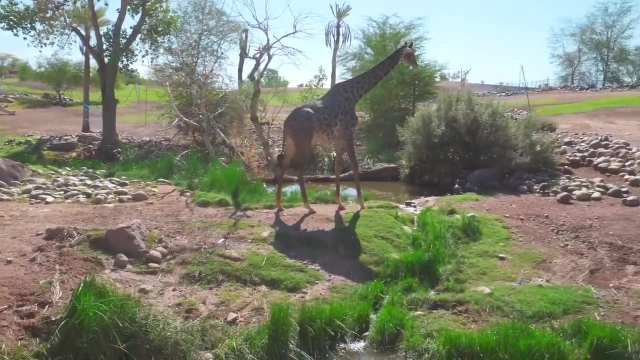 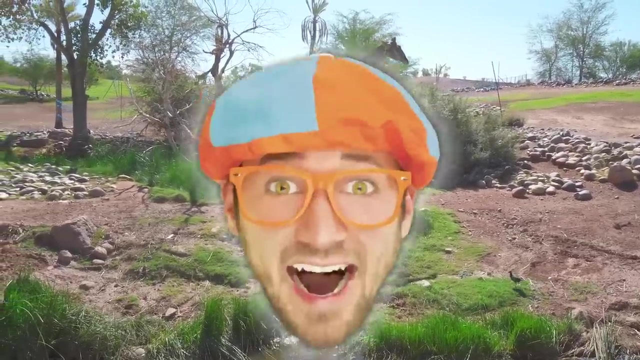 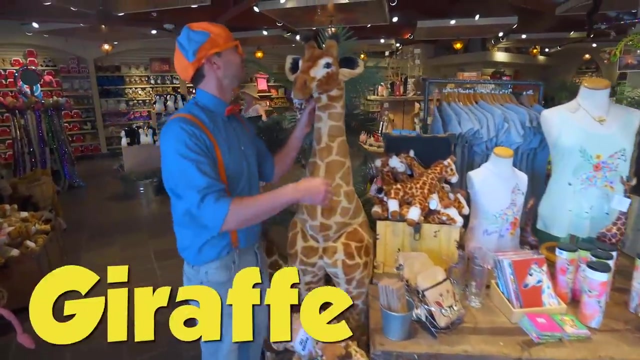 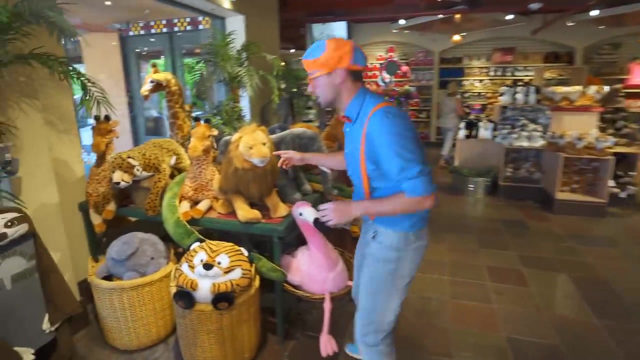 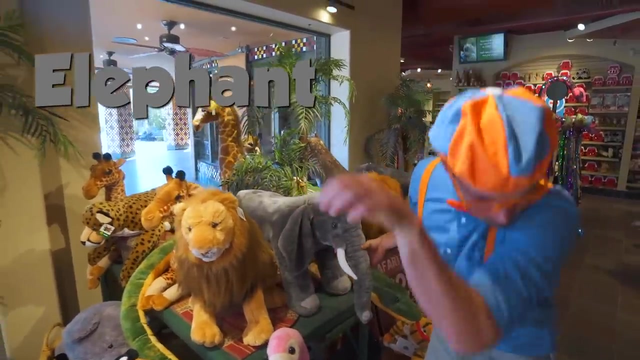 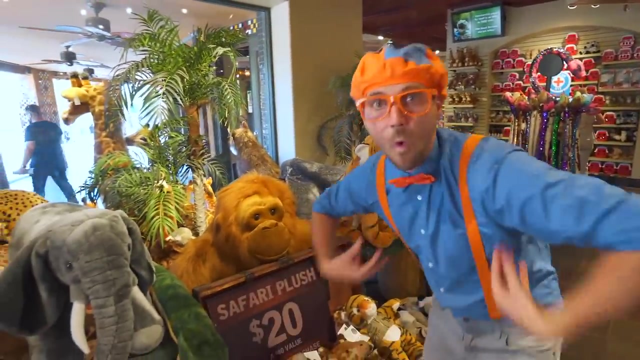 welcome. okay, there you go. that was awesome. good job, let's go. oh, Oh, a tall giraffe, Whoa, it's like my height. hello, hello a lion. whoo, an elephant, Roar Roar, Whoa, look, This is a gorilla, Roar Roar. 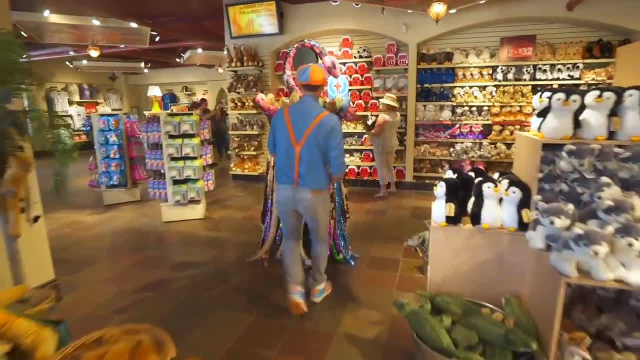 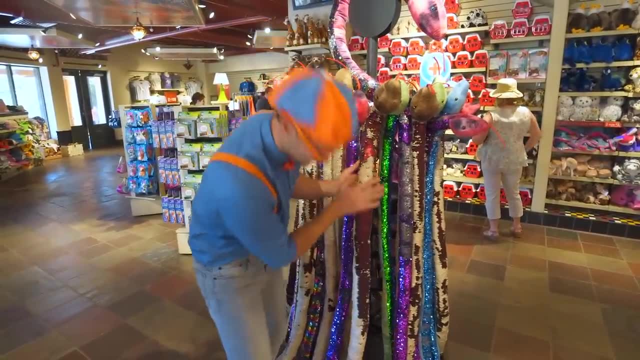 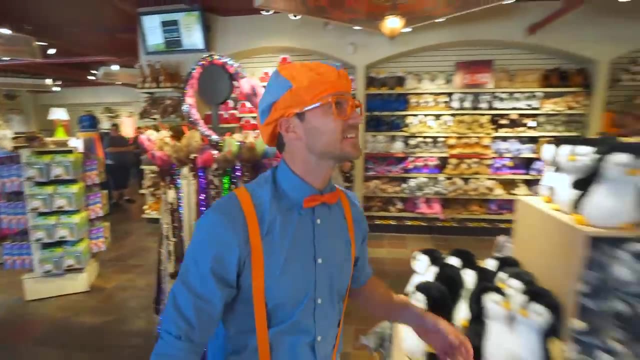 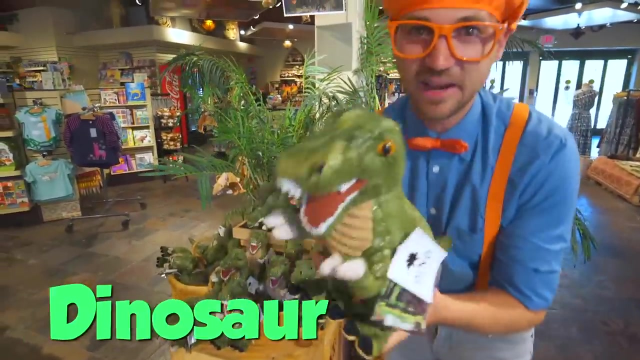 Roar, Roar, Whoa And some snakes. yeah, I gotta hold a snake. whoa, isn't that cool. Whoa, Whoa. There's so many cool things in here. okay, follow me. Whoa, There's even a dinosaur, a tyrannosaurus rex. interesting, well, hey, that was so much fun learning about animals with you at the zoo. this is the end of this video. 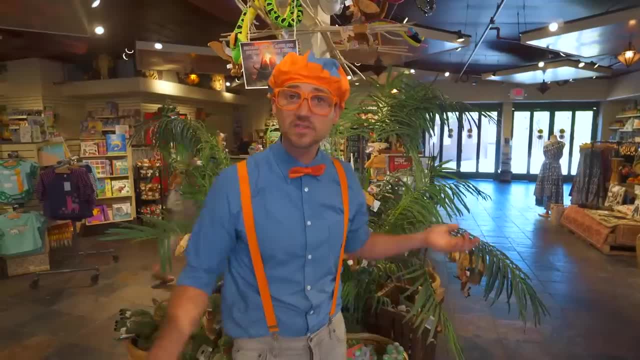 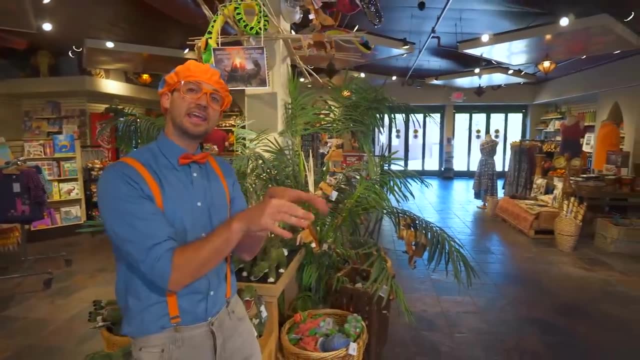 Well, hey, that was so much fun learning about animals with you at the zoo. This is the end of this video, but if you want to watch more of my videos, all you have to do is search for my name. Will you spell my name with me? 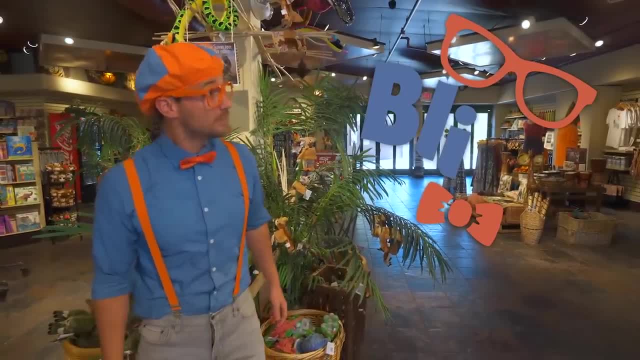 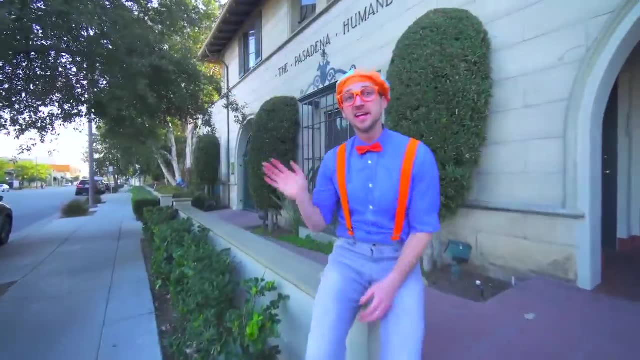 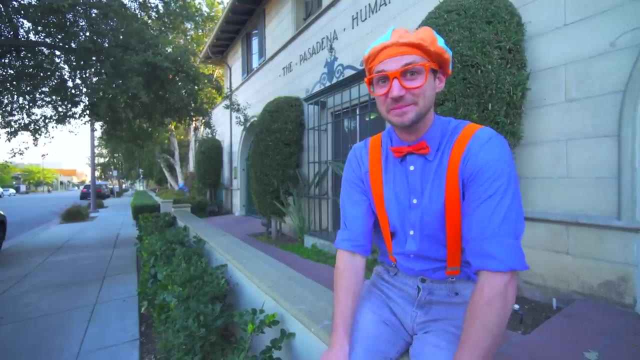 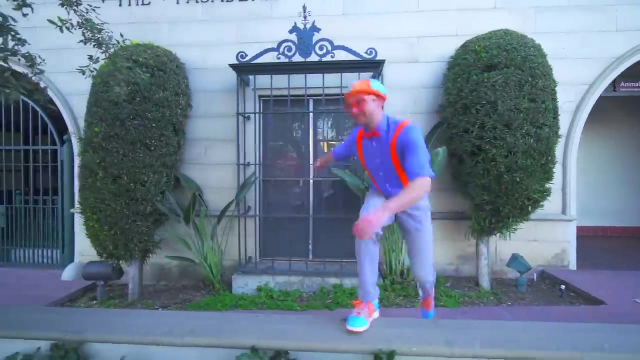 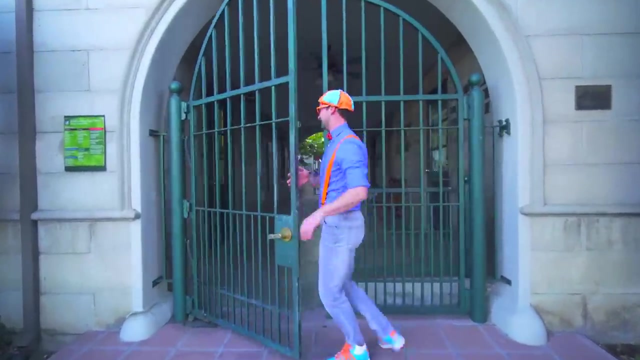 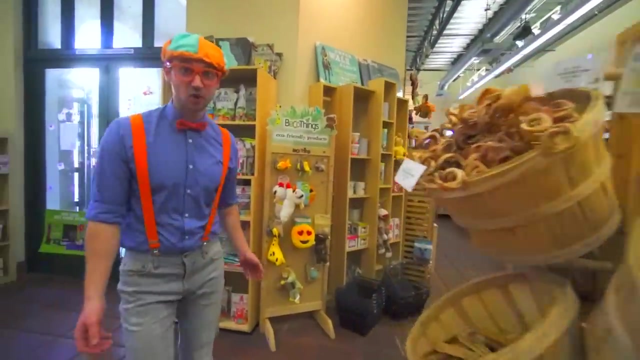 Ready B-L-I-P-P-I. Blippi, good job, alright, see you later. Hey, it's me Blippi, and today we're at the Pasadena Humane Society to see which animals need a home. I am so excited. come on. Okay, now we're in the shop where you can buy treats and toys and food and so many things for all the pets here. 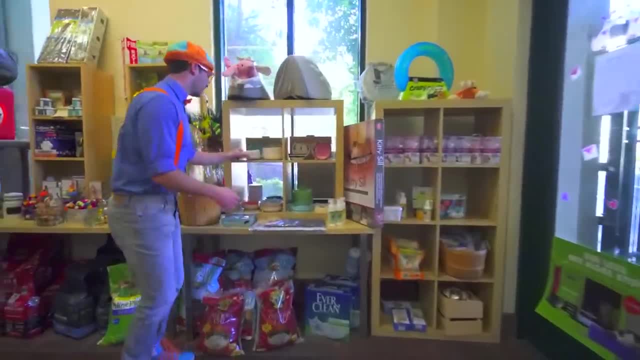 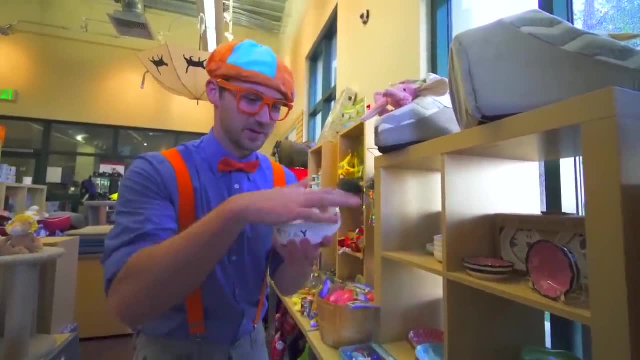 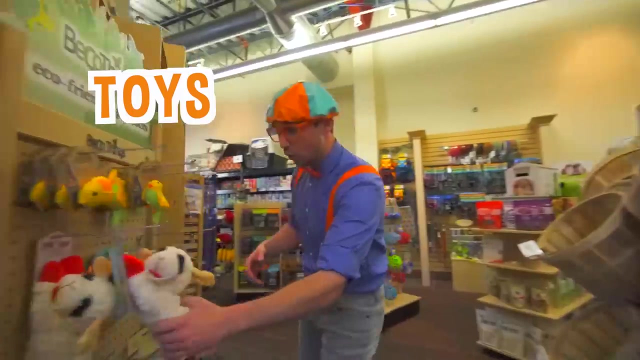 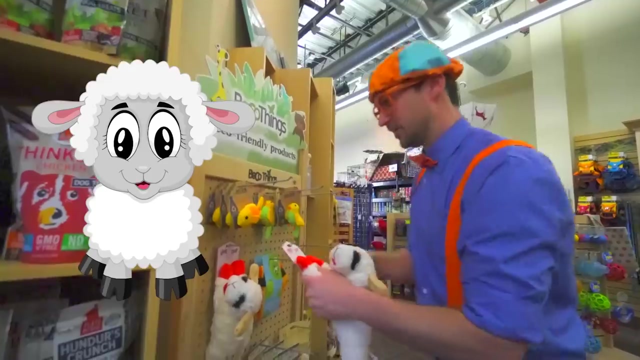 Hey, what do they have? Ooh, look, Hahaha, Every day is Catter Day. That's funny. this is where the cats eat their food. Oh, look over here, Some toys. Whoa, This is called Lamb Chop, Ooh, and it looks like a little fish. 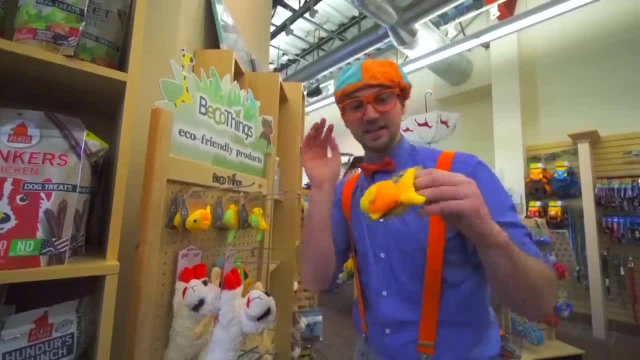 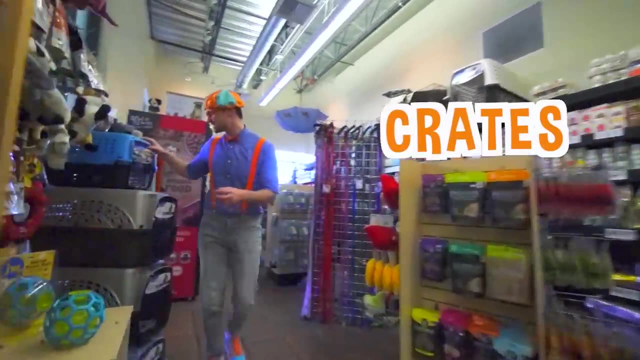 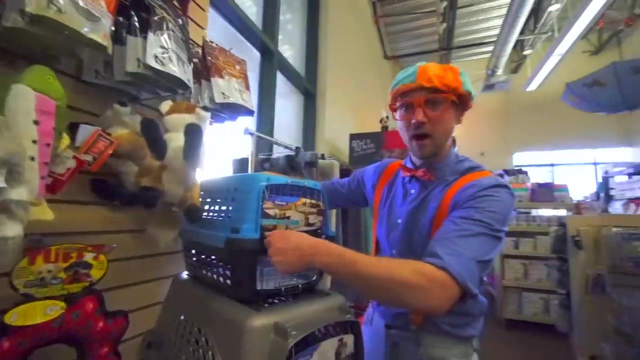 I bet this is for a kitty to play with, because kitties love to play with fish. Ooh, Some crates. Look, If you need to transport your pet from the Humane Society, you will probably take it inside a crate like this See. 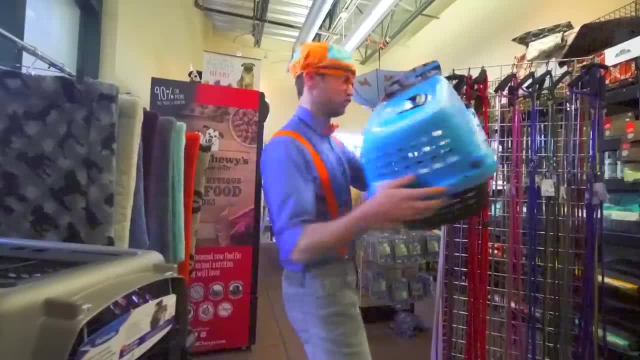 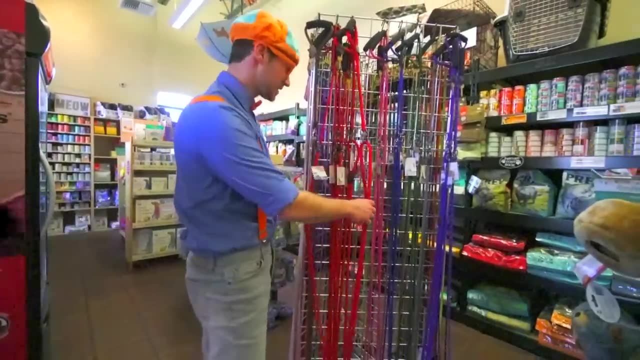 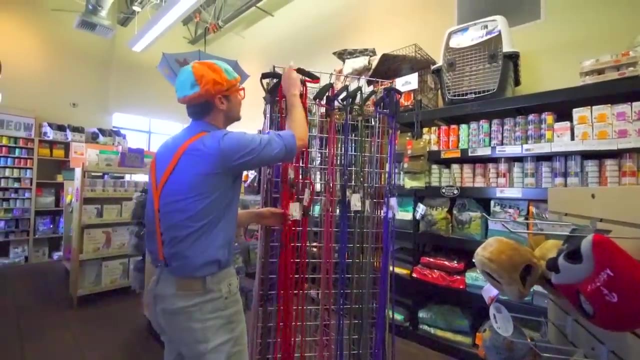 So then they're nice and safe when they travel. Mmm, Ooh, And leashes, Wow, Look at all these colorful leashes. This leash is the color red. Hmm, Hmm, Ooh, This leash is the color pink. 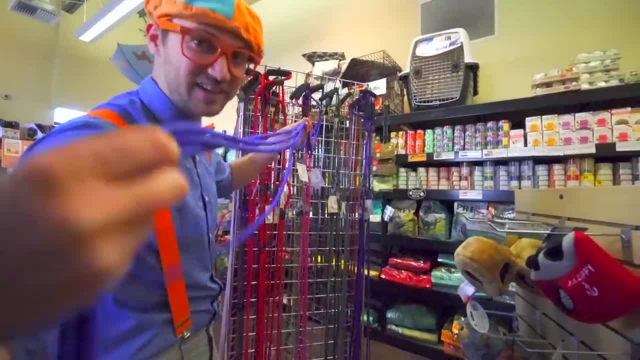 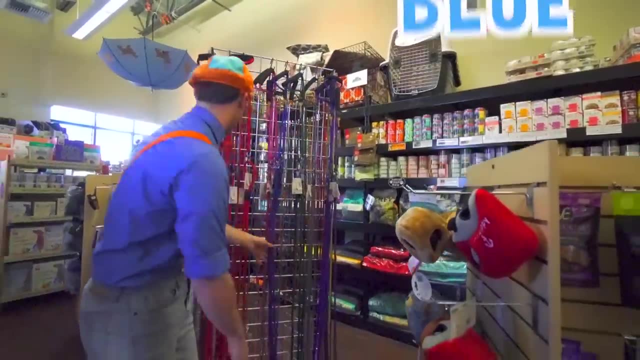 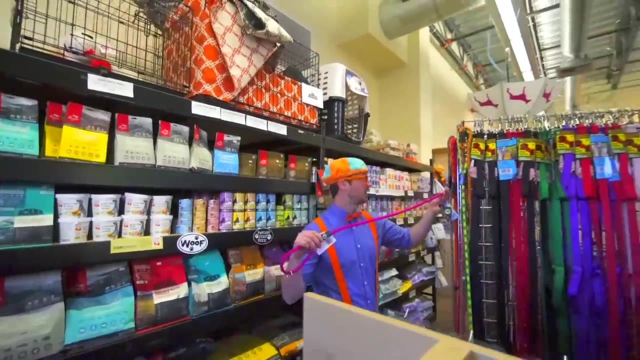 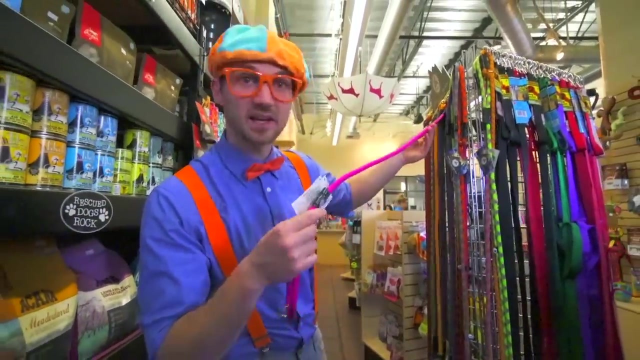 Ooh, I bet you know this color. I wear this color all the time. Yeah, It's the color blue. Ooh, Come on this side. Wow, Look at this color. Yeah, It's so bright and vibrant. This color is the color pink. 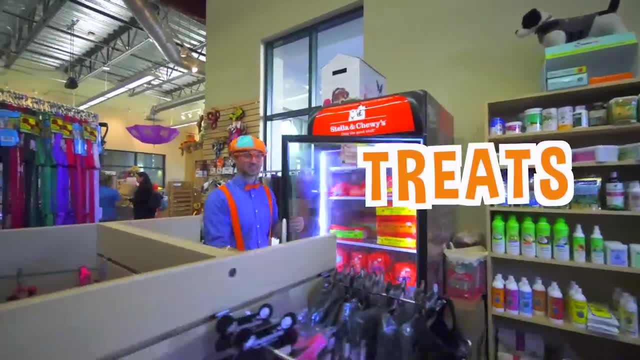 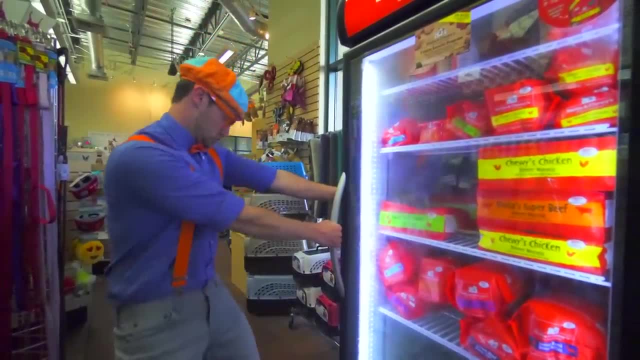 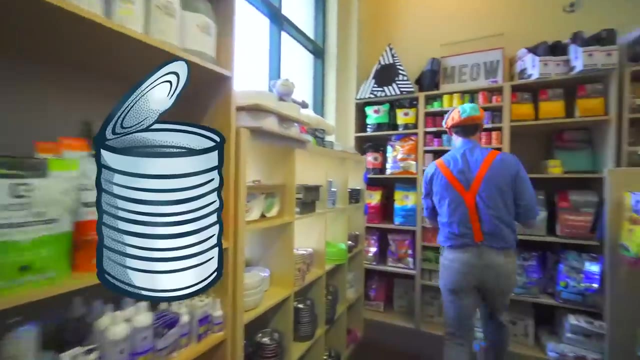 Ooh Yum, Some more treats. But wait a second. This looks like it's for. I can't open it anymore. Hey, Canned food, Come here. Ooh, Some cat food. Ooh, More bowls. 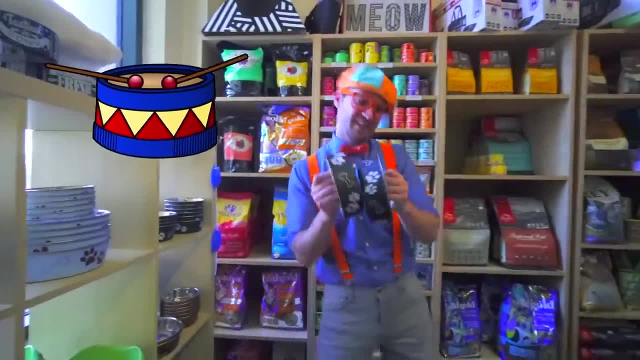 These look like dog bowls. Come over here If you have a dog, or maybe even a cat. you've probably seen these bags. Yeah, They have a lot of food in them, And I think this is for chickens, Or maybe it just has a chicken flavor in it. 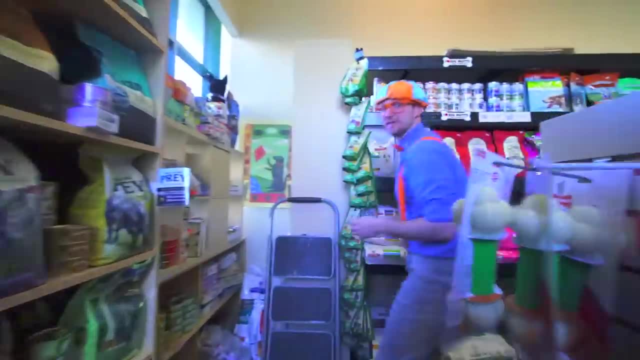 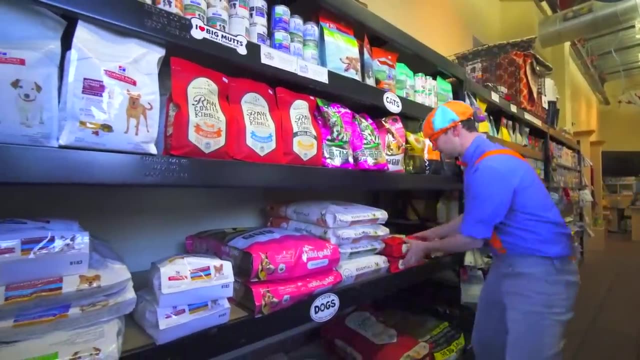 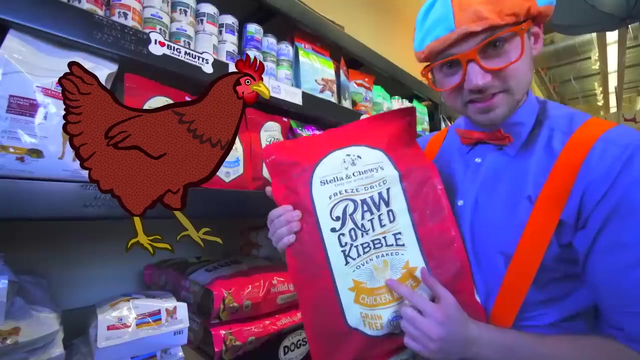 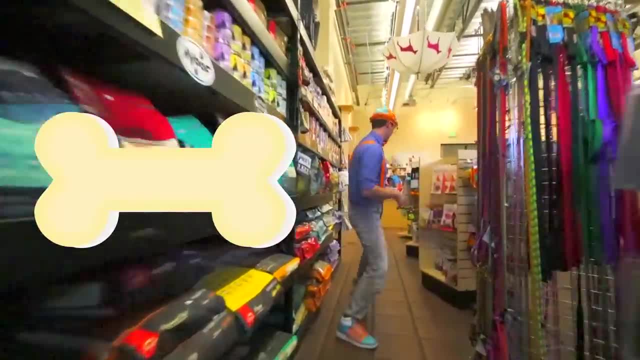 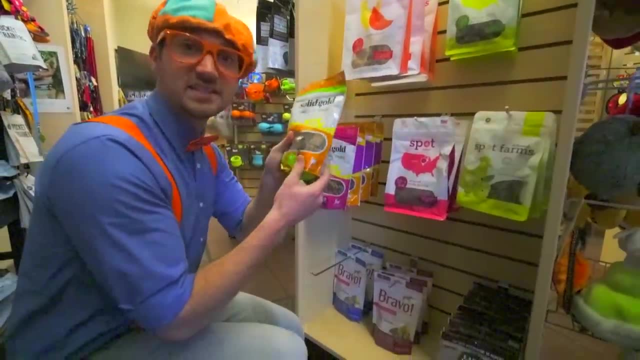 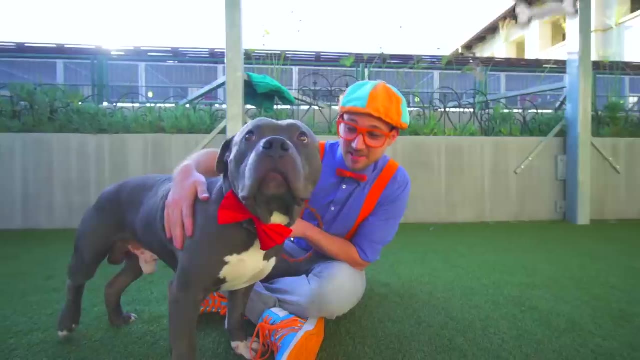 Oh, And treats. Yeah, Look at this. These are treats, and dogs love these. Maybe we can get these and go feed them to a doggy. Come on, Oh, do you see this dog? This dog's name is Timmy. 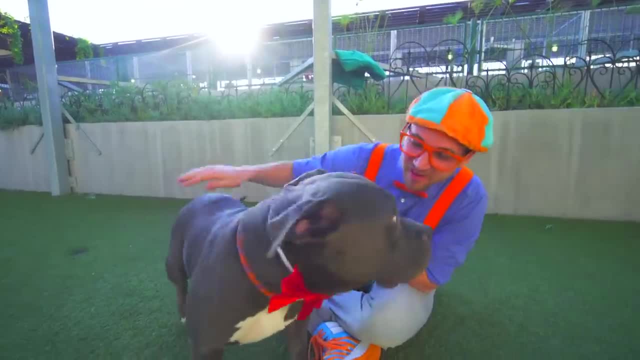 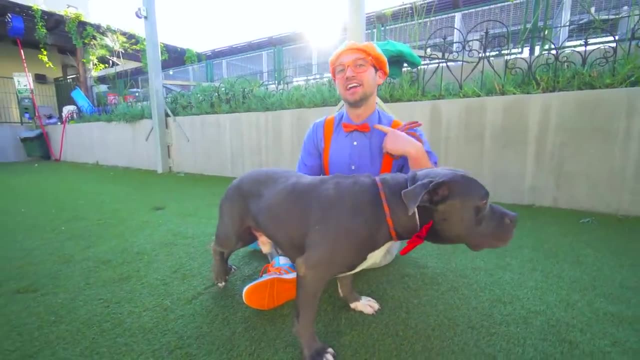 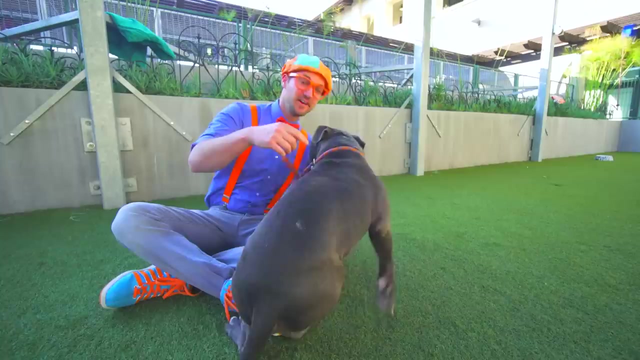 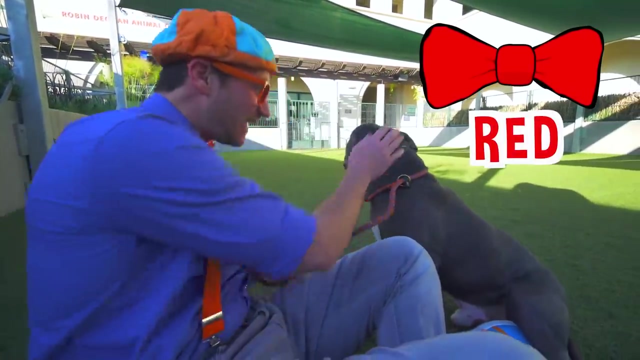 Ha, ha. Oh, And do you see, right here He has a bow tie on a bow tie on, Just like how I have a bow tie. But my bow tie is the color orange And Timmy's bow tie- do you see the color? Whoa, hey, Timmy, Timmy's bow tie is the color red. Wow, that's. 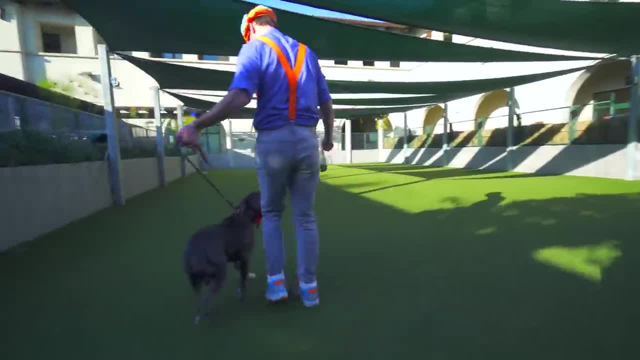 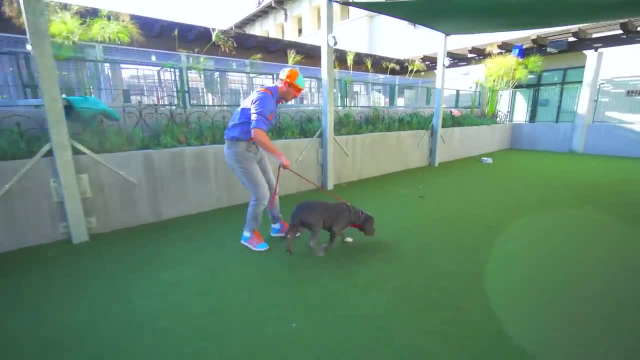 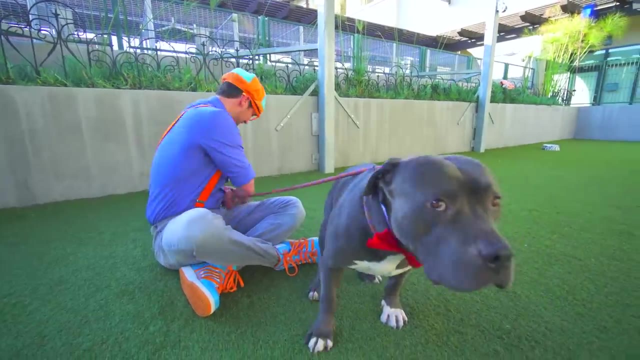 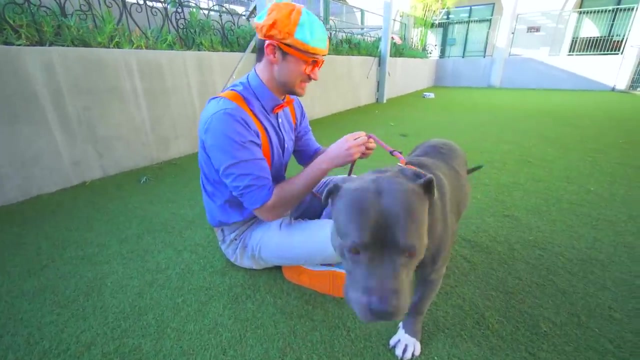 a really cool bow tie, Timmy. Hey, remember the treats we got earlier? Yeah, Timmy loves them. Hey, Timmy, look at what I have for you: A treat. Yum, Timmy loves these treats. This is equivalent to like our. 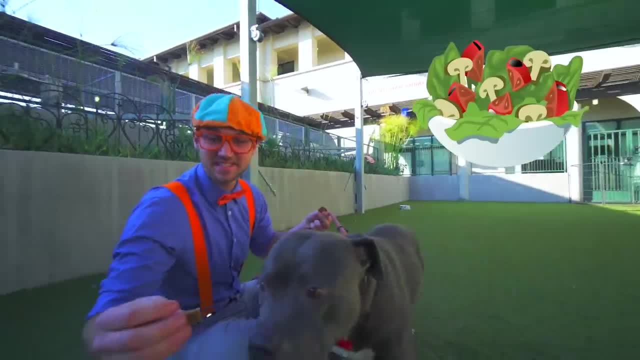 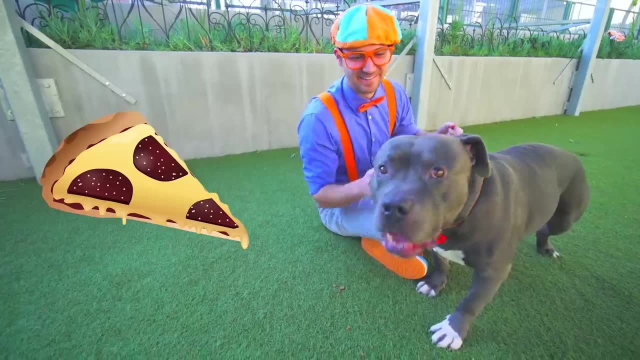 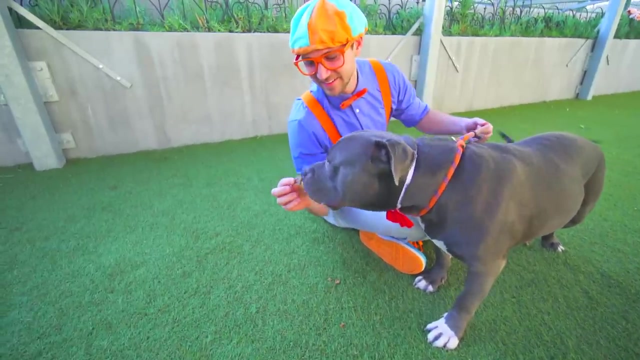 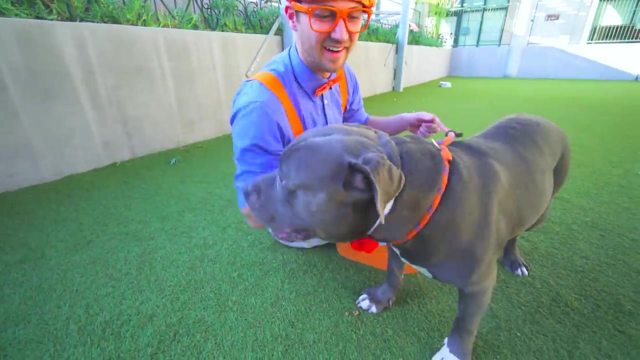 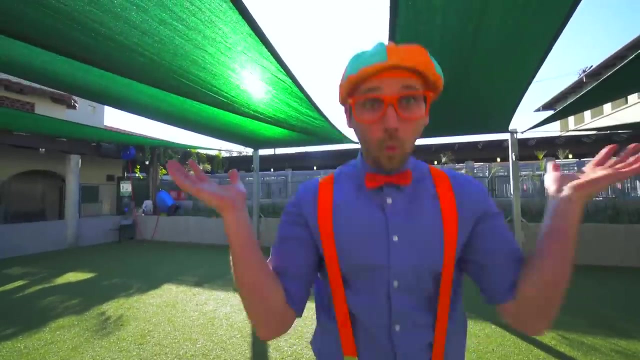 um, a nice tasty salad, Or even maybe like a piece of pizza. Yum, Good boy, Timmy. Okay, last one, Here you go. Ooh, okay, now let's play with Pierre and Panther. There they are. 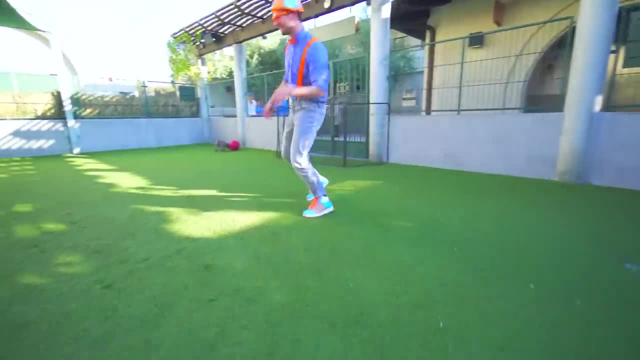 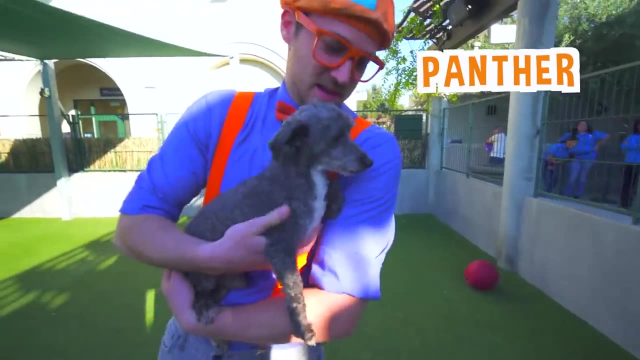 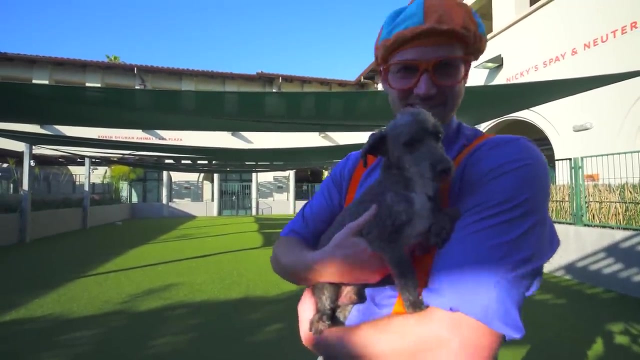 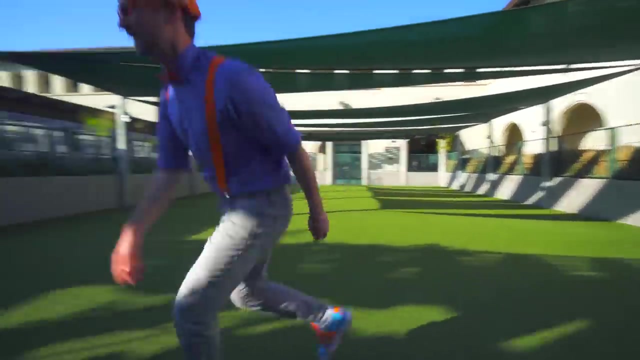 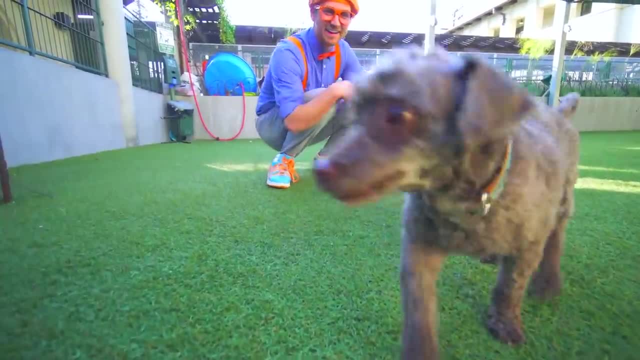 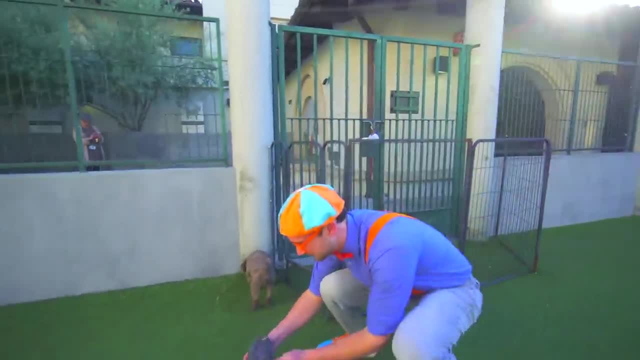 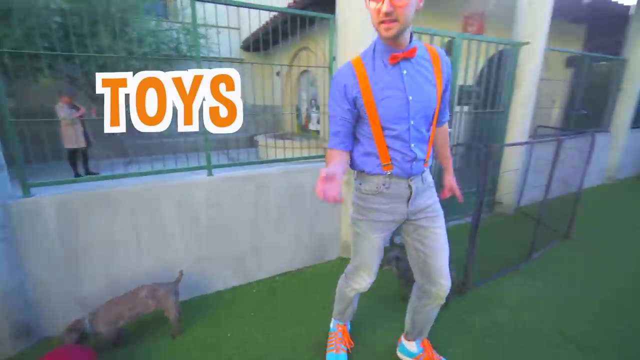 Oh, I wonder if they're siblings. I don't know, But they look so similar. Hey, Oh, there's some toys over here, Let's go get some. Oh, let's see if they like these. Stay, stay on my 뻔șo. 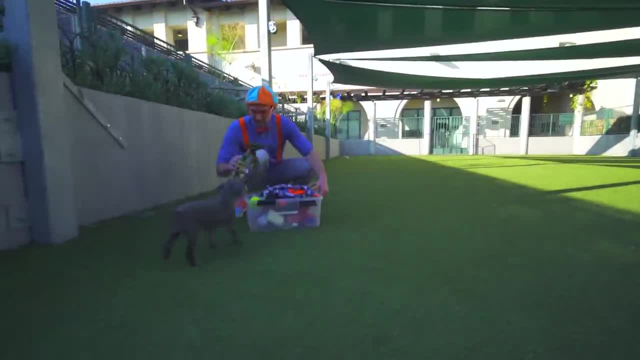 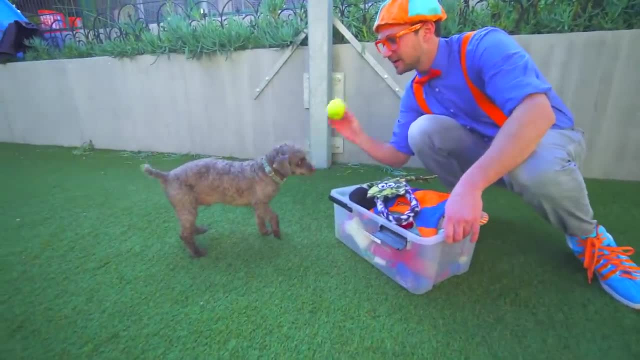 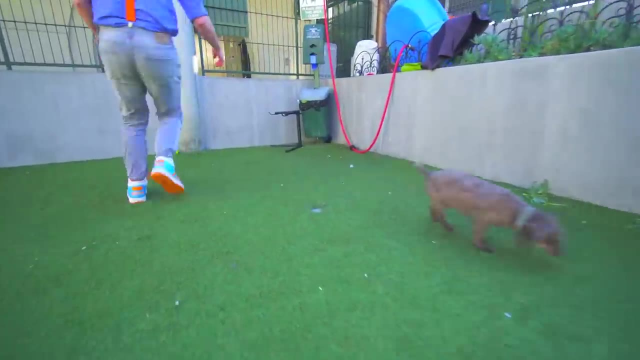 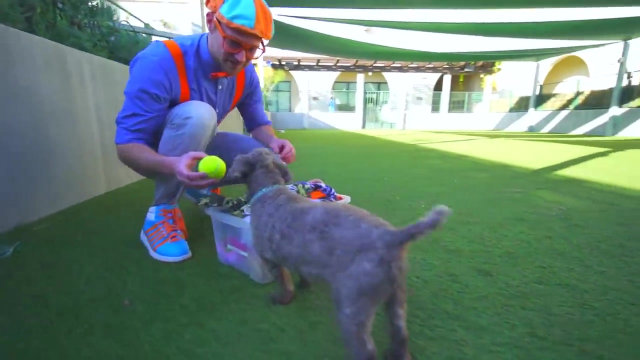 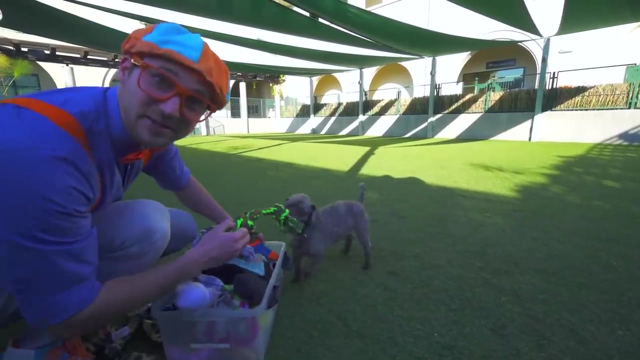 Hey, Haha, Okay, You want a toy. Oh, I guess not. Hey, you want a toy. You want a tennis ball Ready? Okay, here we go. What about? what about this toy? They are so cute. 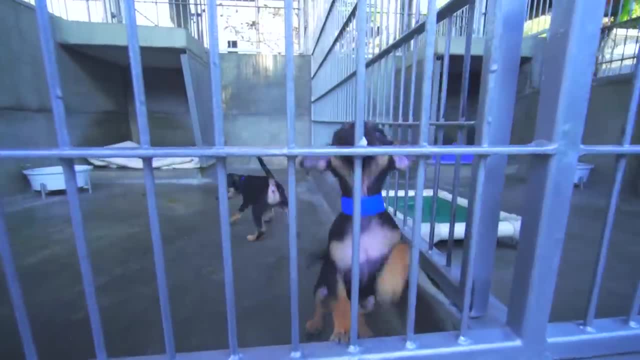 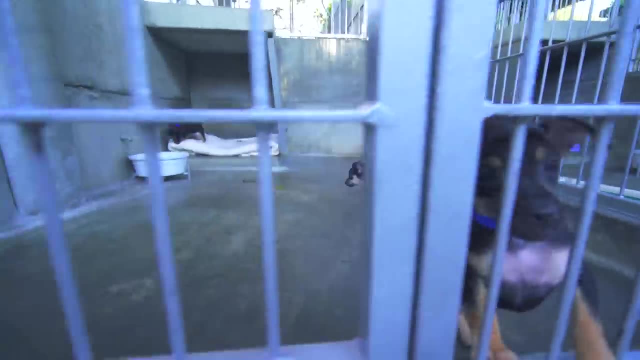 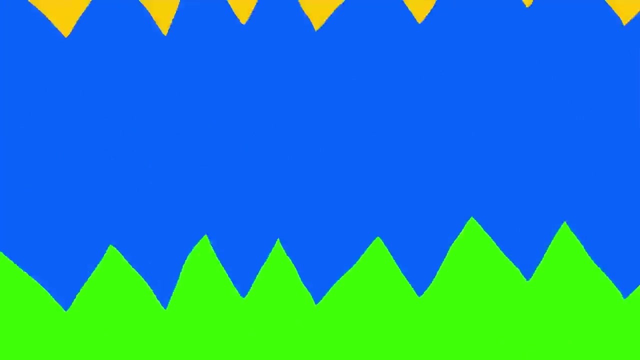 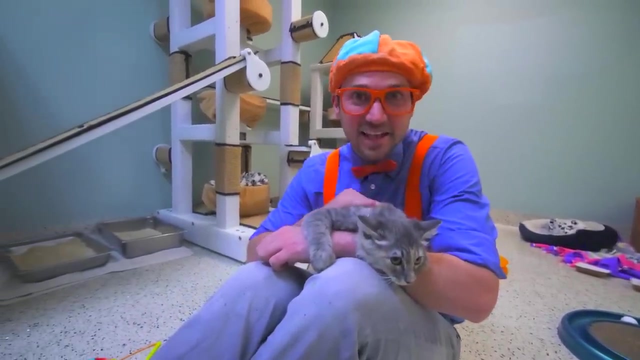 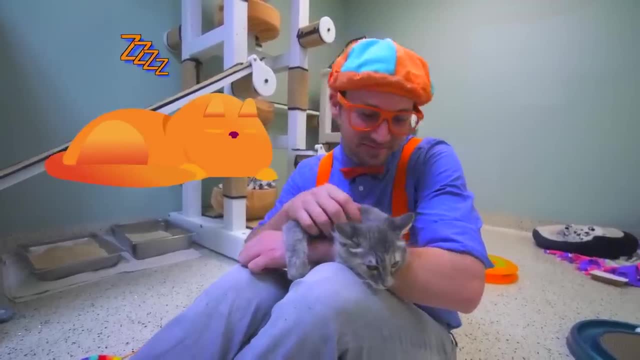 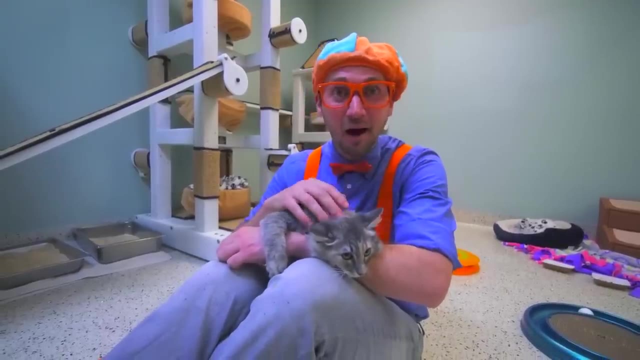 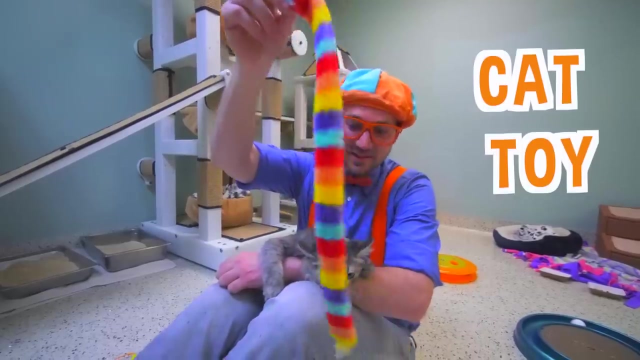 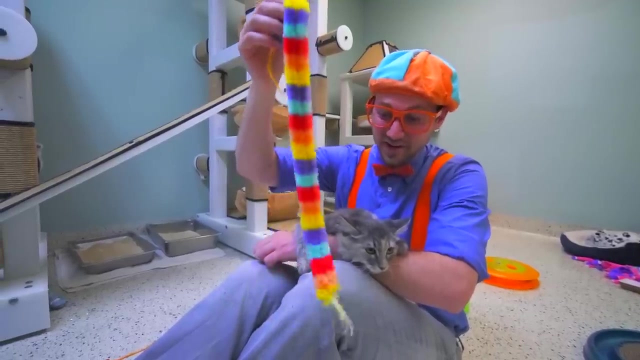 in the middle of the day, when sometimes you take a nap. This kitty just took one of those. I wonder if the kitty had a dream. Yeah, look at this, This is a cat toy. Hey kitty, Hey kitty. I don't think it wants to play right now, but 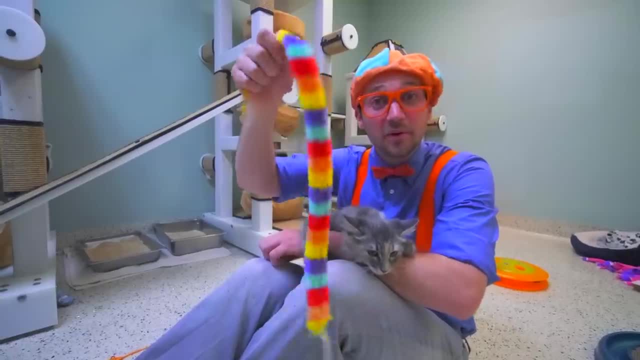 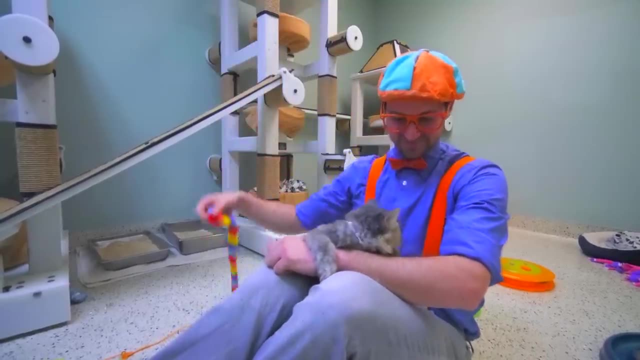 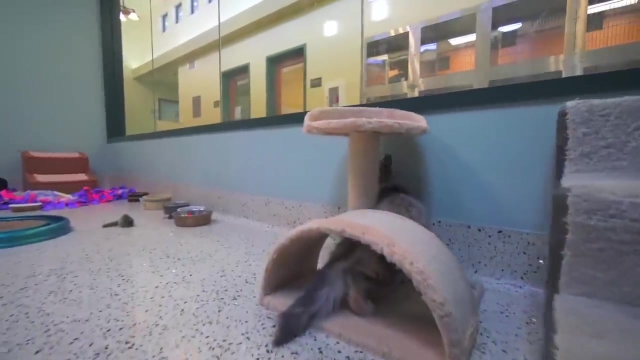 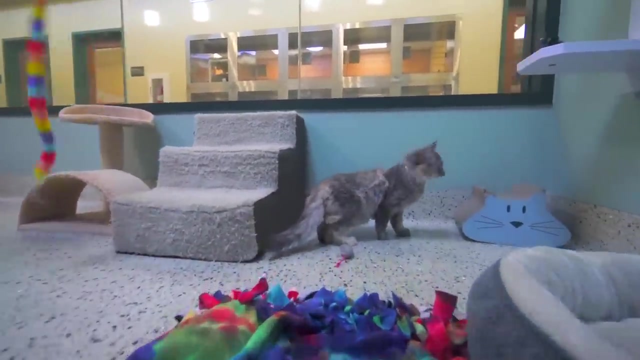 cats love to play and it's really important to play with your pets. I don't like this. Kitty kitty, kitty kitty. Hey, kitty kitty, That's funny. Oh, Oh, Oh, Oh, Oh, Oh Oh. 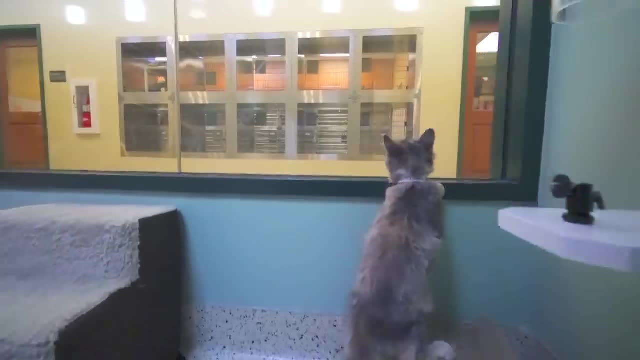 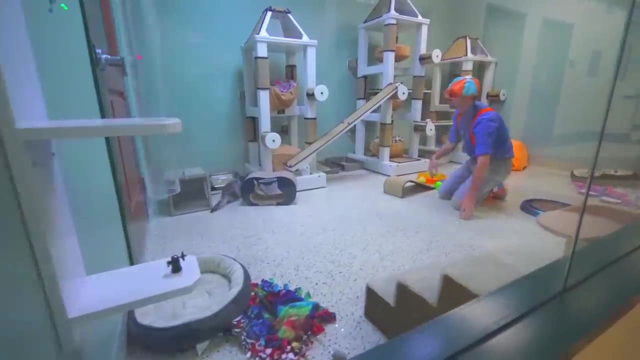 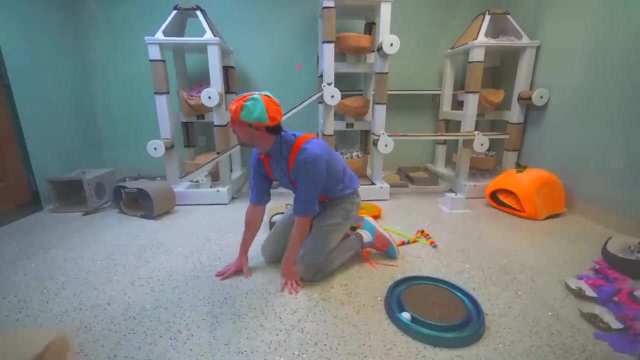 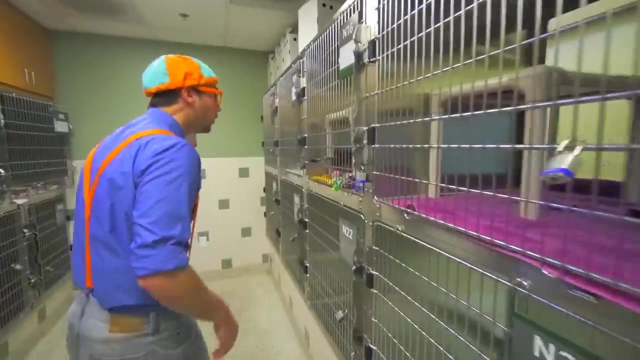 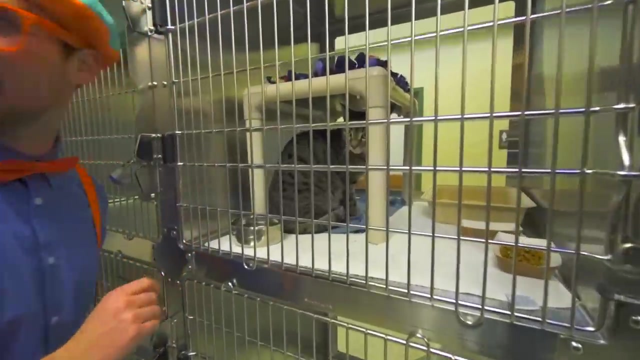 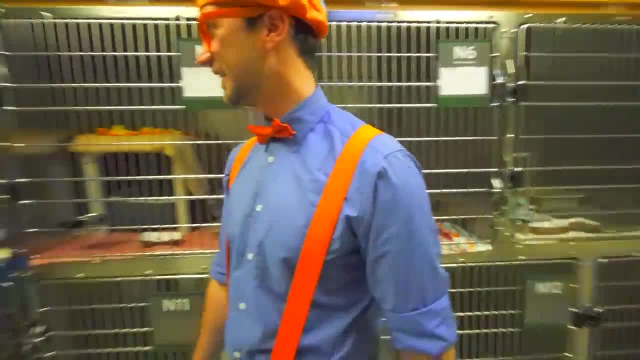 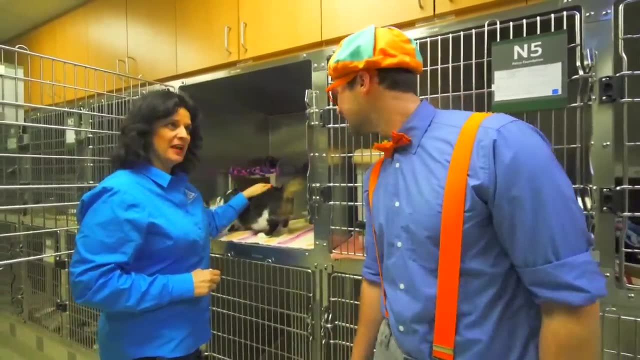 A lot of them are sleeping. Oh, hey, look, Hey, Hi, Ooh, what do you have here? I have Pumpkin. Pumpkin is one of the cats that we have available to find a new home today. Ooh Yeah, she came to us with nobody to care for her. 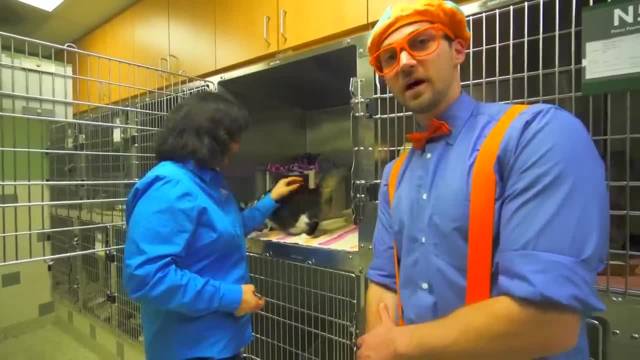 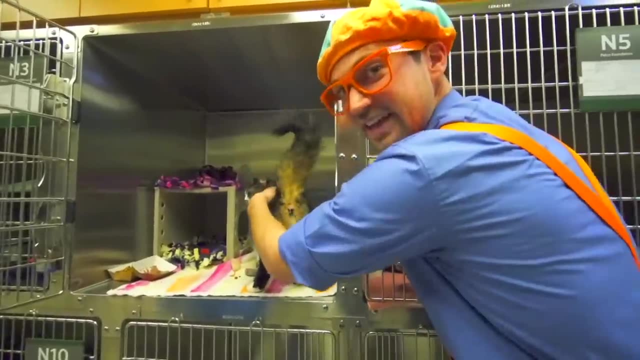 We're hoping somebody comes and takes her home and makes them hers. Oh, wow, can I pet Pumpkin? Sure can. Hey Pumpkin, Hey Pumpkin, Ooh, Pumpkin is really nice and really sweet. Hey, Wow, Isn't she pretty. 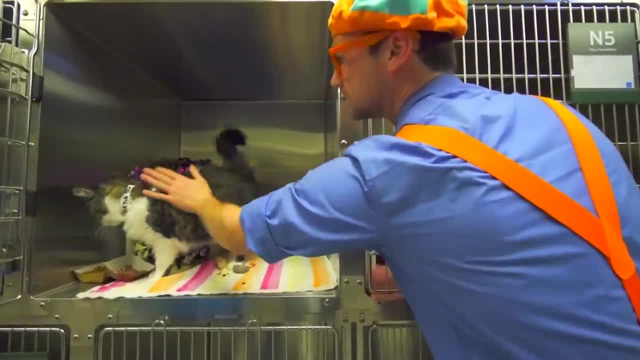 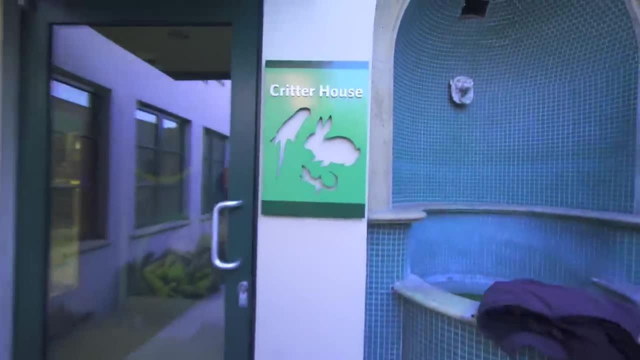 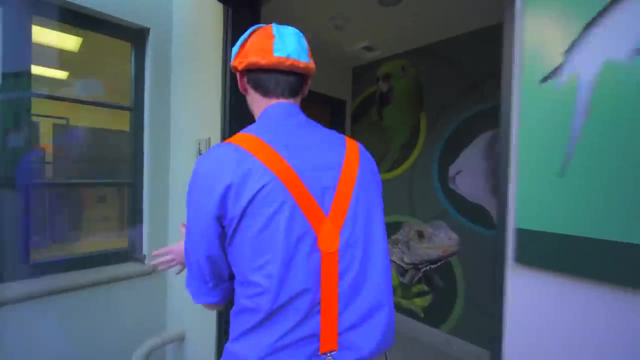 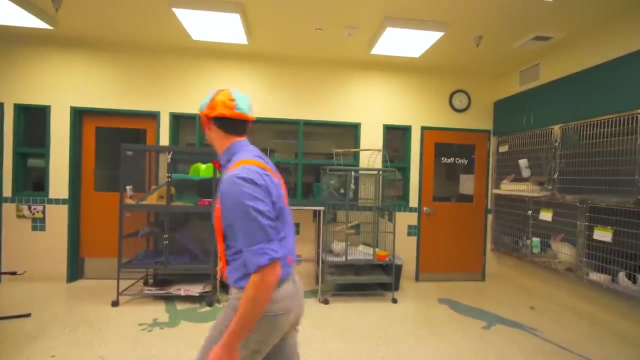 Yeah, she is. Look at her green eyes. Oh, so pretty. All right, buh-bye, Bye. Oh, the Critter House. I wonder what kind of critters are in here. Come on, Wow, This room is great. 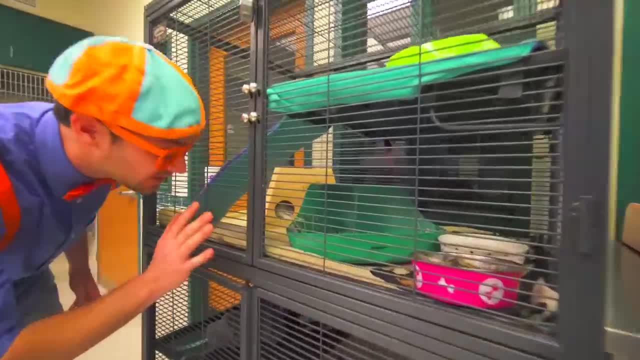 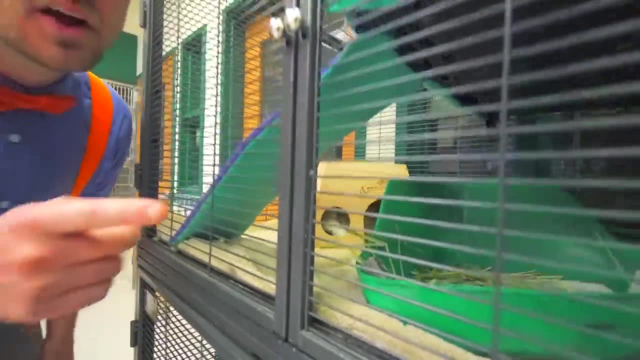 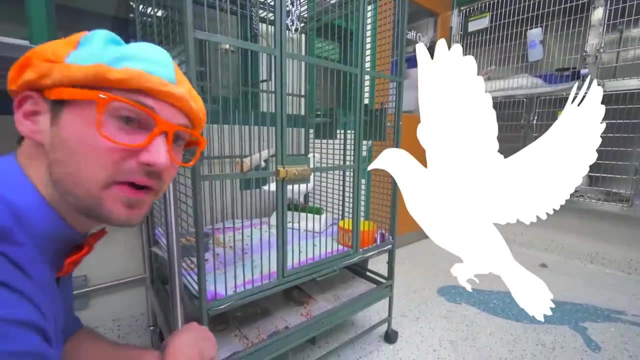 Ooh, look, Hello, It's sleeping, but there's a guinea pig right here. Oh, that's funny. Okay, Ooh, what's over here? Oh, Hey, birdie. Oh, It's a bird. 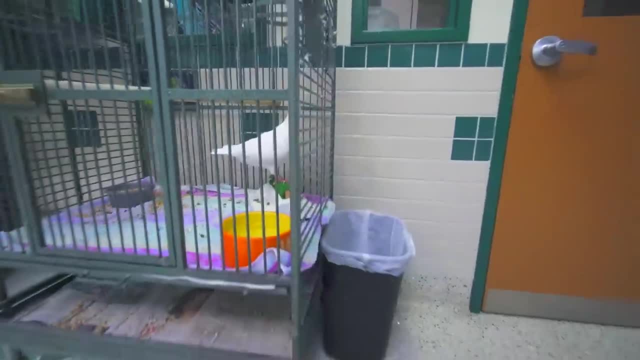 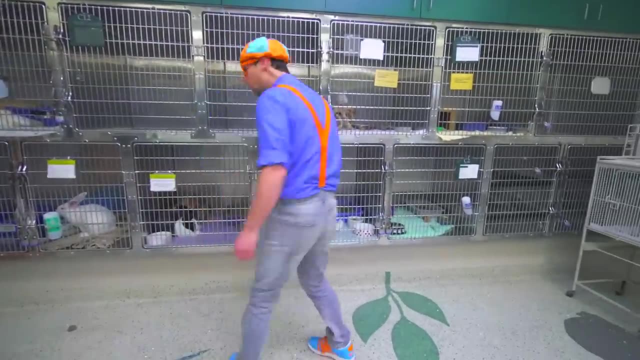 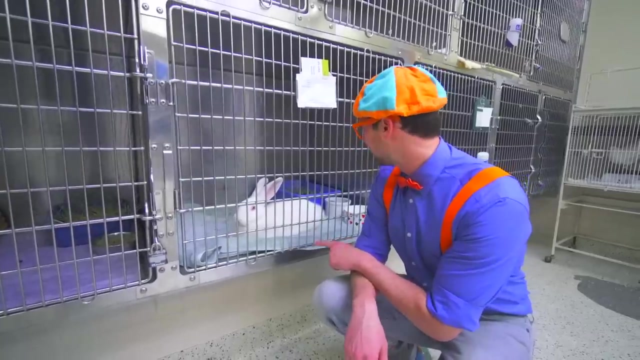 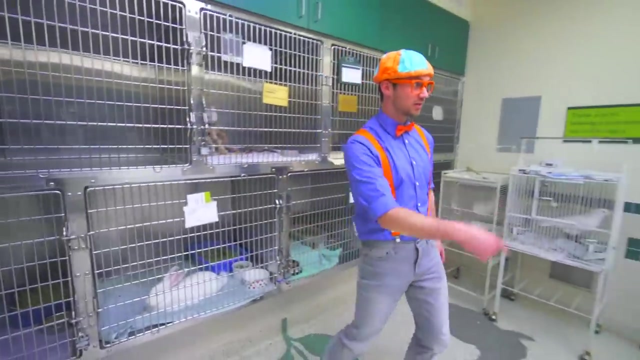 Look, Coo coo, Cute little bird. Ooh, look, That bird was white. And look, There's a white rabbit. Wow, You see that rabbit. Hey, I have a treat for you. Come look over here. 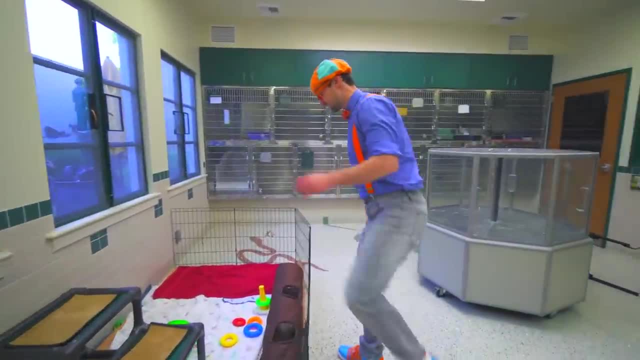 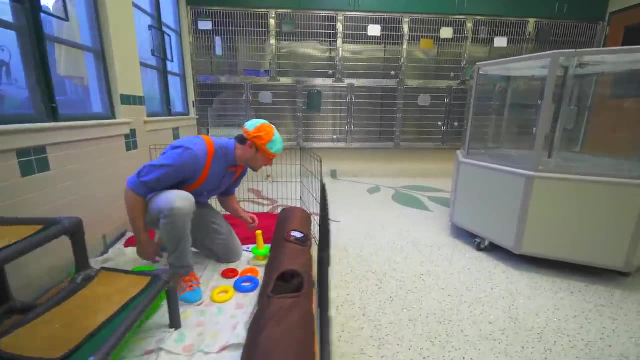 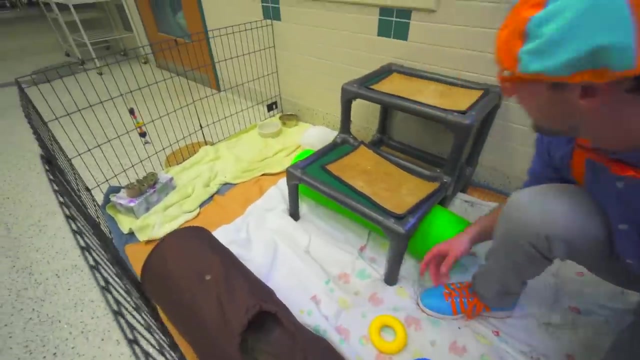 Wow, I have a rabbit, friend right down here. Huh, Okay, Oh, where are you going? Oh, look, Hey rabbit. Oh, there it is, Hey, It's running around. Hey, Oh, Hello, Oh, ho, ho. 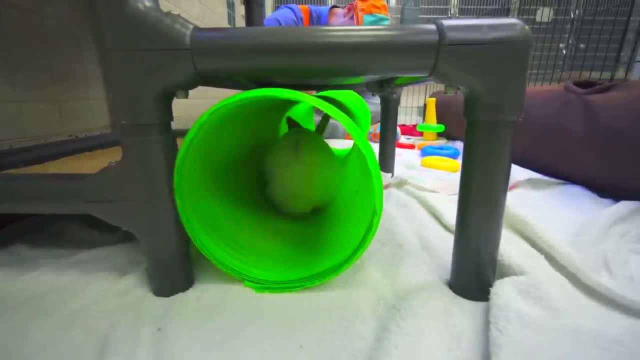 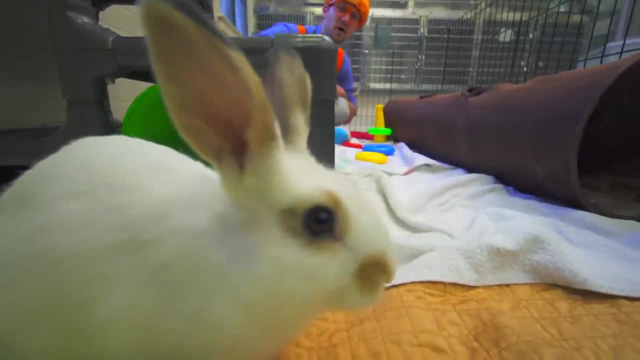 Rabbits have really big ears. Oh, Okay, Rabbit. hey, How are you? Oh, It's really soft, And their ears are so soft. Oh ho ho, There's a rabbit, There's a rabbit, Okay. 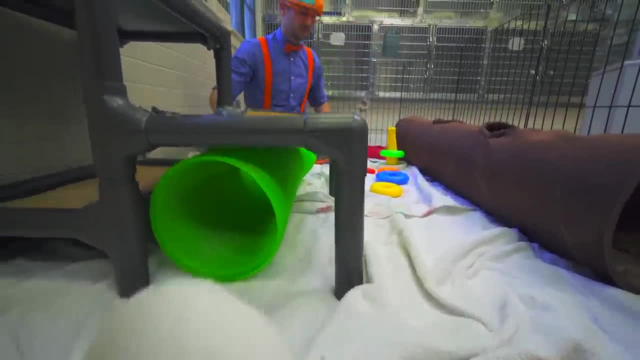 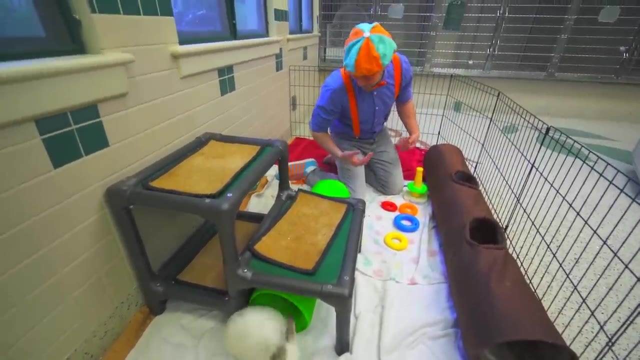 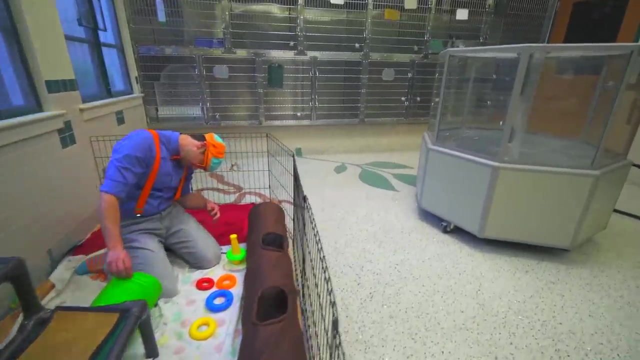 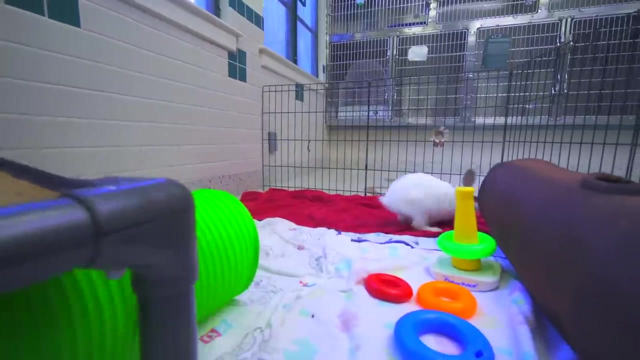 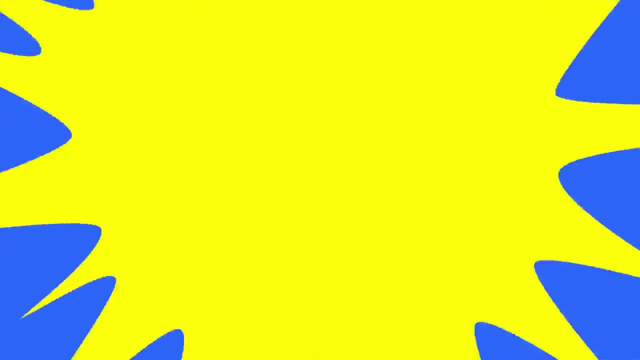 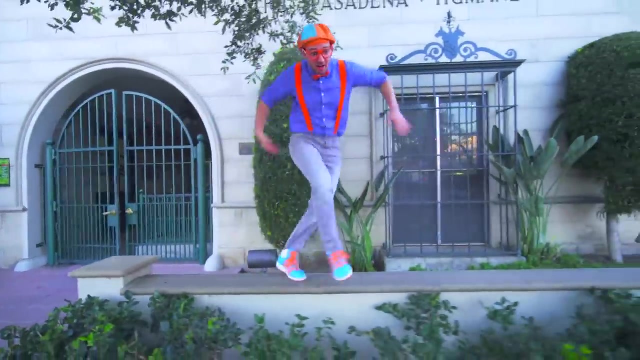 There's a rabbit: Rabbit Rabbit, Hey rabbit, Hey, Rabbit, Rabbit, Rabbit, Rabbit, Rabbit, Rabbit Rabbit. There's a pig. Okay, buh-bye, Yoo-hoo, That was awesome, Yeah. 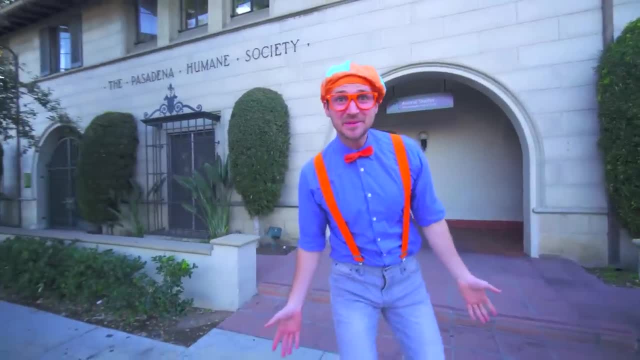 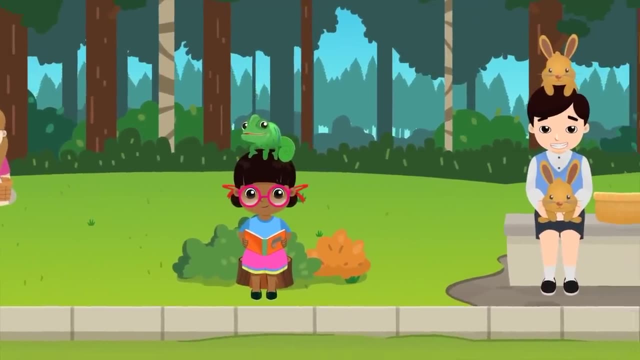 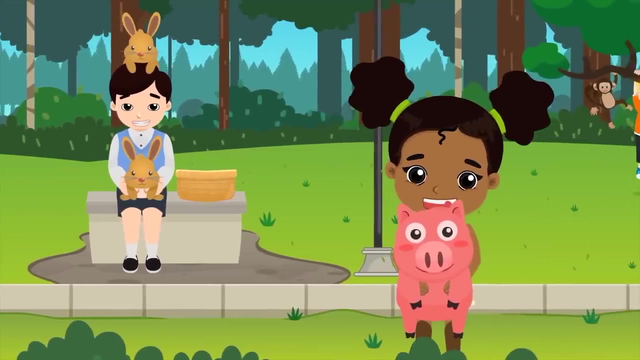 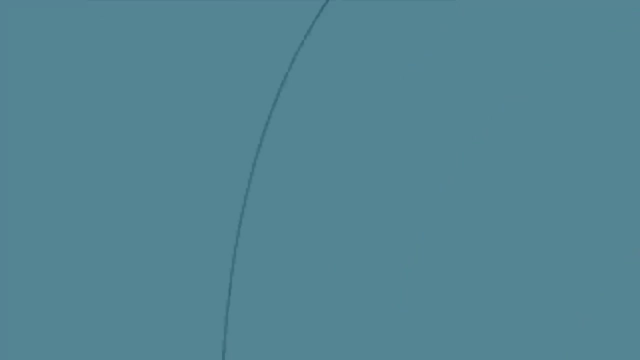 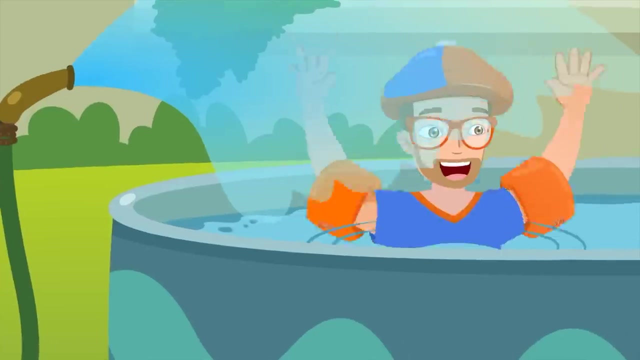 Ha-ha. So many cute animals. Well, see you later. Buh-bye. A pet keeps you company. It will be there whenever you're in need. It cheers you up when you've had a pet Every day. a pet can be your best playmate. 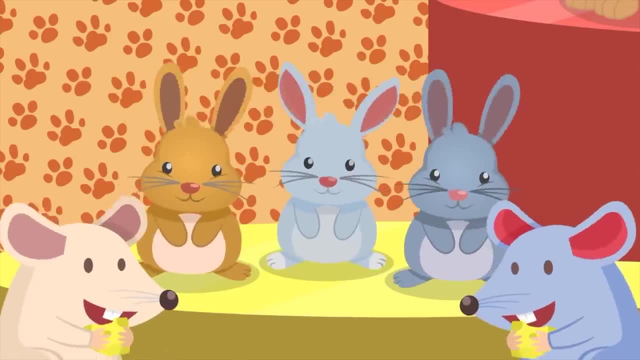 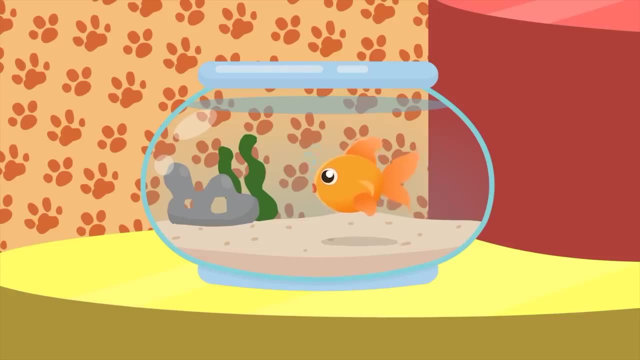 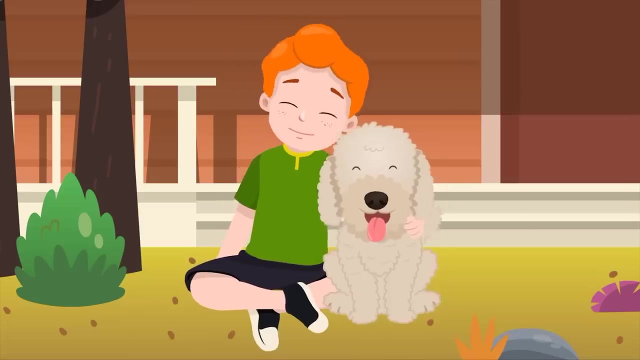 Dogs and cats, and bunnies and rats. these are the pets, pets, pets. Turtles and snakes, goldfish in a tank- these are the pets, pets, pets. My pet, my pet, is my very best friend. 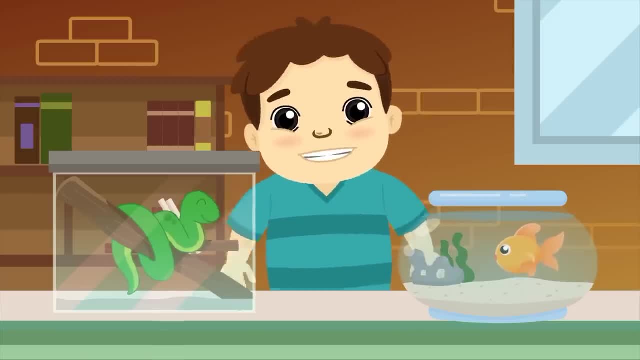 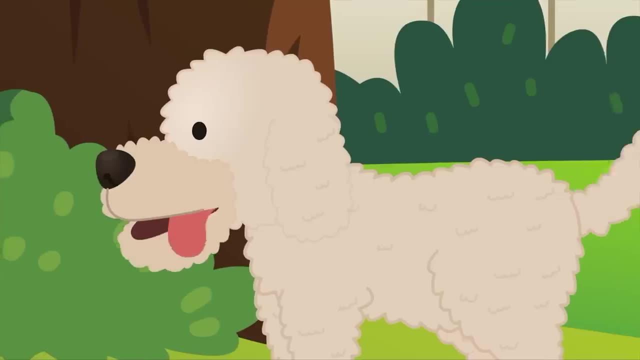 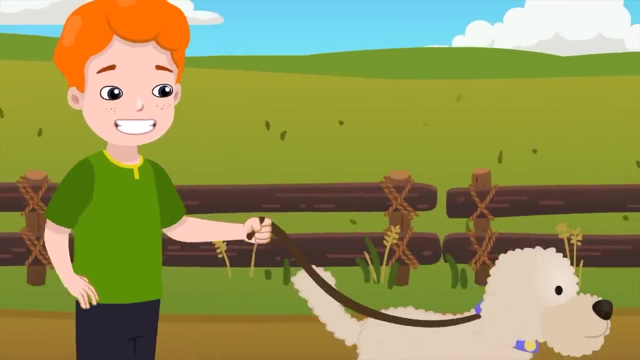 You've gotta take care of your pets. My pet, my pet, is my very best friend. You've got to feed them and clean them. Sometimes you've gotta teach them how to behave. Sit Fido, sit Some pets. you have to walk with them. 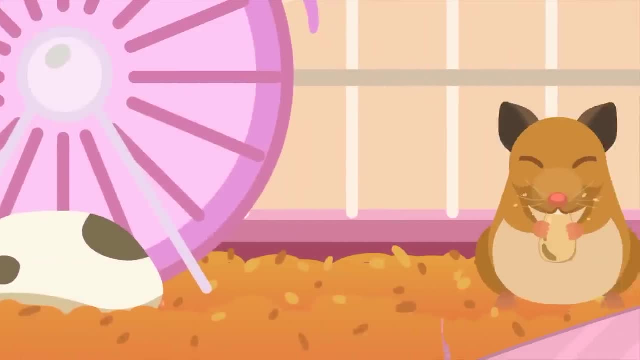 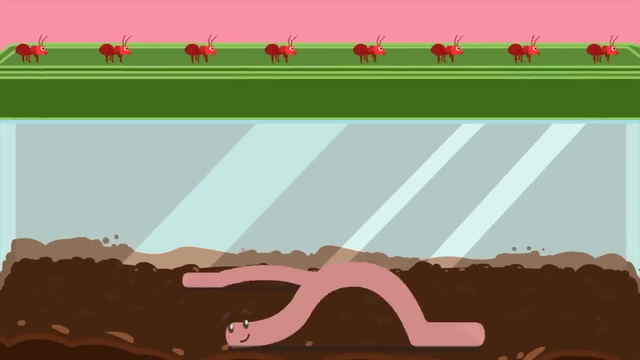 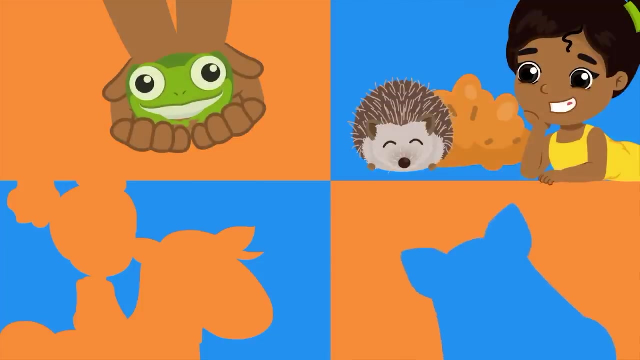 Others you can talk to them And some you have to clean out the cage: Spiders and birds and ants and worms- these are the pets, pets, pets. Ponies and frogs, hamsters and hogs- these are the pets, pets, pets. 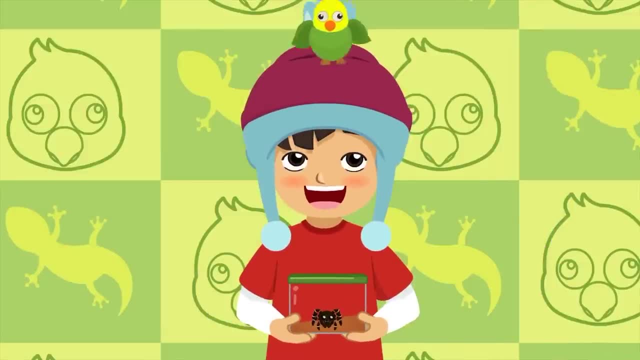 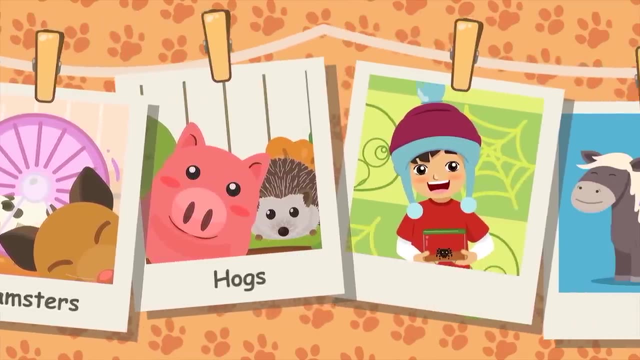 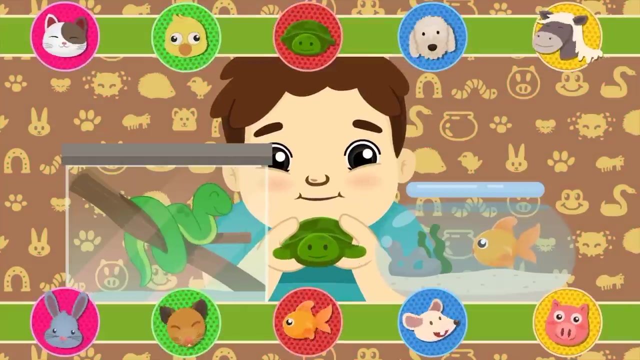 My pet, my pet is my very best friend. You've gotta take care of your pets. My pet, my pet, is my very best friend. Come on, everybody sing along. My pet, my pet, is my very best friend. 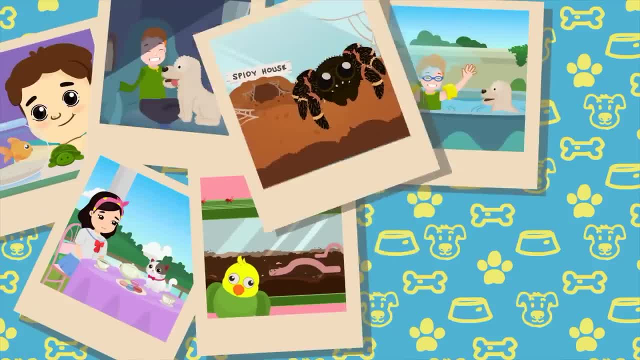 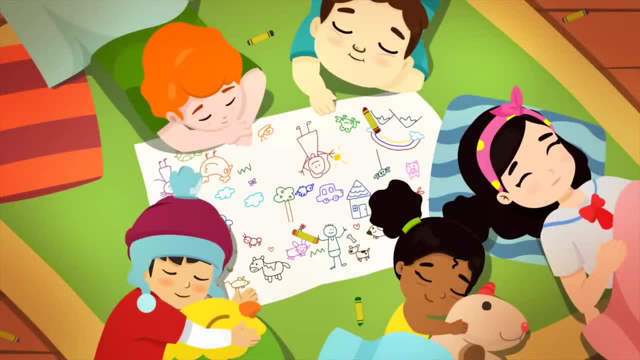 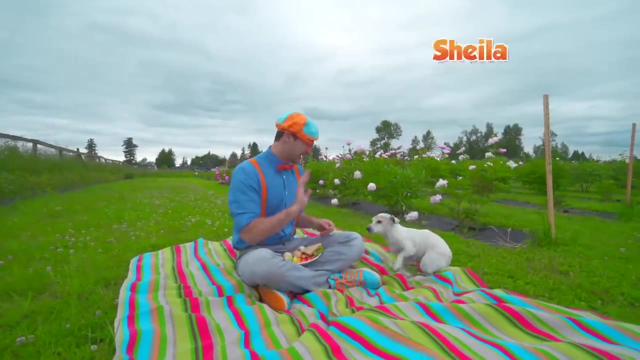 You've gotta take care of your pets. My pet, my pet, He's my very best friend. we've got to take care of your pets. Oh, hey, it's me Blippi, and this is Sheila. Hey, Sheila. 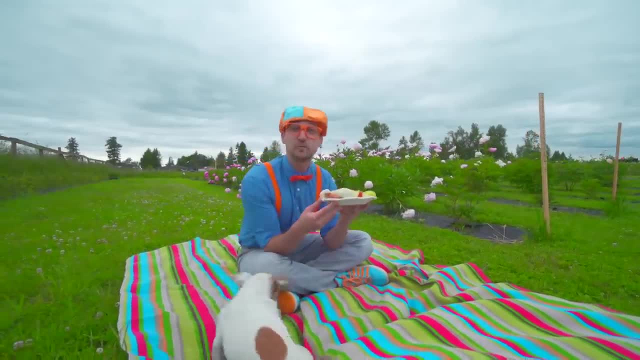 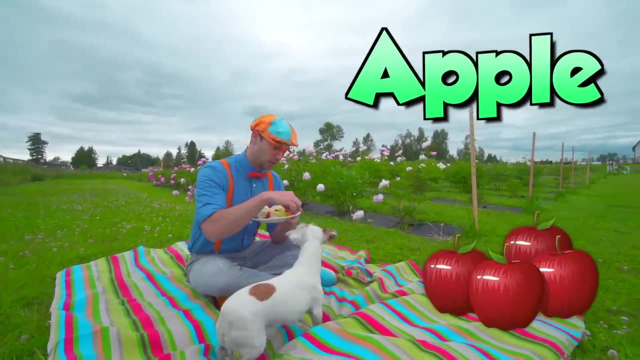 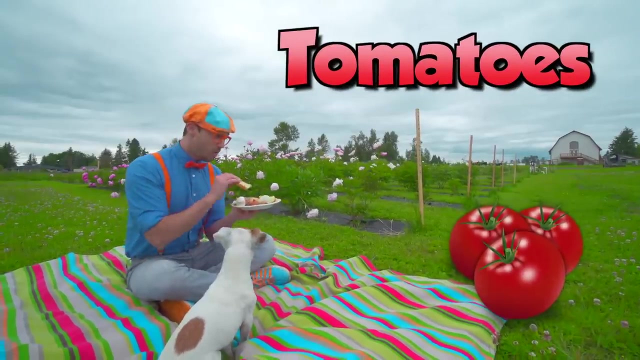 She's a farm dog, Whoa, and look at what I have. This is my lunch. I have a tasty apple- ooh, some strawberries, bananas, a sandwich with tomatoes on it- ooh, and even farm fresh eggs. 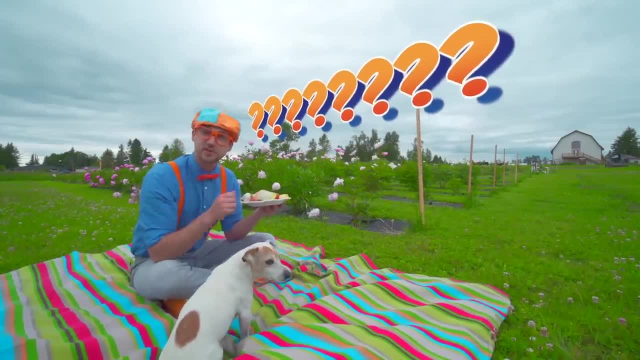 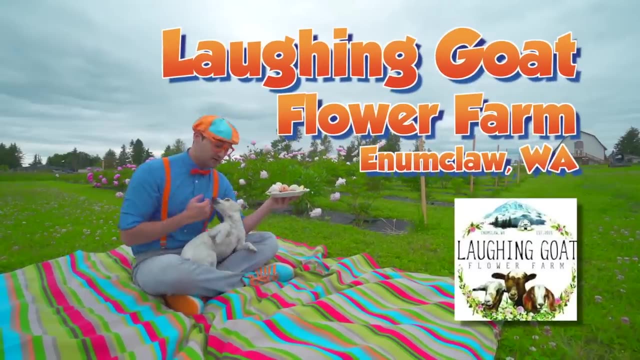 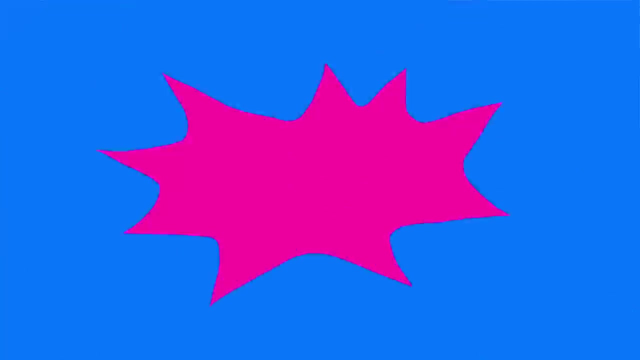 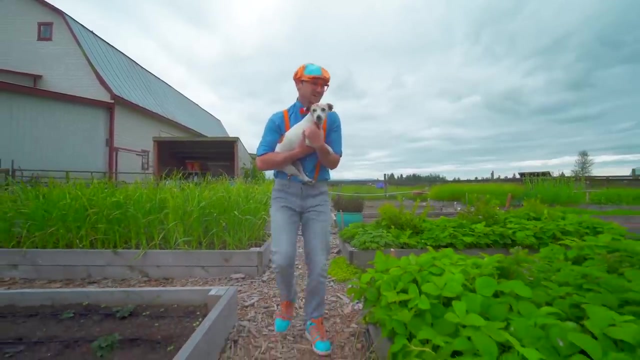 Wow, Have you ever wondered how this food gets to your plate? Yeah, I have too. So today we are at Laughing Goat Flower Farm in Enumclaw, Washington. This is going to be so much fun. Ooh, Sheila, look at these plants. 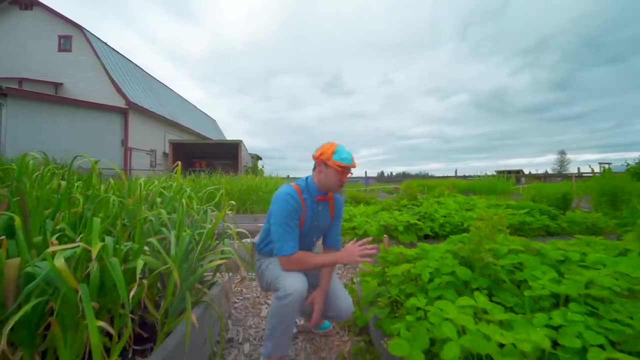 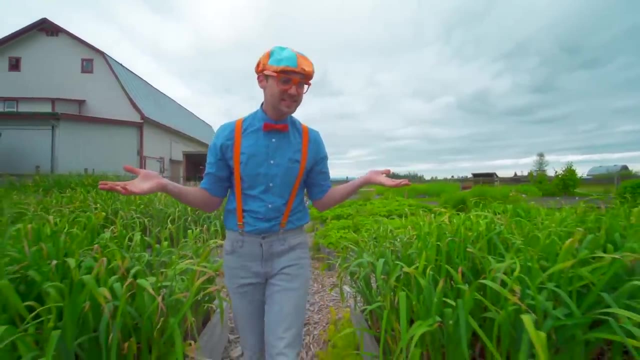 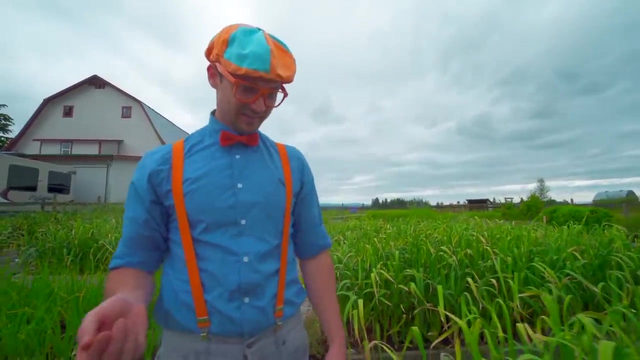 Whoa, these are strawberries and blueberries. Have you ever had a strawberry or a blueberry? Yeah, so tasty. Ooh. and look at these. Hmm, pretty interesting looking. This one is a strawberry. This plant, yeah, this is another fruit or a vegetable. 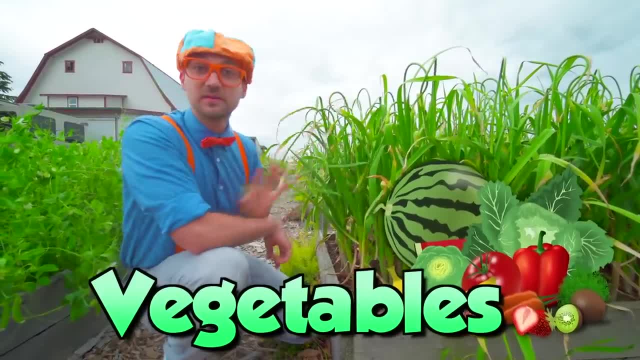 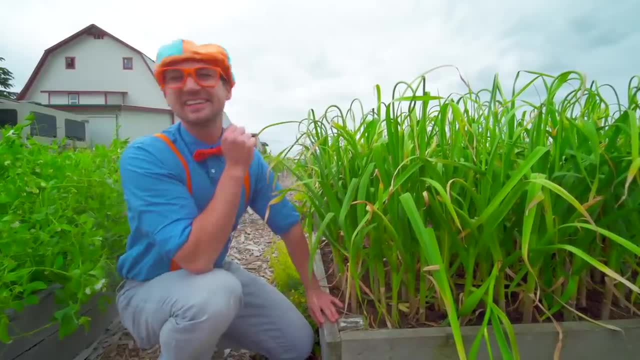 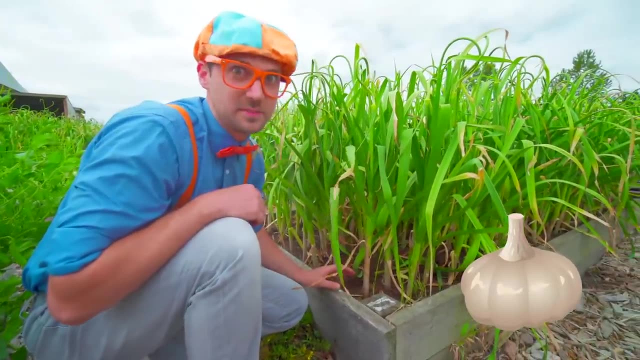 Yeah, this one's a vegetable, and this vegetable is called garlic. I love garlic. It makes my food taste so good. So garlic is actually a bulb right down there, but it's not ready to be harvested yet. But up here you can harvest the tops, and it's also tasty. 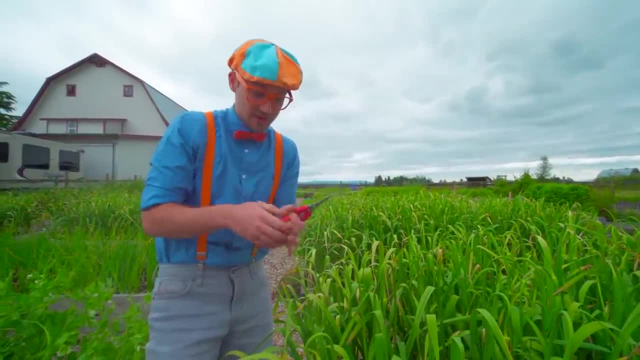 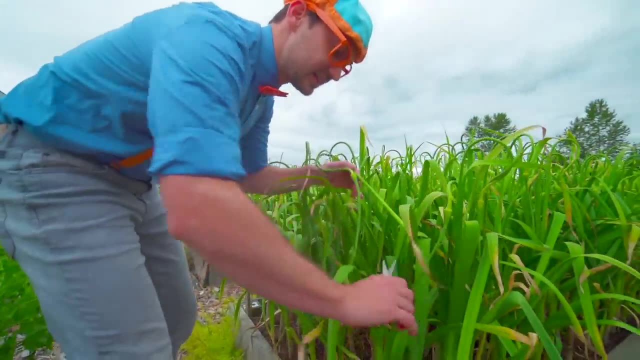 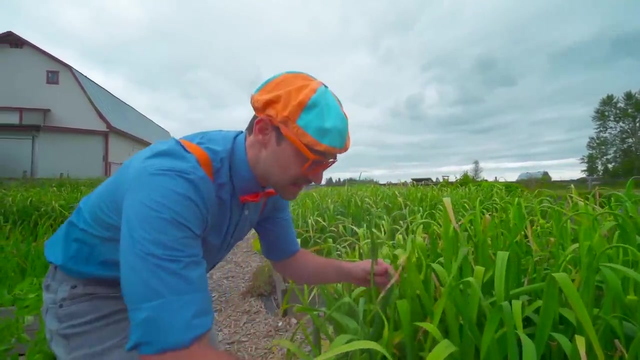 I'll show you how to do that. So I'm going to take these really sharp scissors, so I'm going to be very careful and I'm going to snip it right there. This is what it looks like, Whoa. one great thing about this farm is that all the food and the flowers are organically. 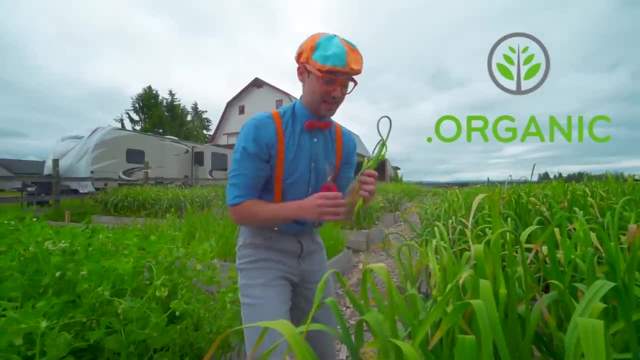 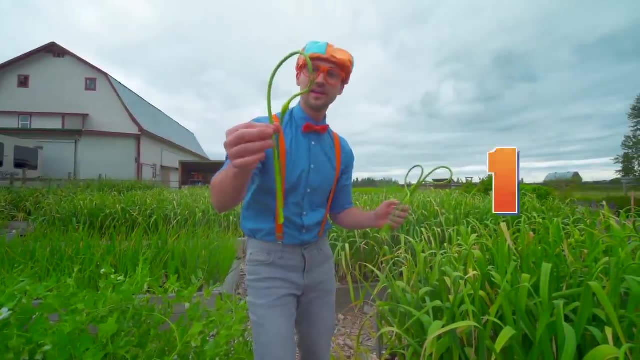 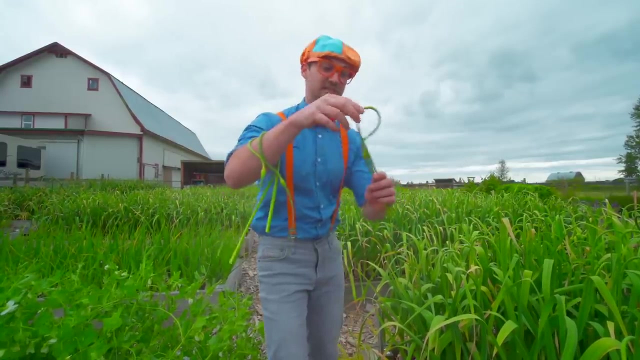 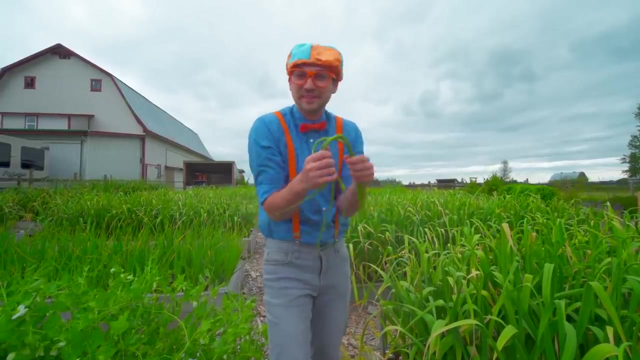 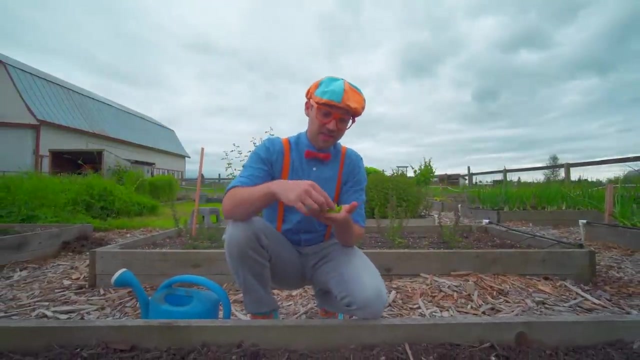 grown. This is going to be so tasty. All right, I think that's good enough. Let's count them. All right, we have one, two and three- Wow, three pieces of garlic top. Yum, Ooh, these are called snap peas. 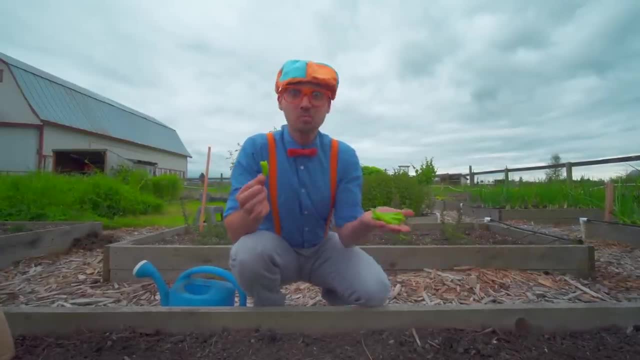 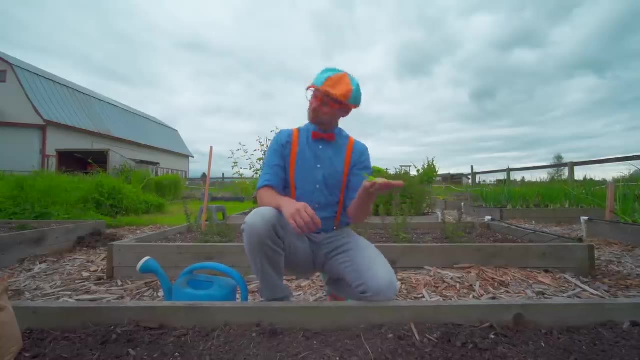 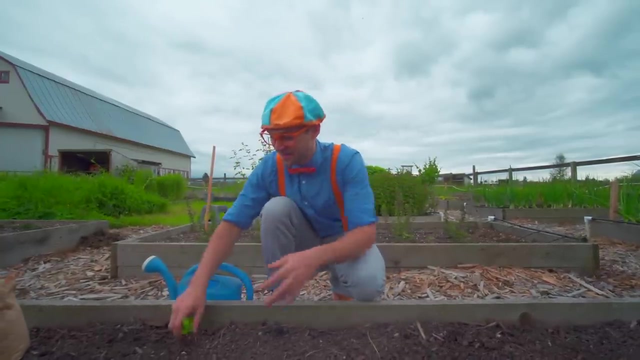 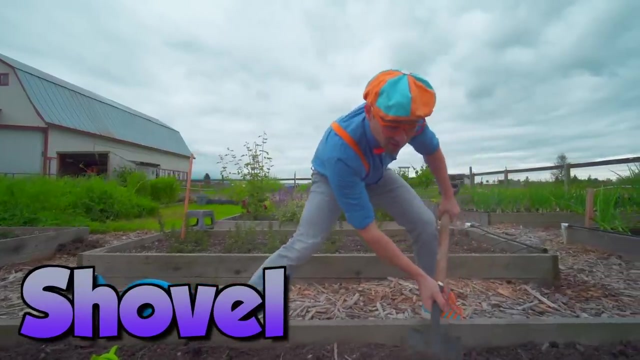 Mmm, And they're so yummy, Mmm, I think you and I should plant some snap peas. Okay, so, to plant some plants, some plants, you need a shovel where you dig a hole in a bed of soil, just like this, and put a seed right in the hole. 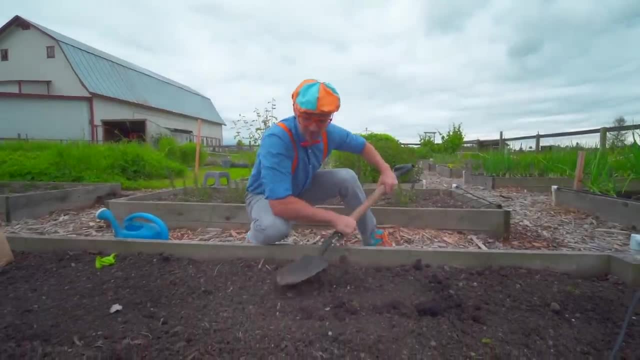 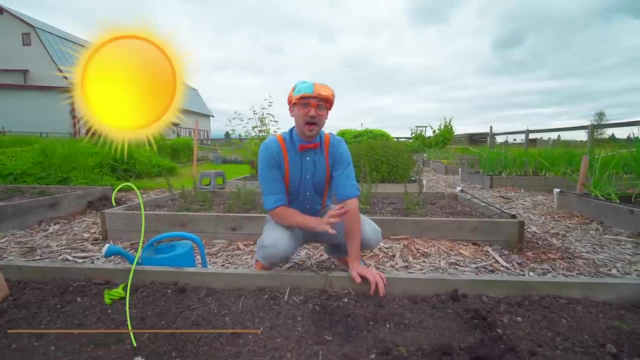 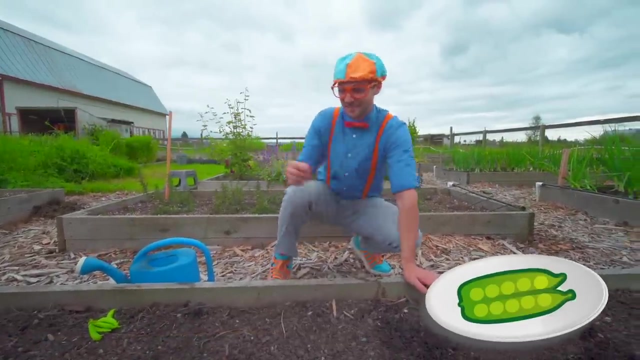 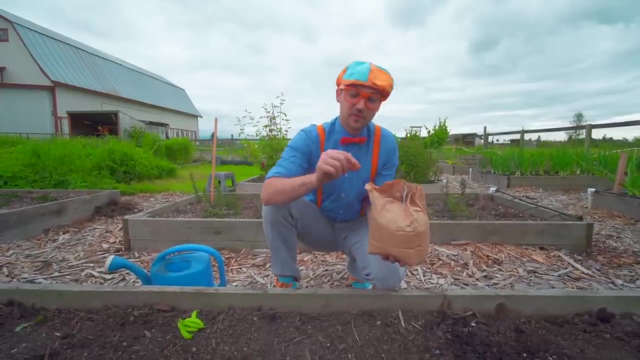 Fill it up. Fill up the hole, Put some water on it And then, after a lot of sun and some more water and a lot of love, it'll grow into a tasty plant. All right. but for snap peas, all you have to do is put one of these plants in a box. 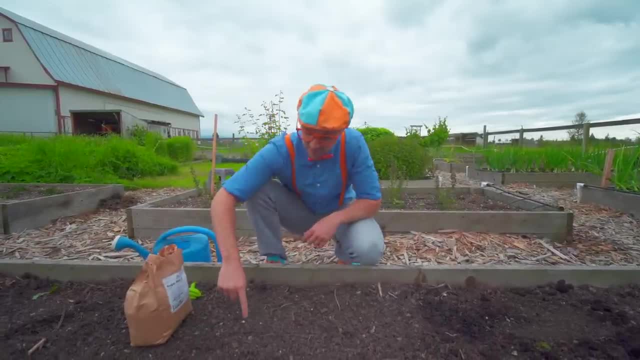 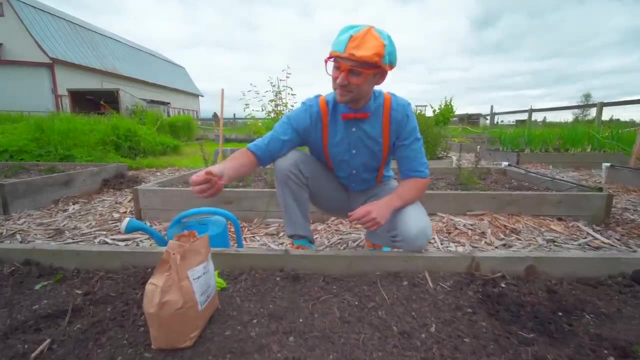 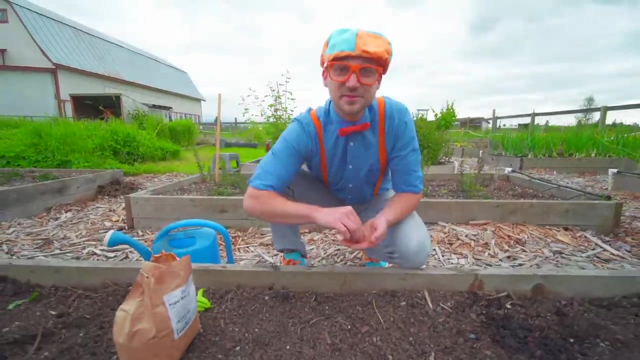 right on top of the soil, All right. And push it down to right about there, Perfect. And then you take another one and push it down. Let's do a few more together, All right. This is really fun. Look at them. 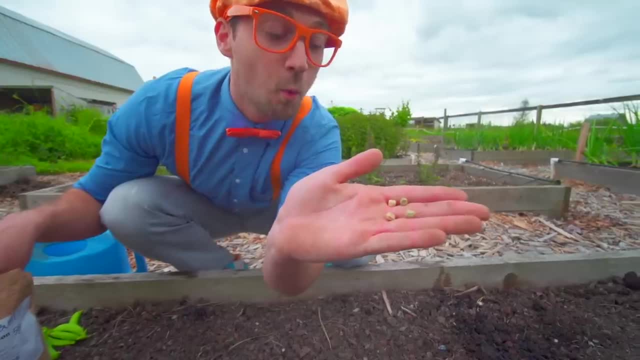 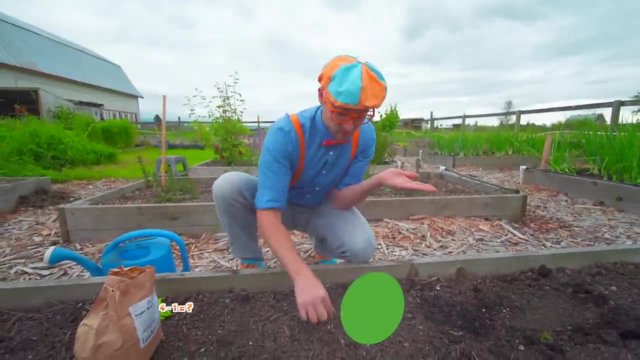 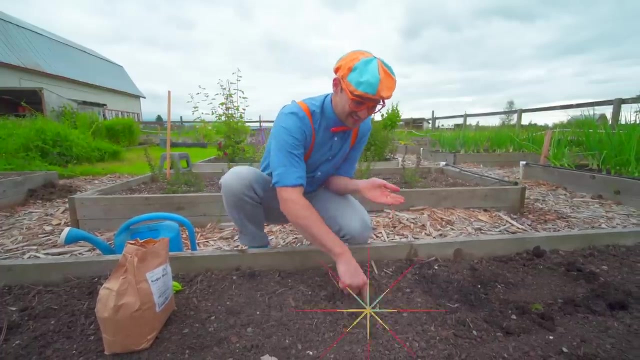 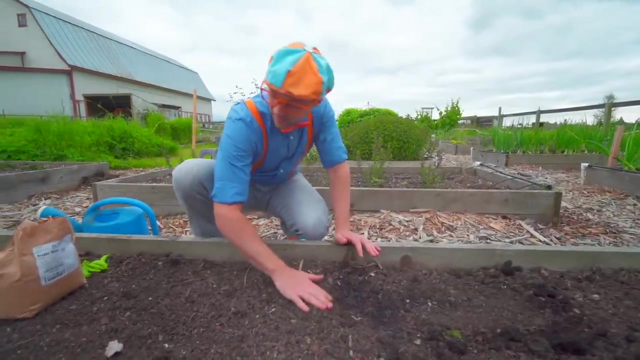 See, Let's count them: One, two, three, four, All right, Four minus one is three. Whoa, All right. Let's put the rest of these down inside the soil. There we go, Okay, So we have a bunch of them right in a line, right here. 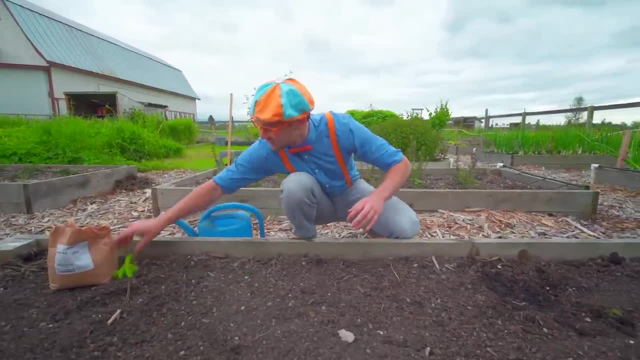 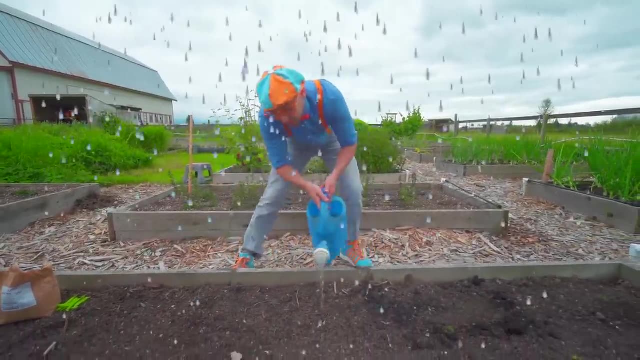 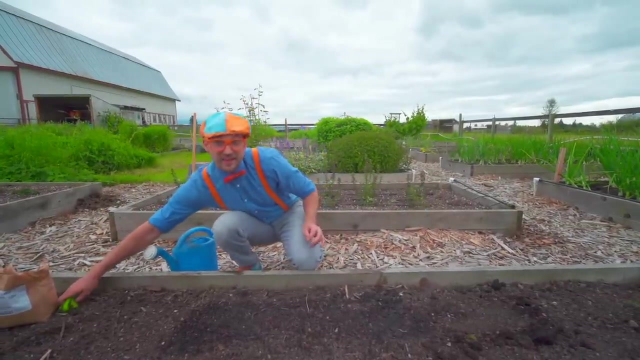 So let's move the rest of that and those And let's take the water and let's give them some water. All right, So we're going to take our water and let's give them some water. Wow, All right. Then in a while, these are going to grow into really big plants. 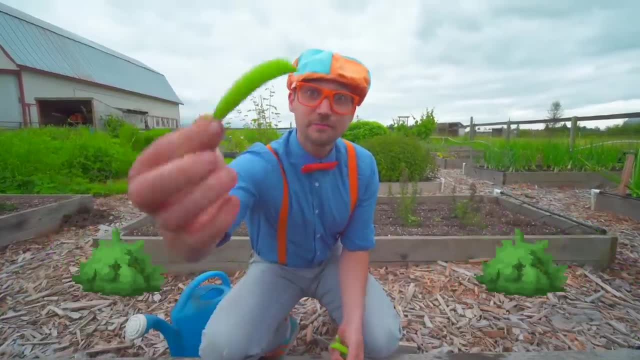 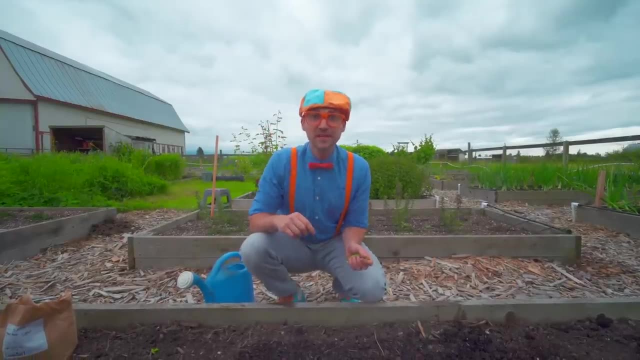 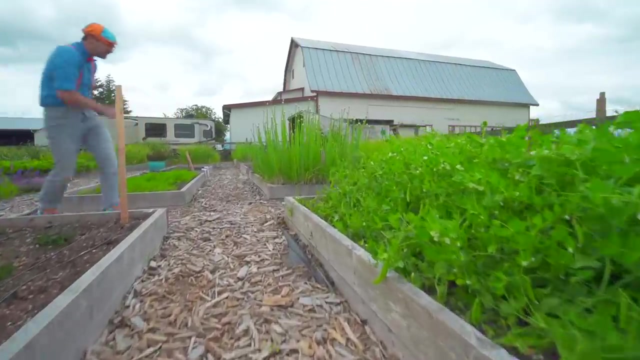 And then they'll grow these on them And then you can eat them like this. Wait a second, I think there's some big ones over there. Come on. Oh, there's a lot, Come on. All right, so those snap peas that we just planted. 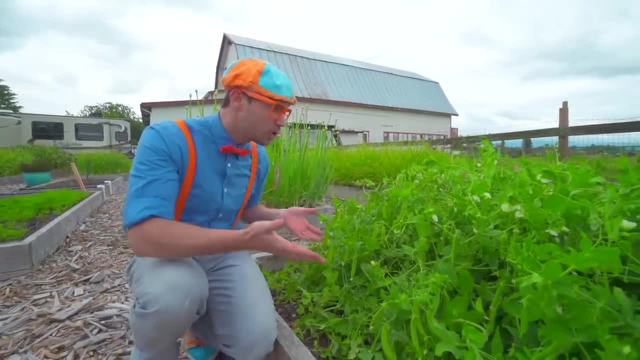 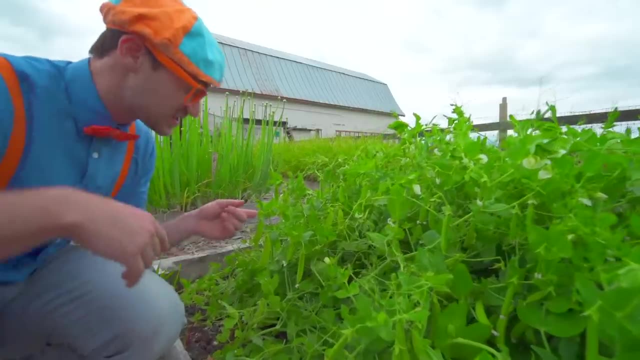 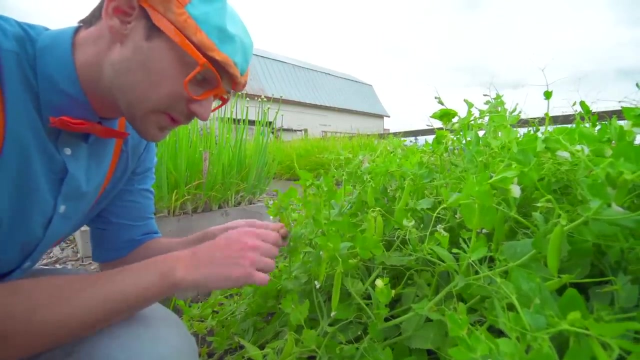 in seed form after two months are gonna grow to look like this. Look See, the plant has nodes and then those nodes grow the snap peas off of them. Ooh, pull it off and look, You have a lot of snap peas off this one plant. 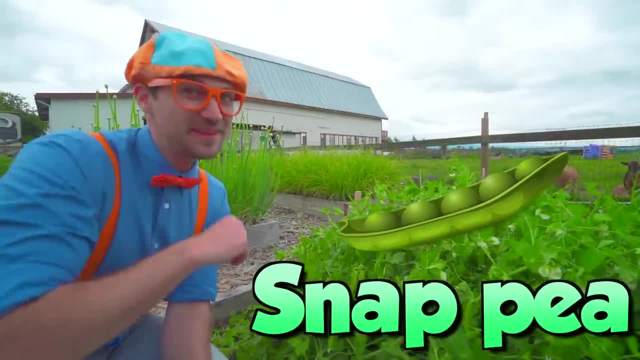 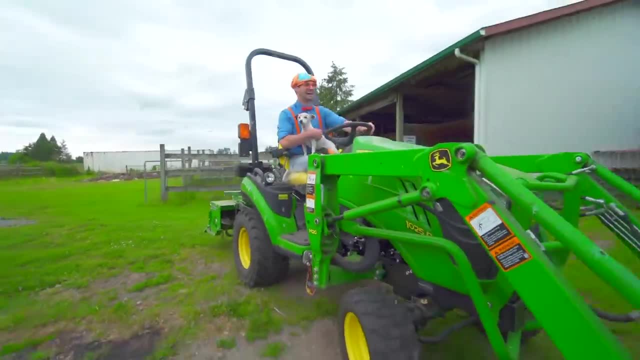 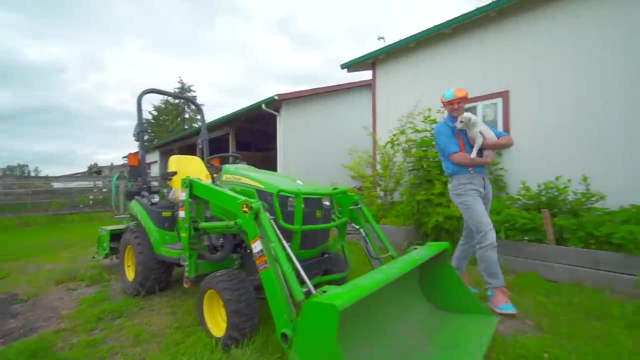 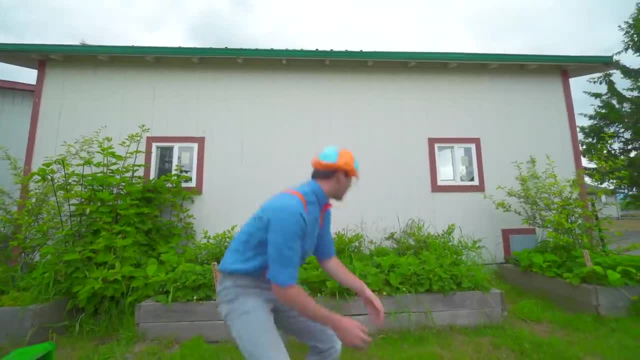 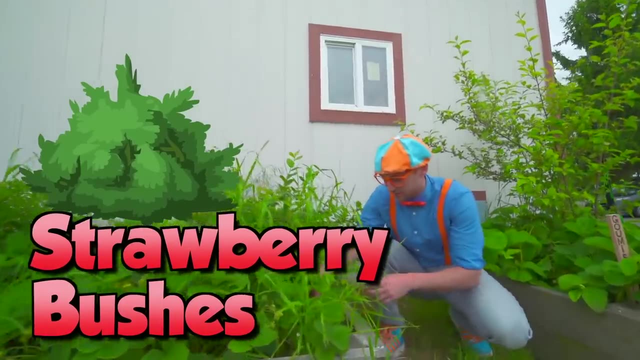 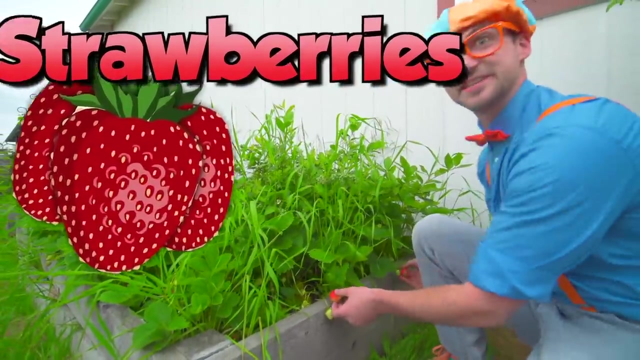 Okay, all right Time for some more food. Come check this out. Ooh, these are strawberry bushes. And look down here, These are strawberries, Really red strawberries. Let me pull it off. Yum, Mm, mm. 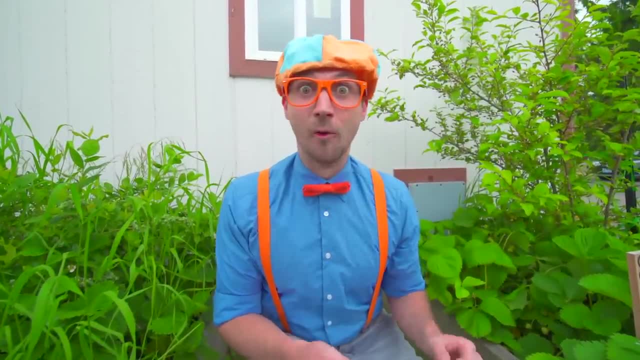 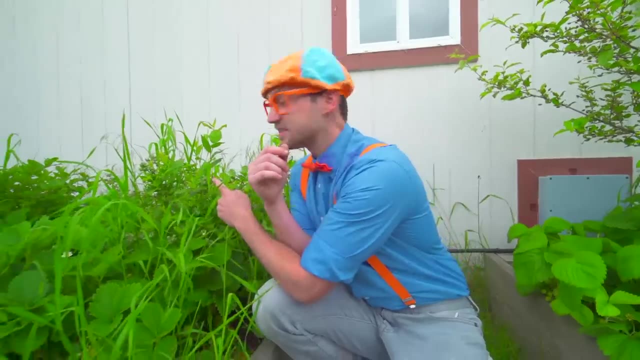 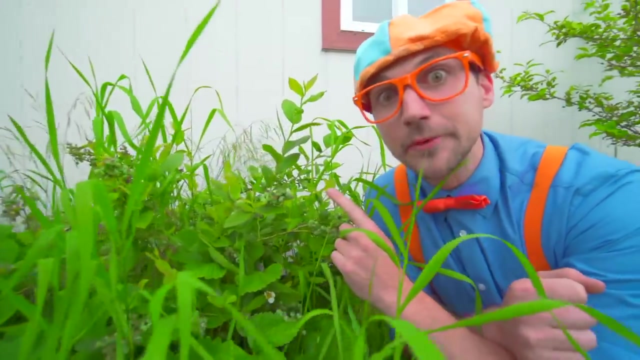 Mm. Wow, That was tasty. Whoa, I love strawberry bushes. Ooh, and here's some blueberries, But they're not quite ripe yet. See these. Yeah, they'll be blue when they're nice and ripe. 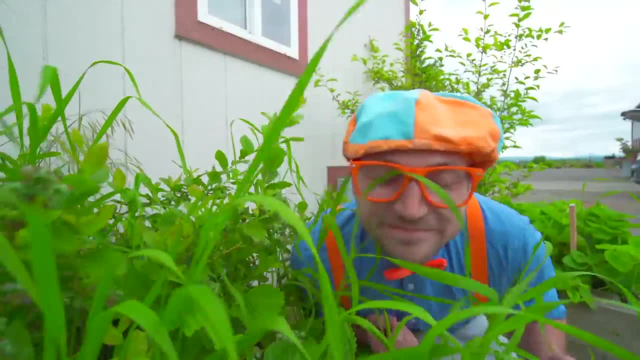 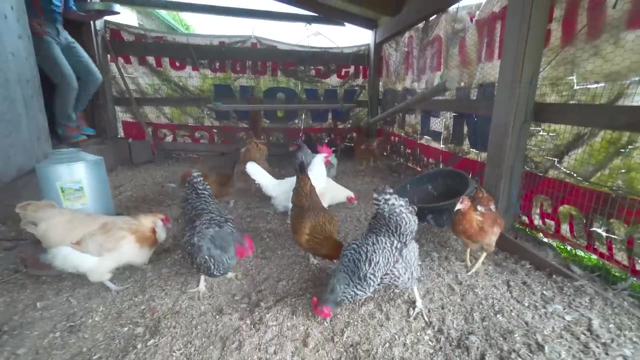 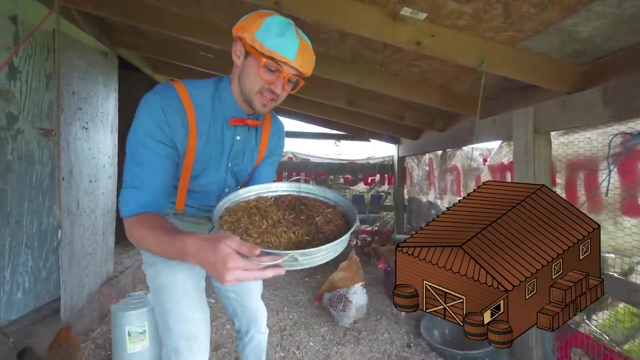 And then you can eat them. Ha ha, Ah, Ah, Ah, Ooh. Now we're in the chicken coop. Hey, chickens, Ha ha, And look, These are some tasty treats for the chickens. They love to eat these tasty treats. 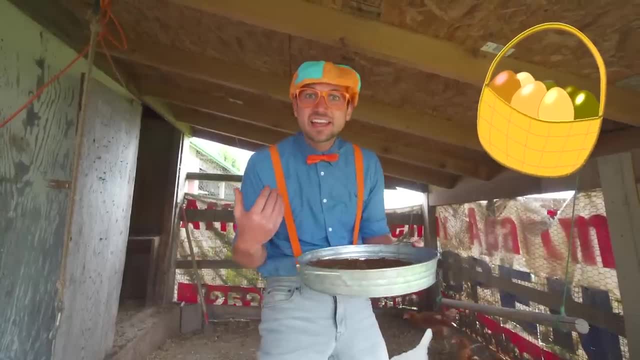 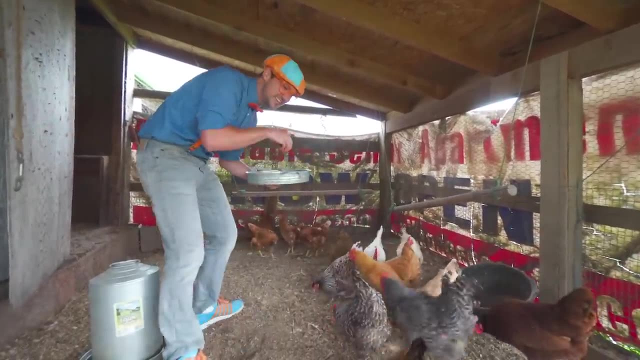 So then they lay lots of eggs. I love eggs For breakfast, of course. All right, here you go chickens. Ha ha, Whee, Here you go. Oh yum, Yum, Yum, Yum Yum. 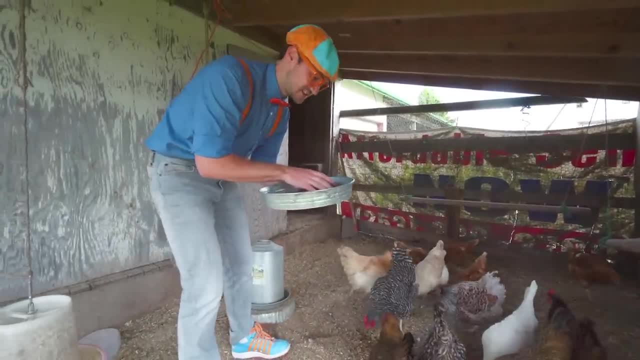 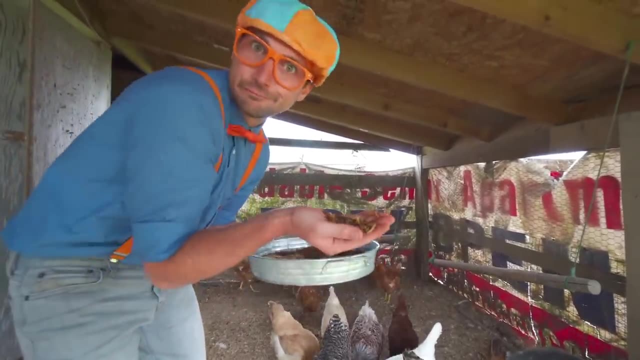 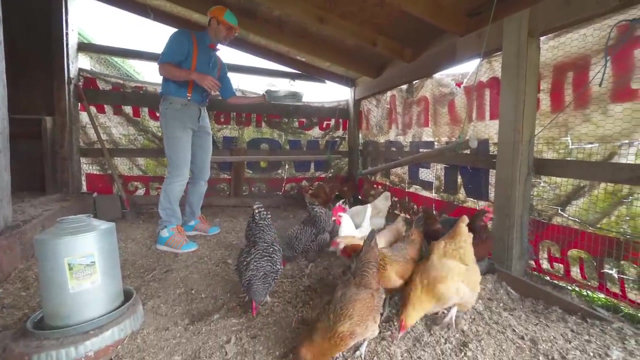 Yum, They love these tasty treats, Just like how I love fruits and vegetables. these chickens love this stuff. I don't know what it is, though, Here you go, All right. All right, There you go, And from there you can spread the rest around. 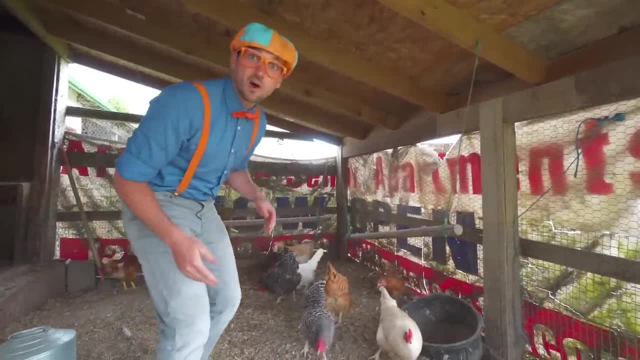 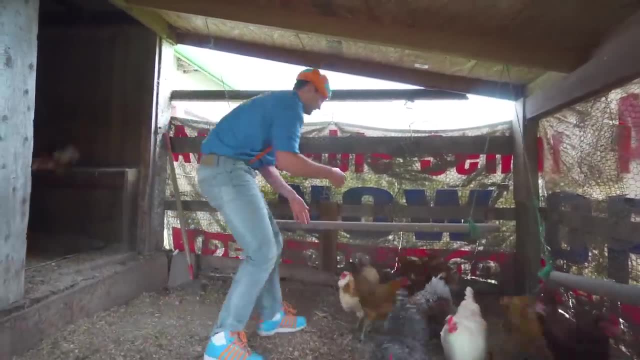 Here you go, And now I'll pick one up so I can pet it. Oh Look, I have a chicken And they love to be pet on their head. Oh, Oh, Oh, Oh, Oh, Oh, Oh. 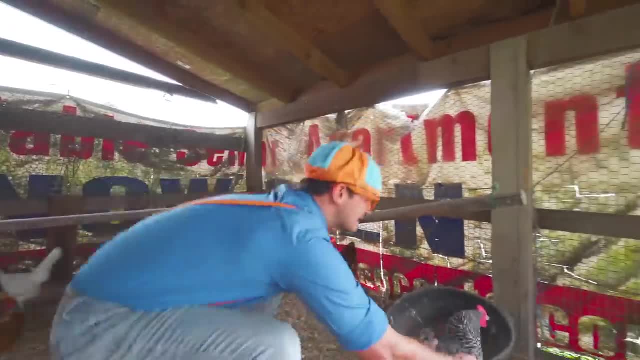 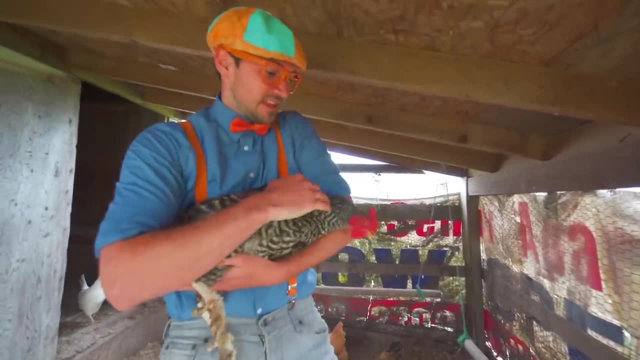 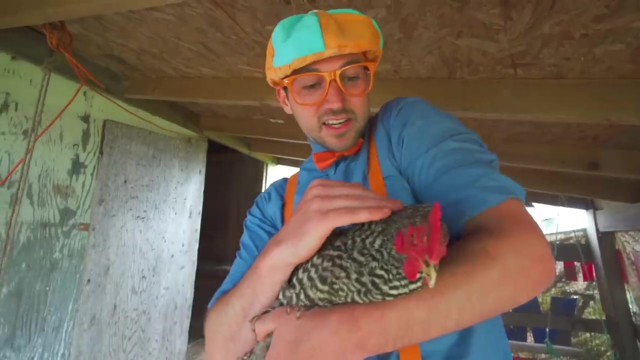 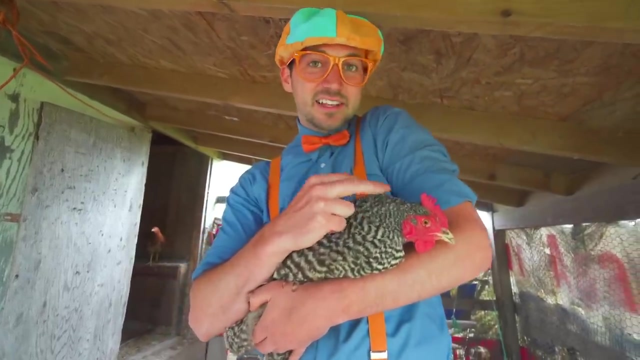 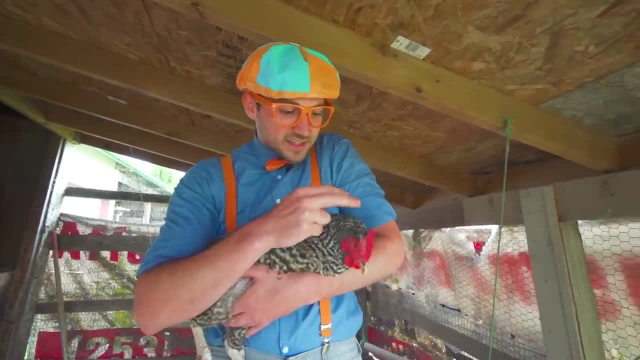 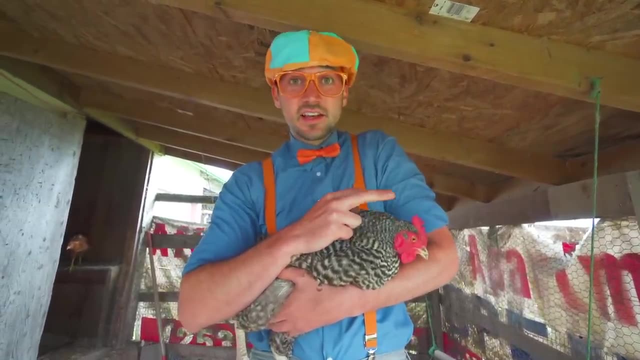 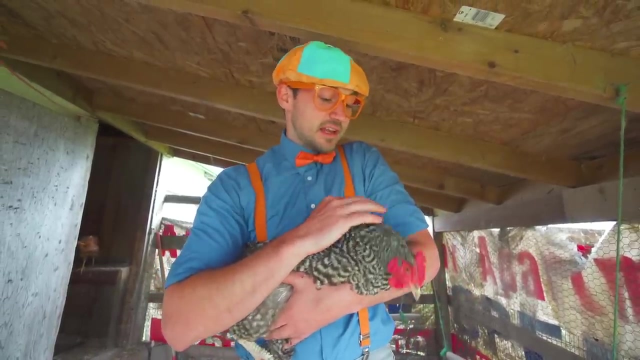 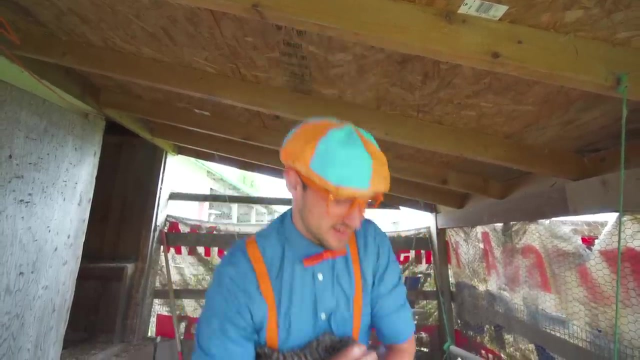 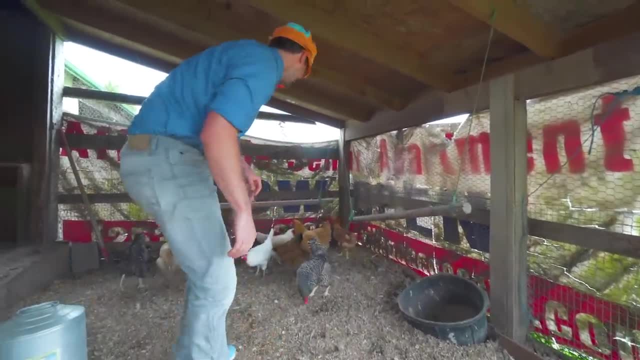 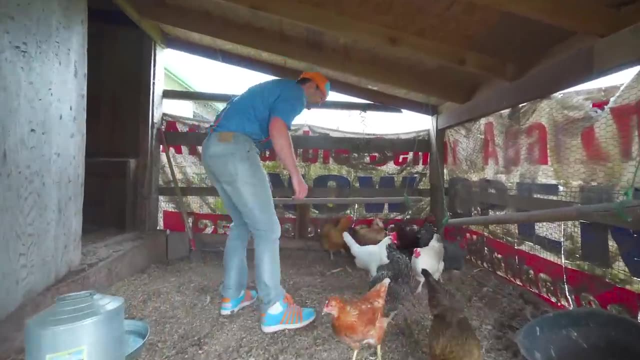 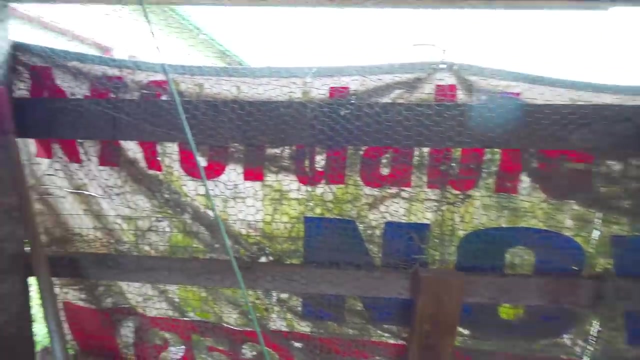 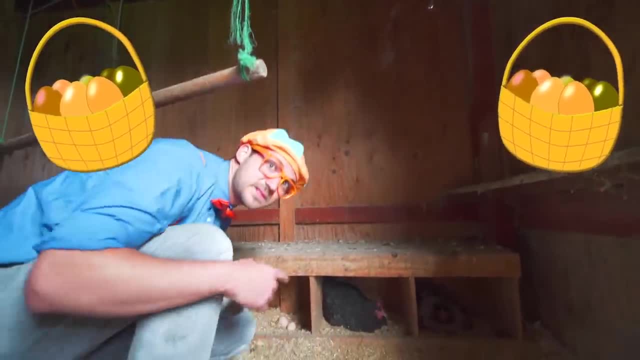 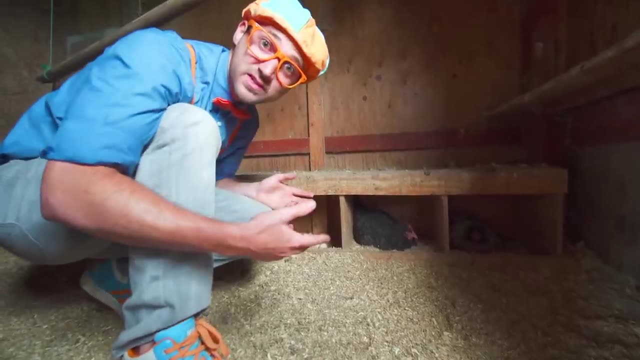 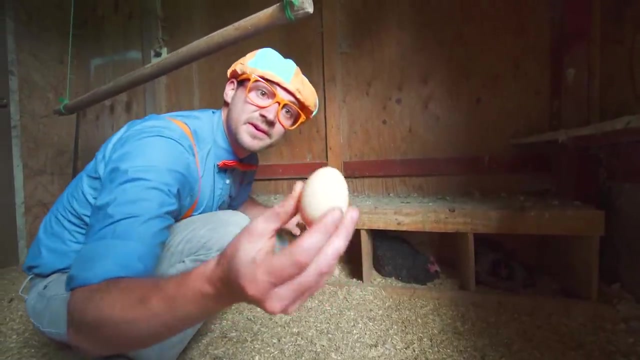 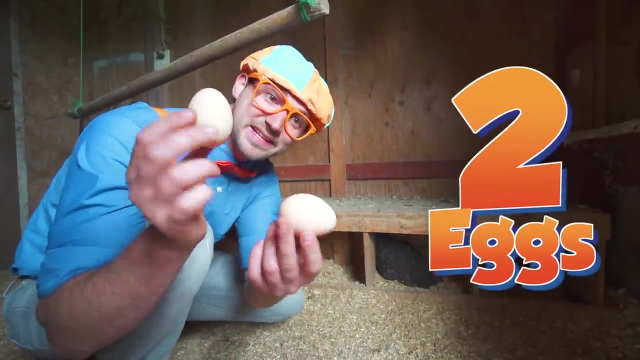 Come here. Whoa, see them down there. Yeah, they're laying eggs And if you look right here, there's a couple eggs ready for us to grab. look Right down there. One egg, Two eggs, Yum. 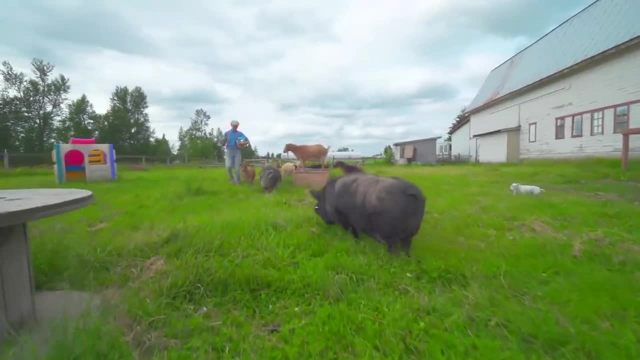 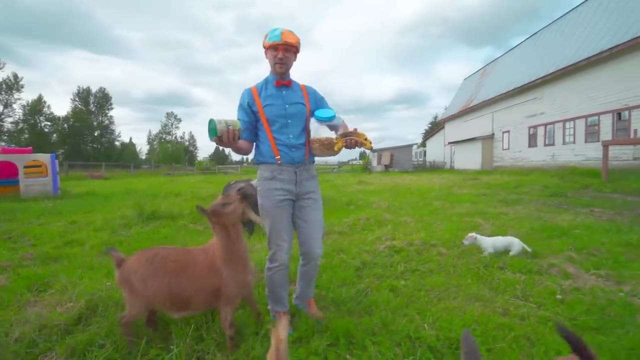 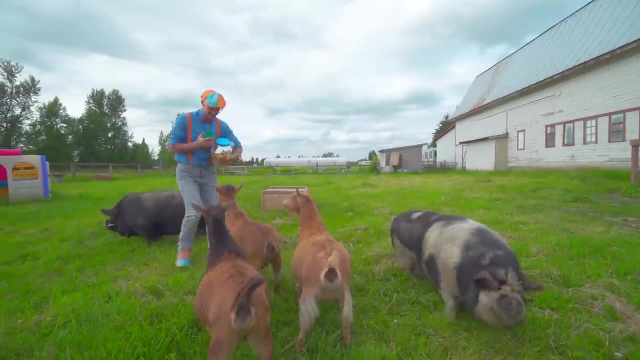 Yum, Hey, pigs. Another fun thing about this farm is they have farm pets too, just like these goats. Whoa, and there's some pigs back here. All right, hey down, All right. so let's give them some treats, all right. 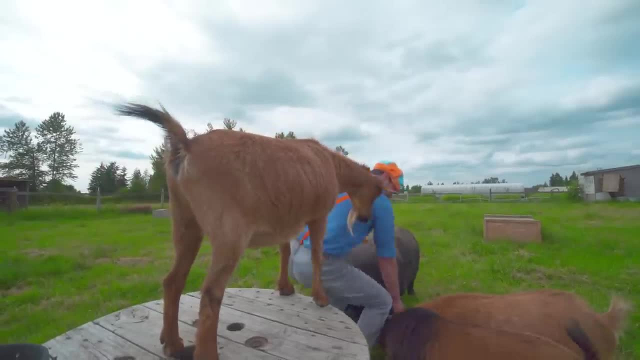 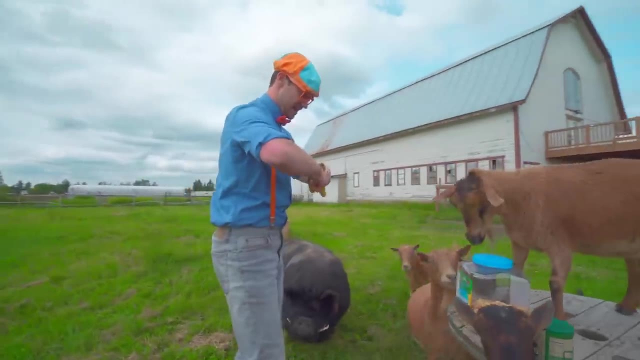 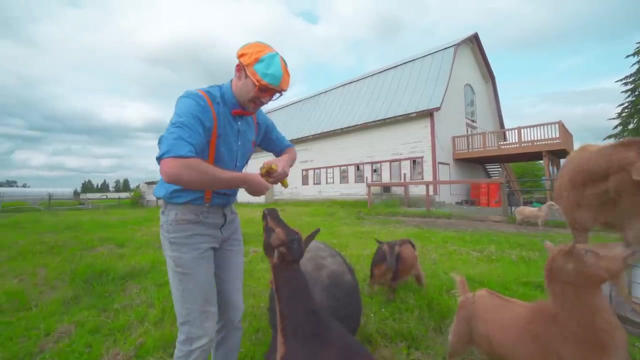 Let's see, oops, sorry, Here's. oh, whoopsies. Okay, let's set some of this stuff down. I'm gonna set that down, All right. who wants some banana? Oh yum, All right. would you like some banana? 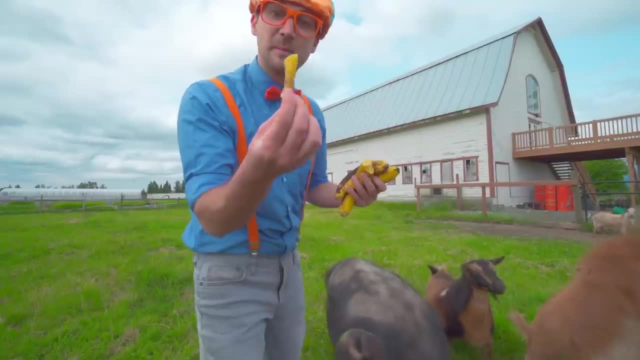 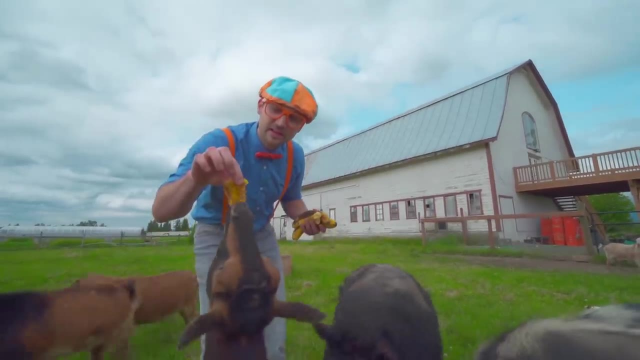 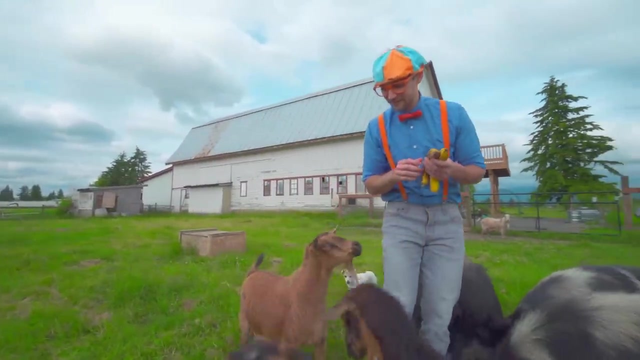 Oh, there you go. Ooh, you know the banana peel part that you and I don't like. They love it. Check it out. You want it? Yum. Ooh, Would you like some banana Yum? Enjoy. 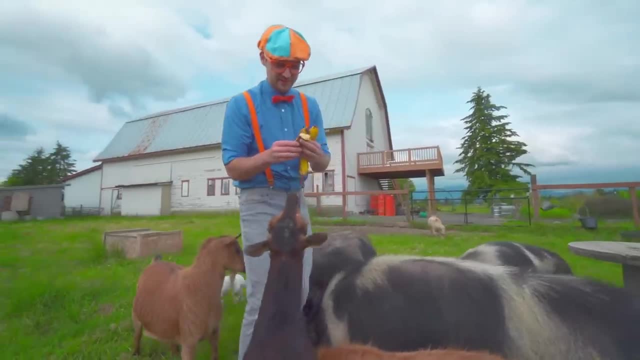 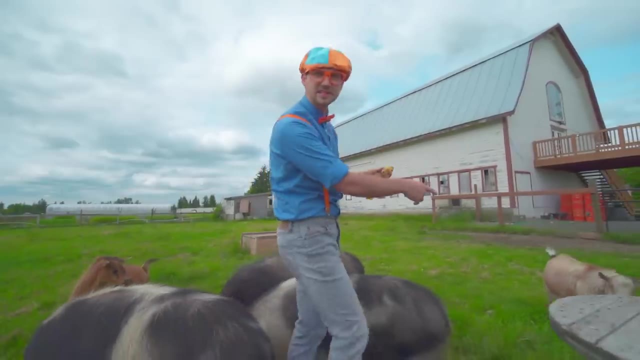 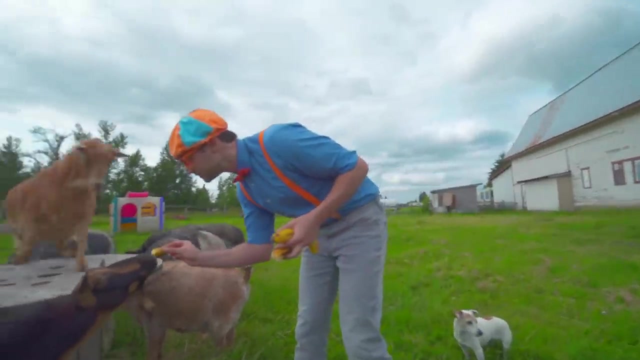 Whoo, Would you like some banana? Okay, there you go. Okay, hey, this one hasn't got any. Hey, would you like a treat? Hey, oh, hey, would you like a treat? Ooh, oh, oh, oh, hey, down. 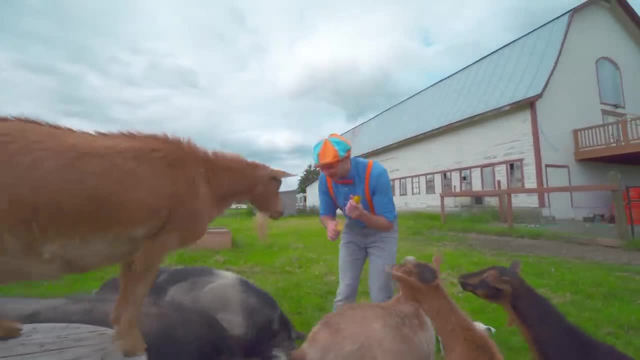 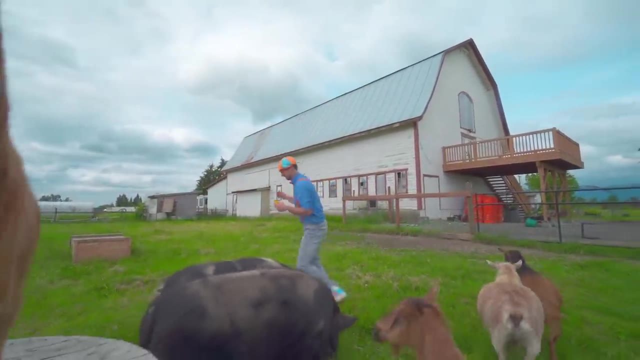 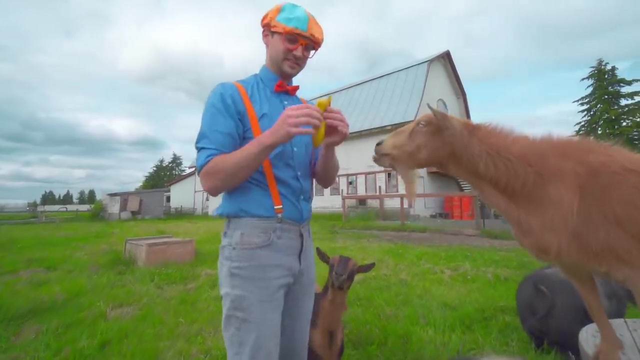 Good down, There you go, Hey pig. Hey pig, There you go. Oh, all right. Would you like some banana? There you go, All right. Whoo, there's some peel for ya, Hey down. 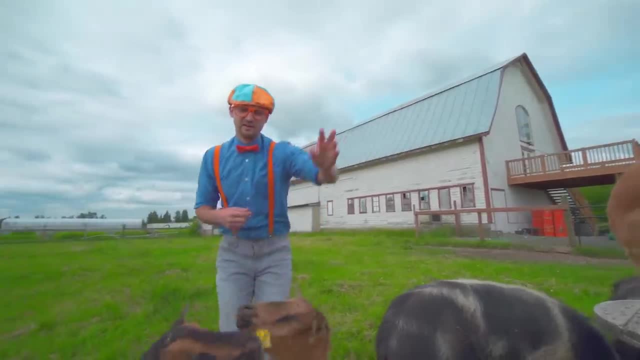 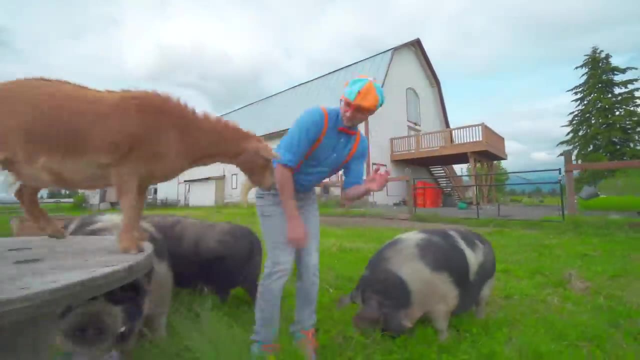 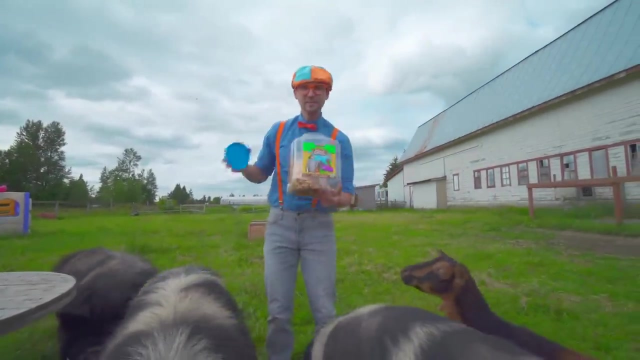 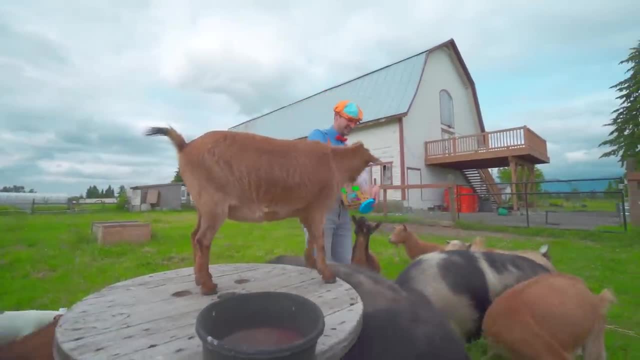 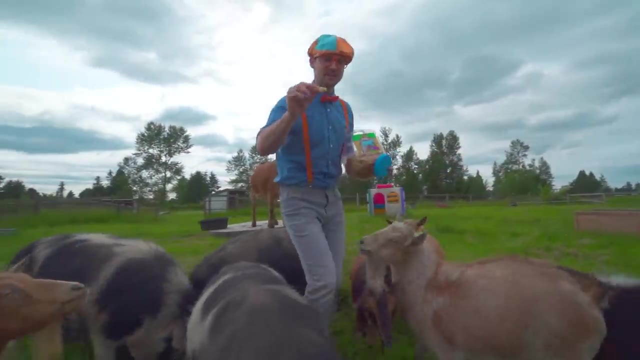 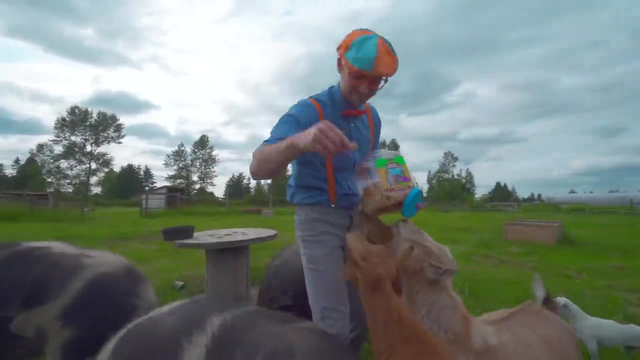 Here, want some crackers. Whee, Here you go, Here you go Here. see, It's an animal, But it's a cracker. There you go, Hey, there you go. Here you go, Here you go, Oh, there you go. 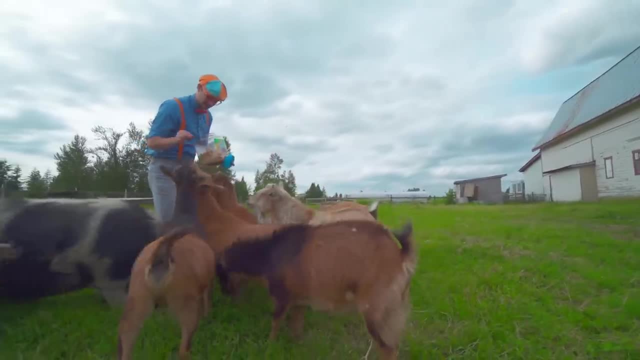 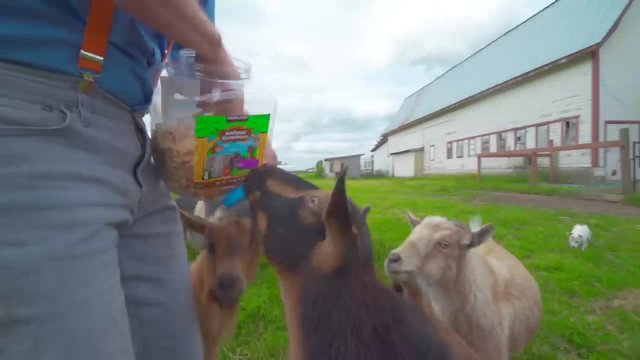 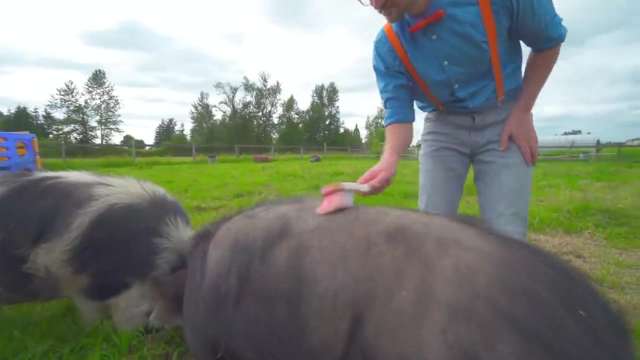 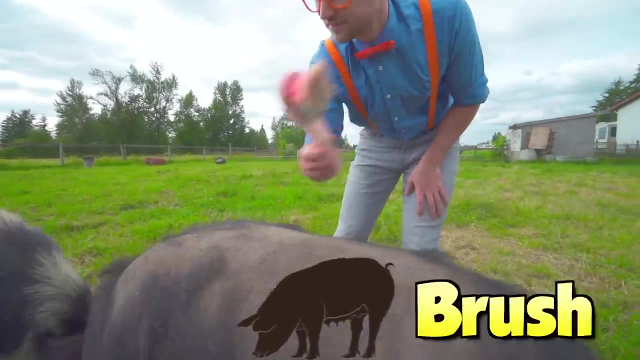 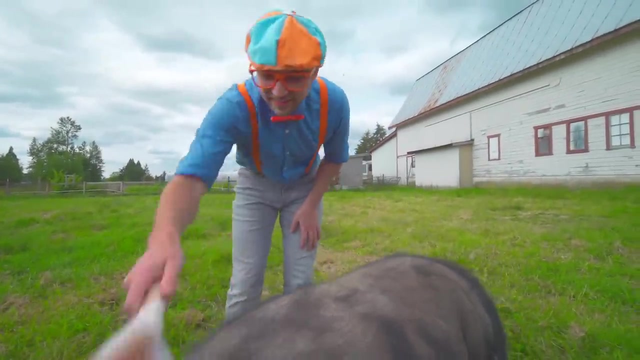 Hey, down, go down. Do you see what I'm doing? I'm using this brush to give him a nice back scratch. There you go. Hey, does that feel good? Yeah, have you ever gotten a back massage or a back scratch? 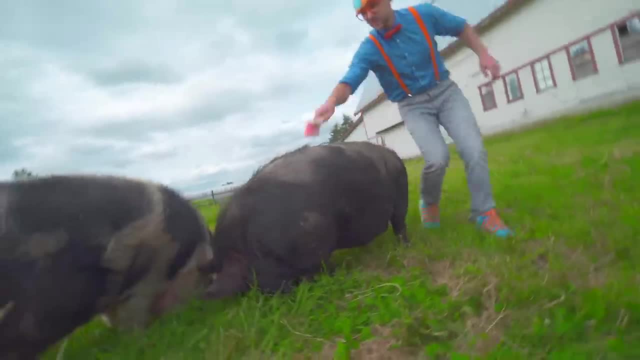 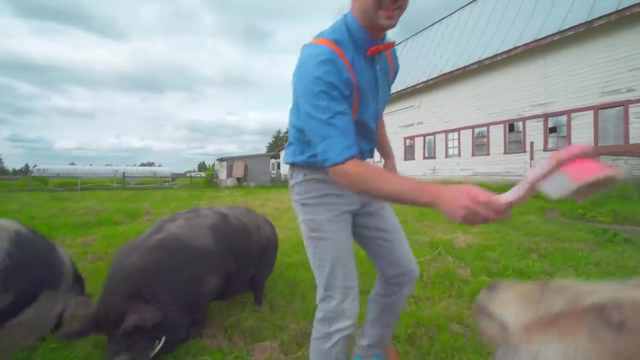 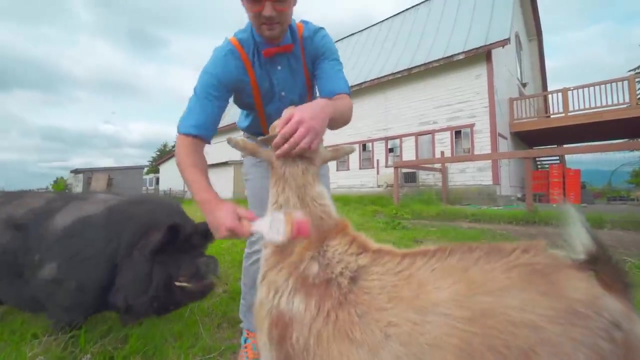 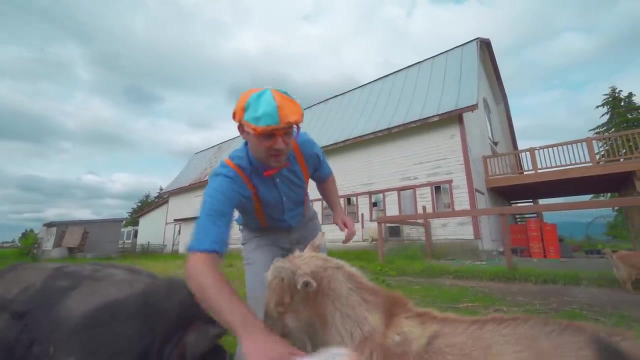 Yeah, this probably feels just like that Right pig The skin. Hey, would you like to get brushed? Yeah, there you go, There you go. Yeah, does that feel good? It's kind of like a bath, but without water, and it doesn't clean you. 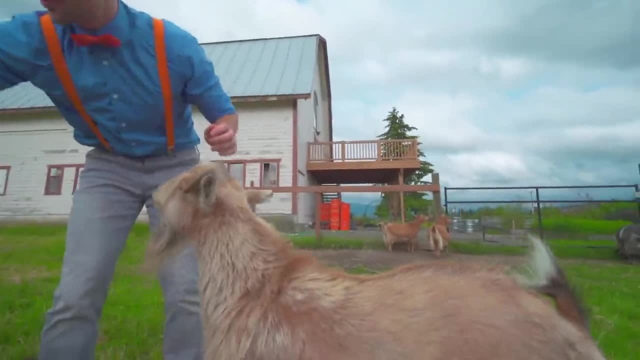 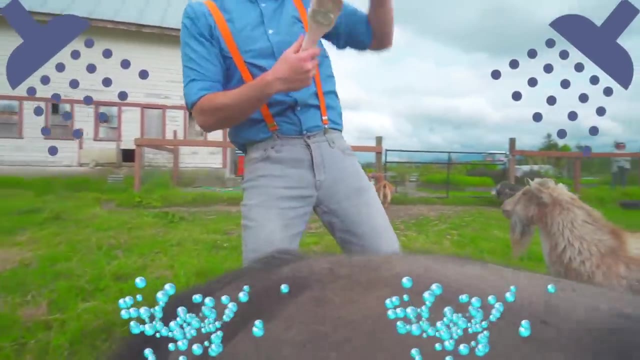 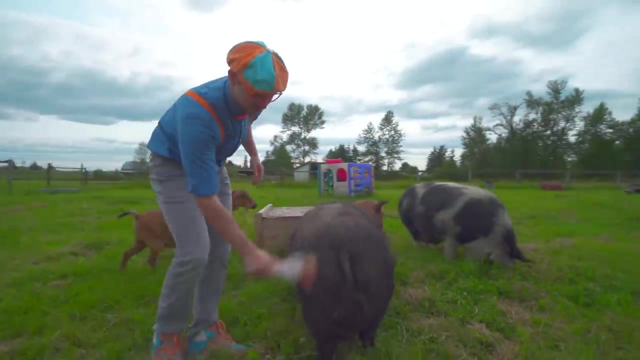 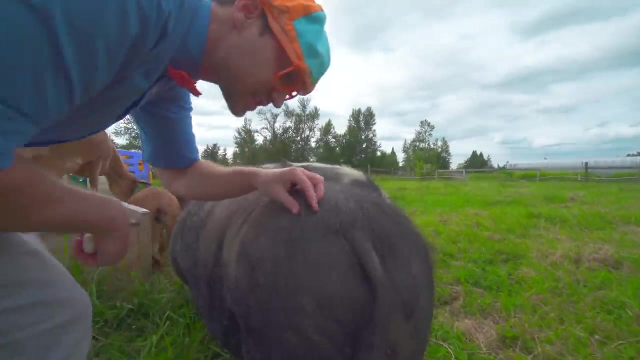 It just feels really good. I like taking baths and showers nice and clean and rubbing a brush on my skin. Okay, there you go, Let's get you right there. Come check out this pig's hair. Whoa, it's really coarse and really thick. 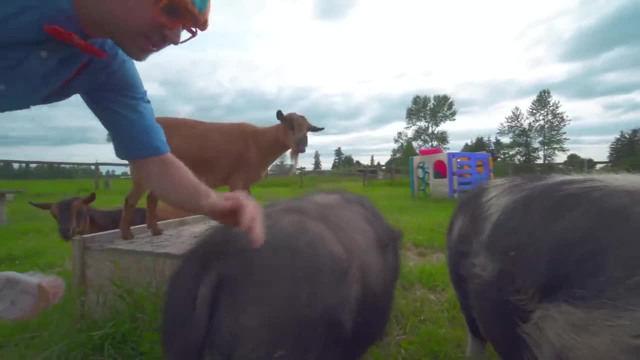 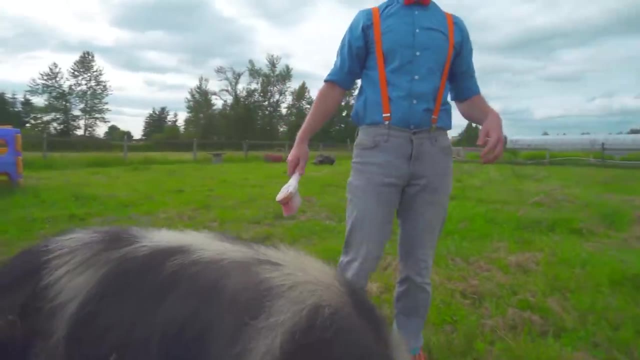 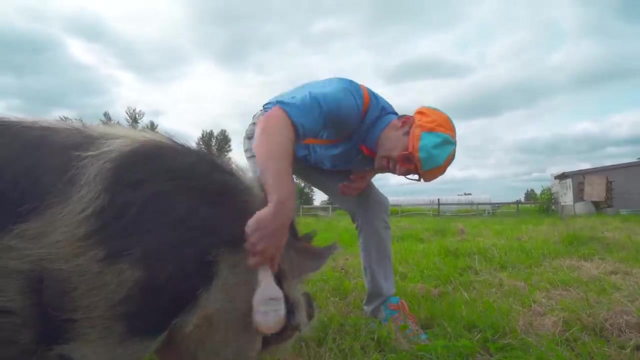 Wow, It's really thick. Oh hello, Hey pig, There you go. Oh yeah, does that feel good? Oh, I bet, There you go. Yeah, See, I'm brushing this pig. This pig is really big. 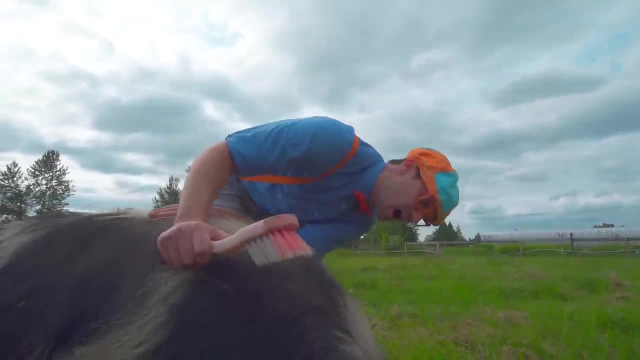 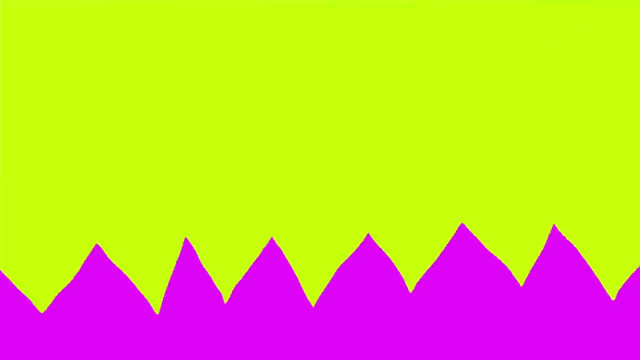 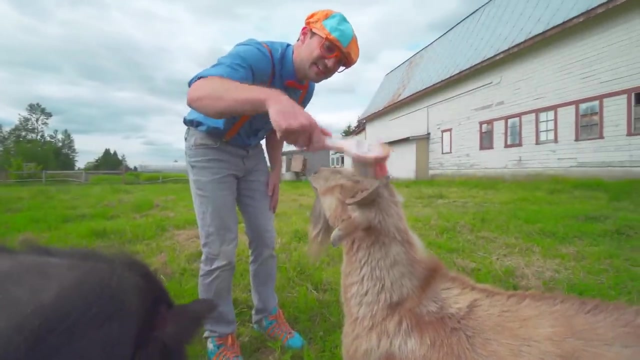 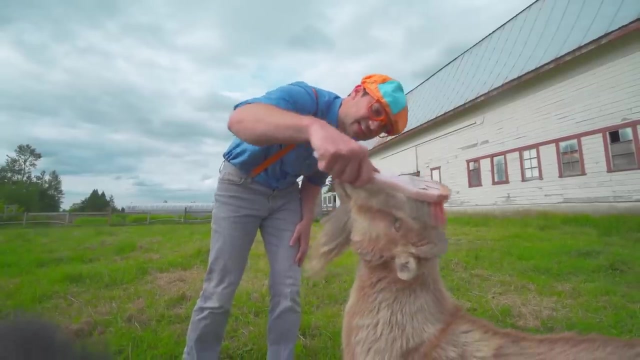 Whoa, Can I give you a hug? Ha ha, Does that feel good? Yeah, that feels real good. You like your horns brushed? huh, Yeah, there you go. You're a nice guy, Whoa, And do you see his eyes? 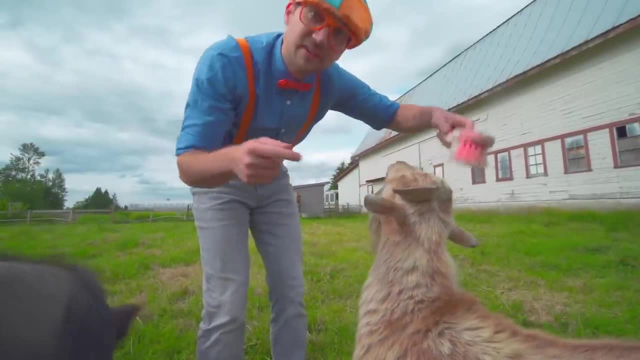 Look, Look at his eyes, Come here. Do you see the black pupil? Yeah, that black part is called the pupil, And it's sideways. So then, from there, the goat can see all around itself. Wow, There you go, buddy. 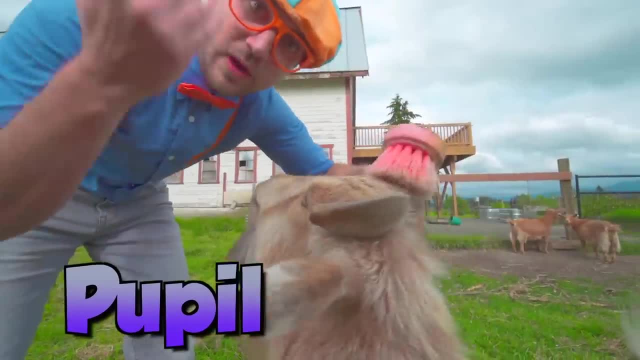 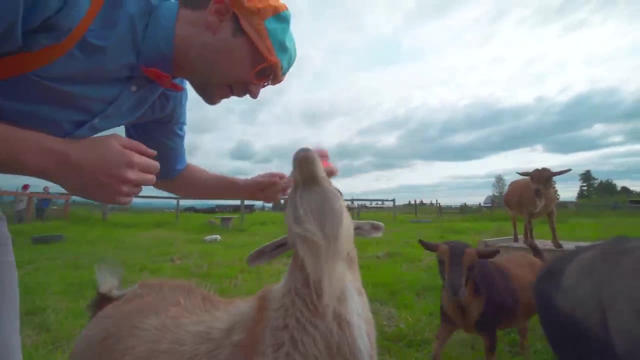 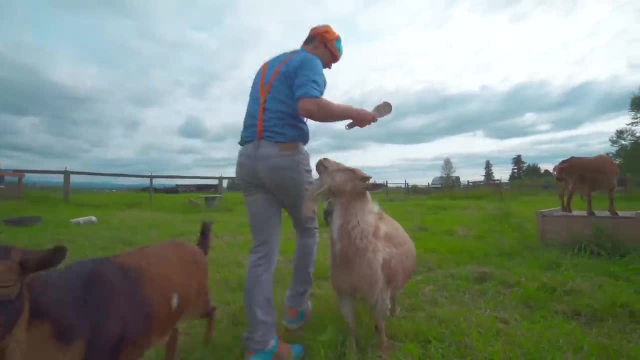 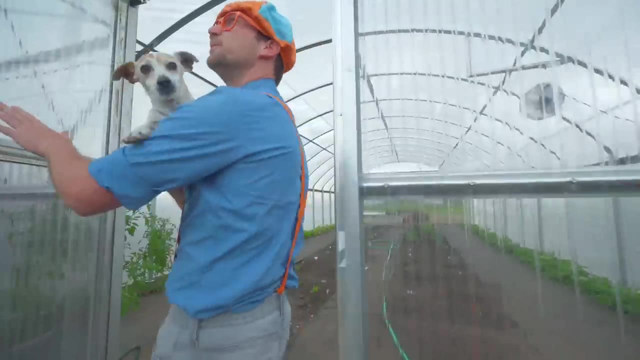 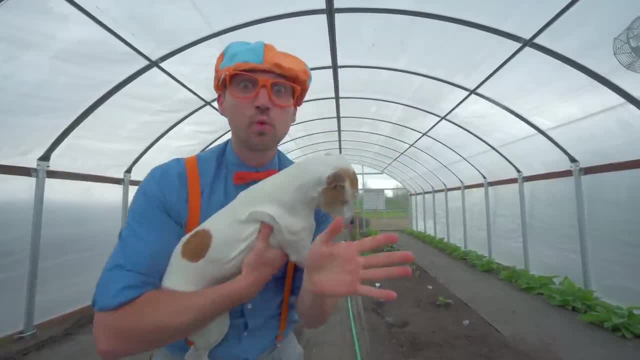 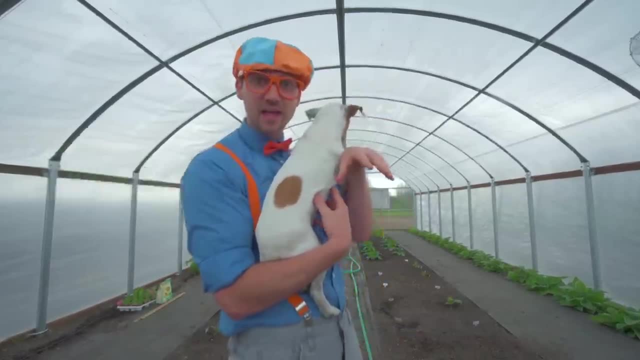 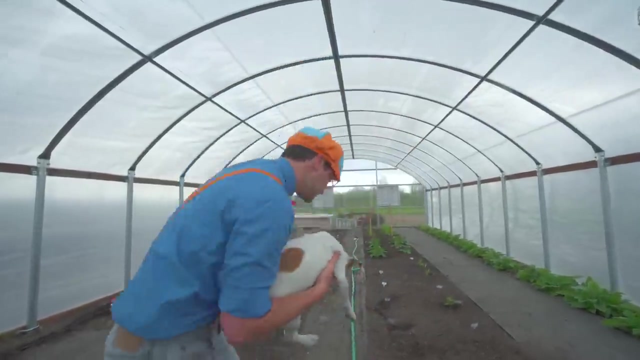 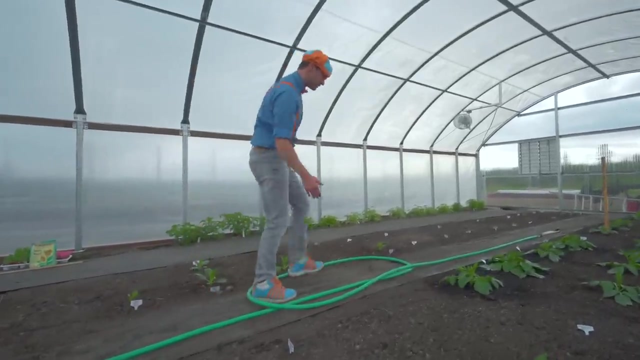 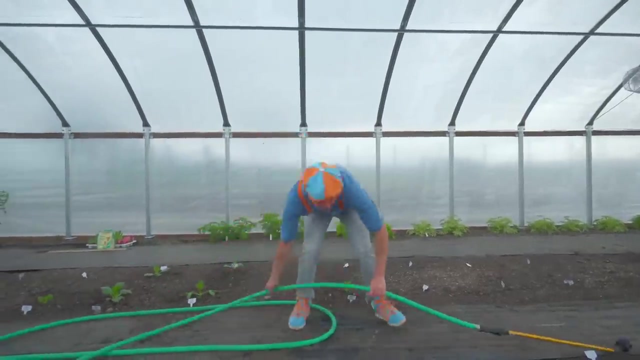 Growing rooms are kind of like greenhouses. They keep a little bit more heat inside than outside. Right, Sheila? All right, let's go explore Here. it is Cool. Ooh, Look at what it is: It's a green hose. Whoa, Oh, hey, Look at what's on the end of. 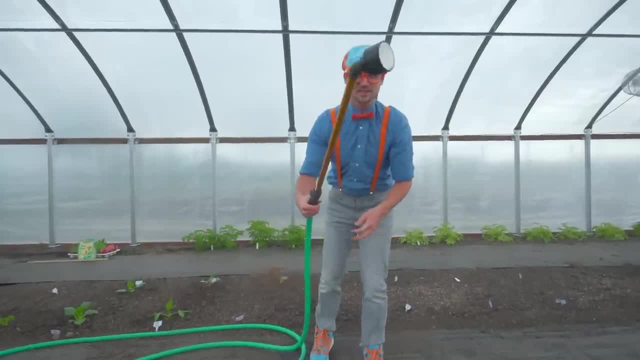 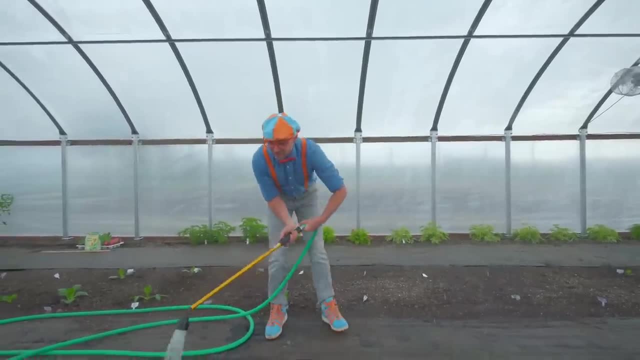 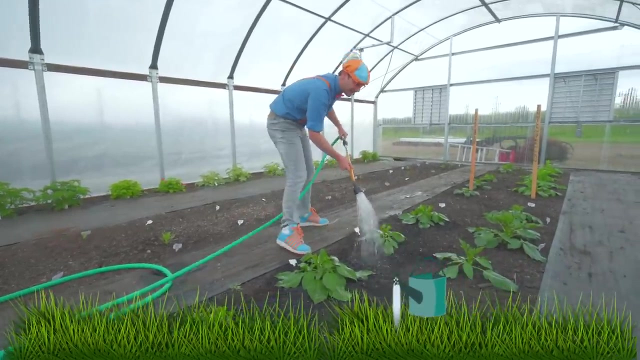 the hose. Oh, it's a watering spigot. What does it do? Whoa, It sprays water. Let's water the plants. There you go, There you go. Yeah, Plants love to drink water, just like you. 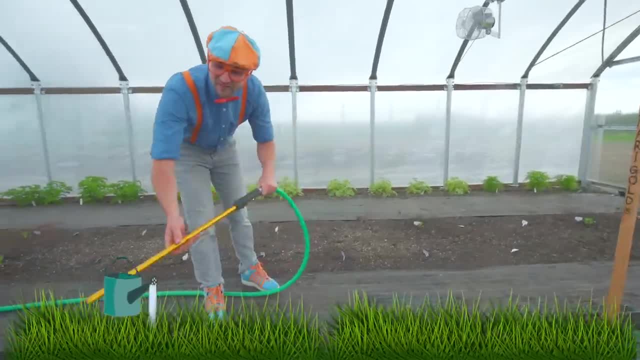 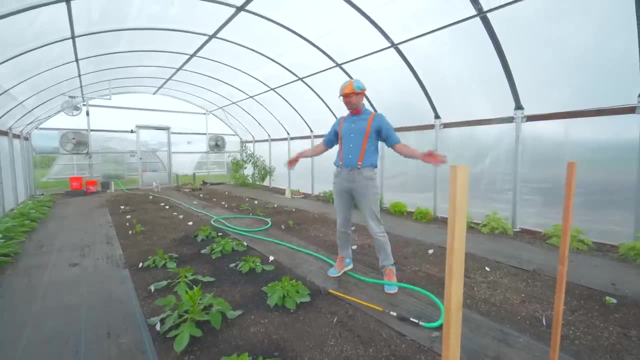 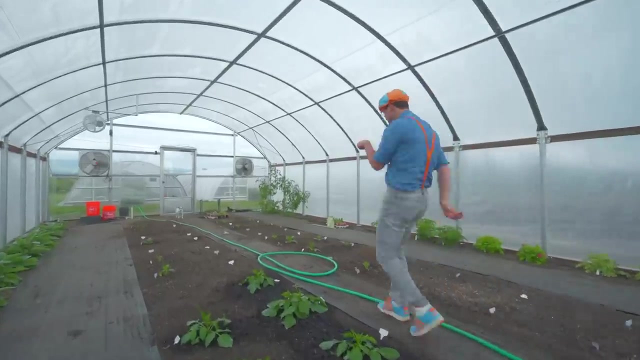 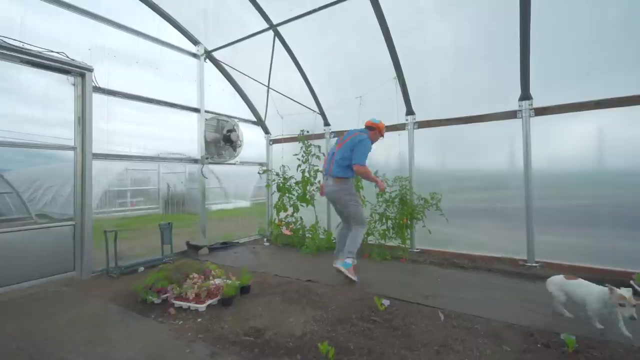 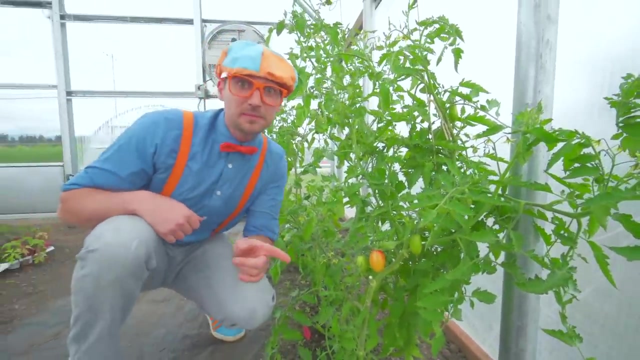 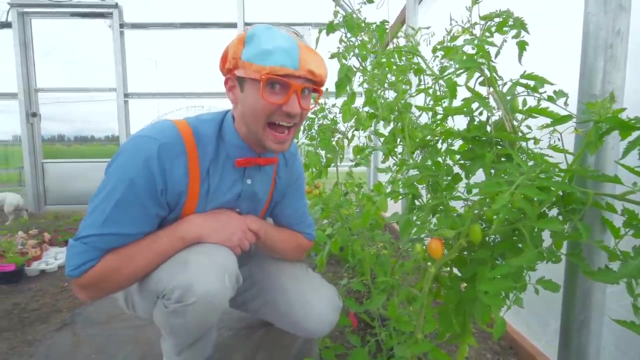 and I do All right. Wow, This is so much fun growing plants, because I love to eat the food afterwards. Speaking of food, look way down there, Whoa. Look, It's a plum tomato. Whoa, It looks so tasty, Shall we eat it? Whoa, Yum. 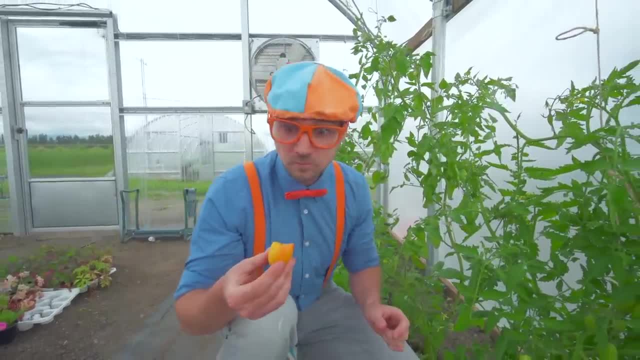 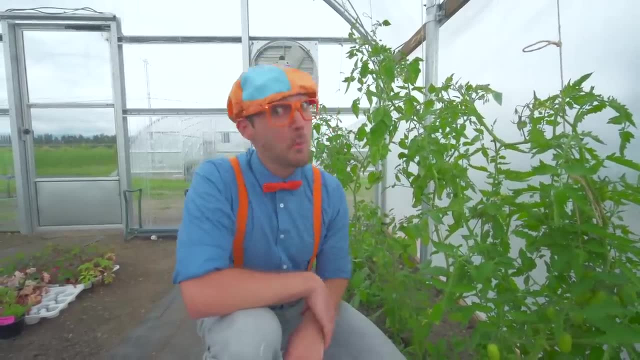 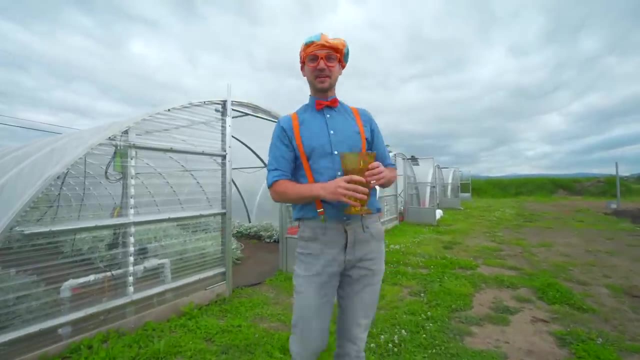 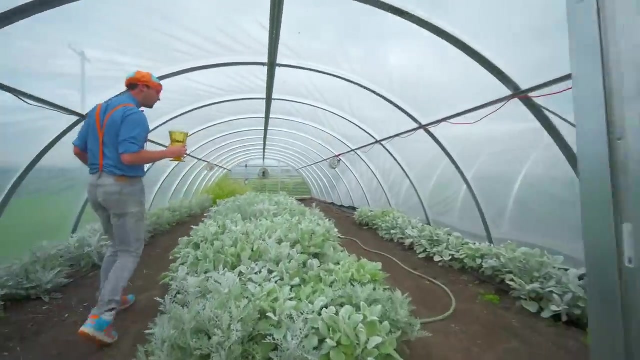 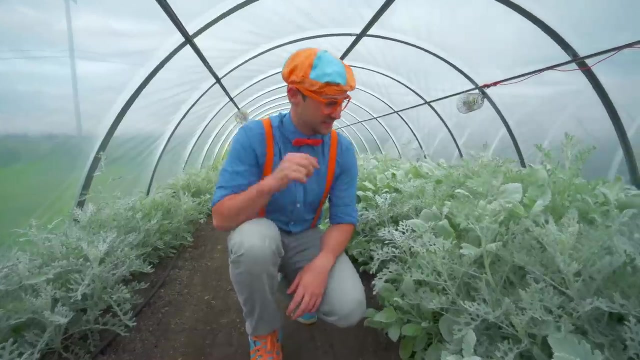 Mmm Ooh, Another fun thing to do at Laughing Goat Flower Farm is to make a bouquet. Come on, Whoa, Look in here Some more plants, All right. So these plants you don't eat, Yeah, These plants you make a bouquet. 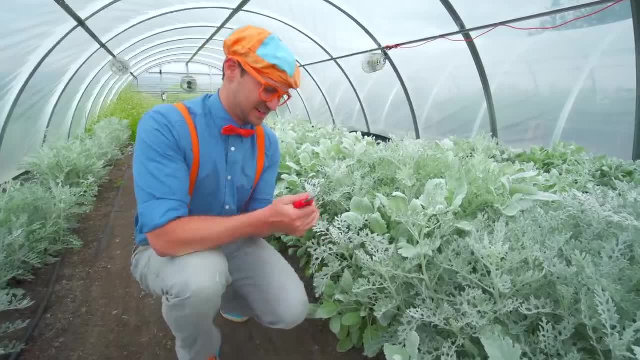 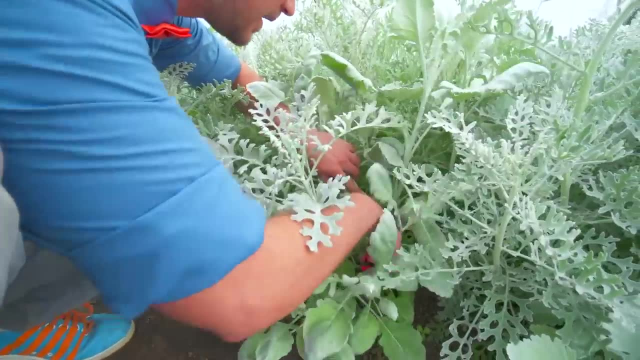 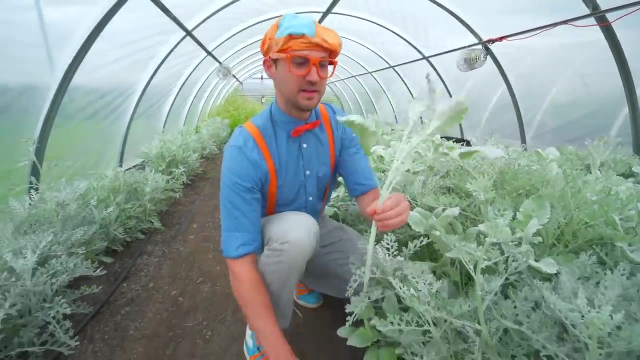 Yeah, These plants, you make a bouquet, Beautiful, beautiful bouquet with. All right, Here we go, Let's take our snips. All right, Where to go? How about right there? All right, Okay, Oh, that's real pretty. So how you? 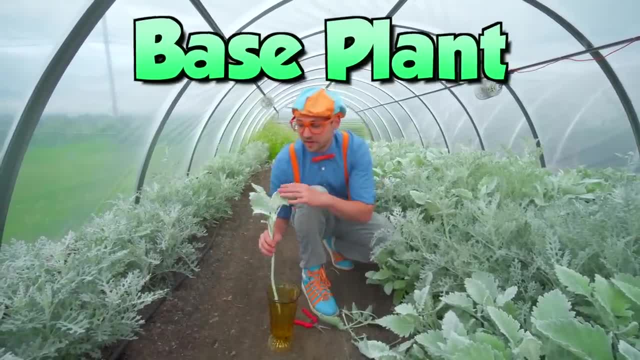 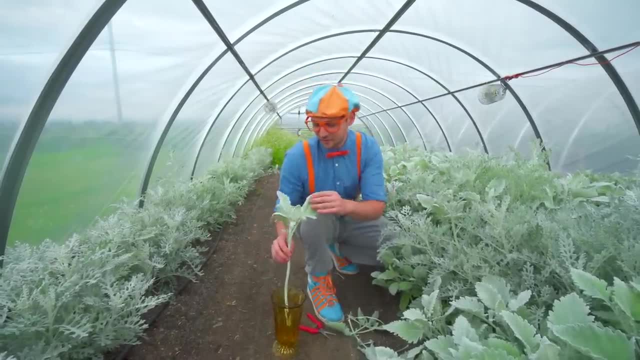 make a bouquet is you start with a base flower like this. Well, actually, you start with a base plant and then you add the base plant, And then you add the beautiful colorful flowers, But this plant right here, yeah. 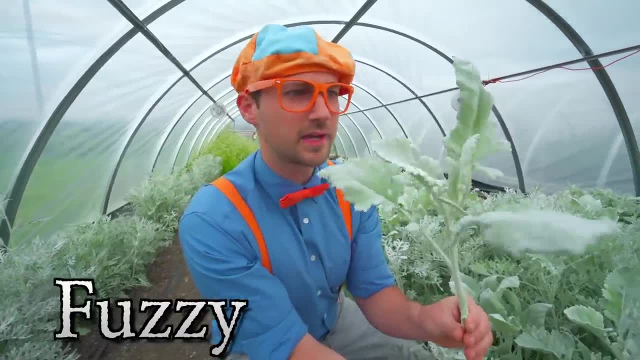 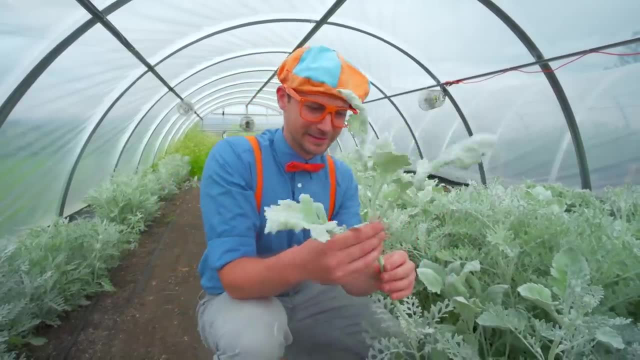 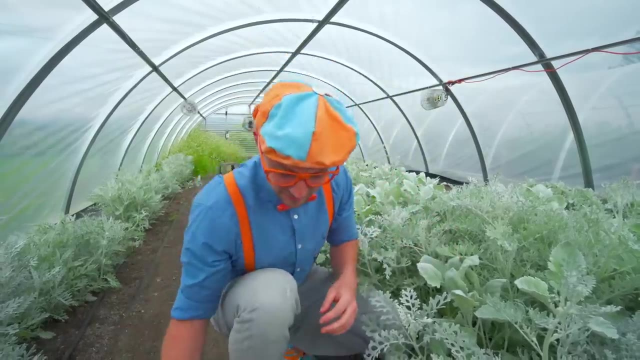 it's fuzzy And it kind of looks like the color white. Yeah, Normally plants are the color green. Well, sometimes It really depends on the plant, But this one is pretty white looking. All right, Let's cut some more, shall we? 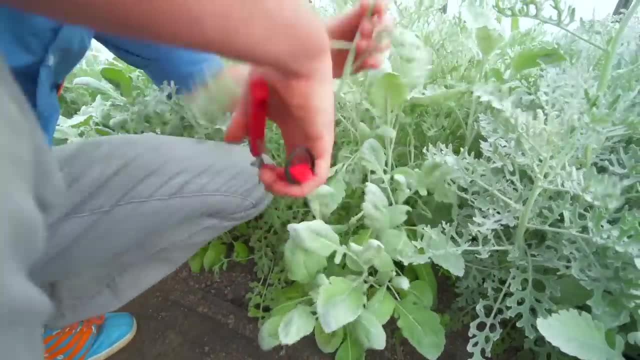 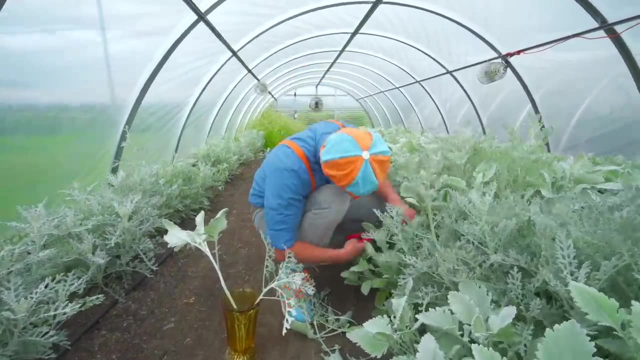 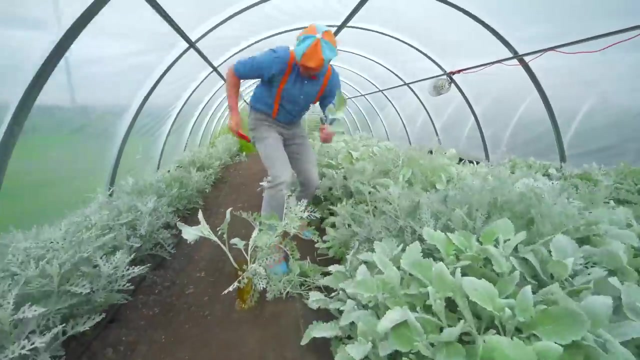 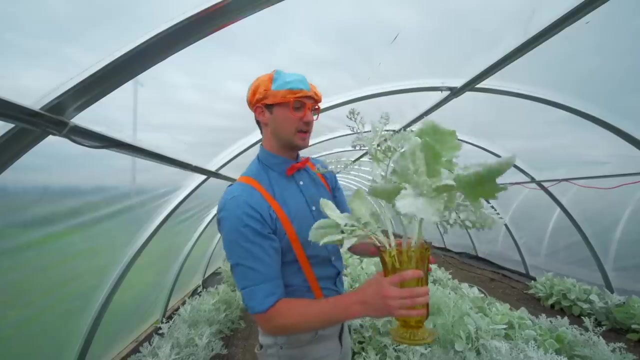 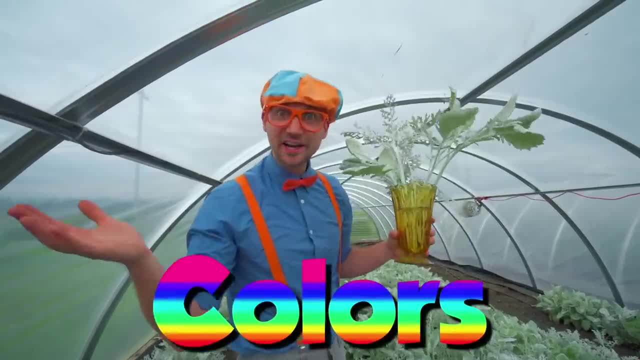 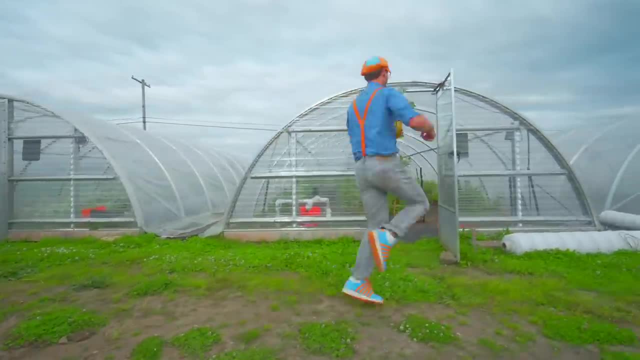 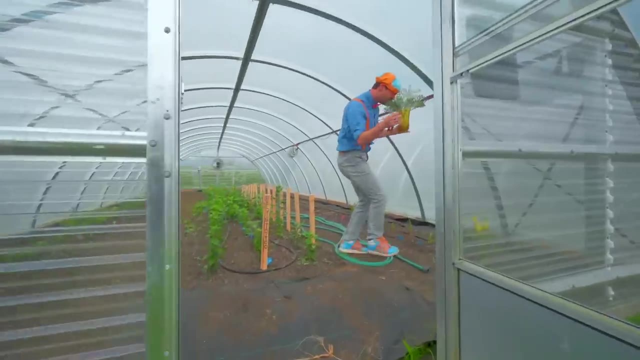 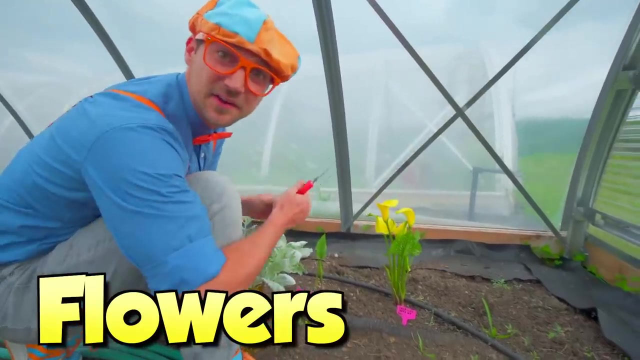 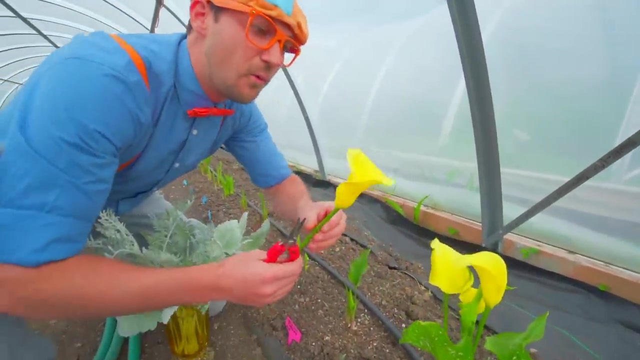 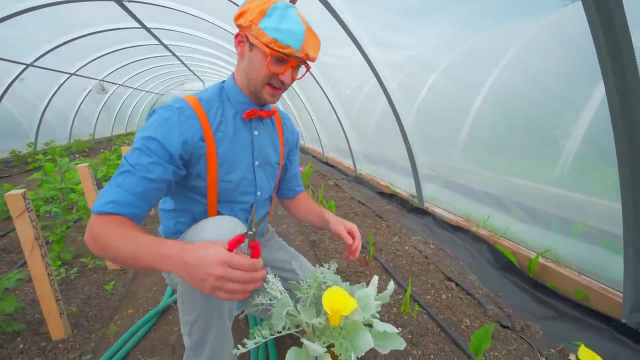 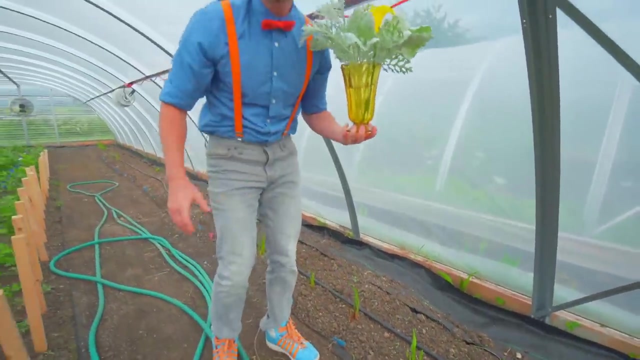 base. We need some color. Let's go: Oh, look at these colorful flowers. yeah, they're the color yellow. these will look beautiful in the bouquet. all right. whoa, so interesting looking. okay, let's put that right there. all right, one will do. all righty, let's find some more flowers. 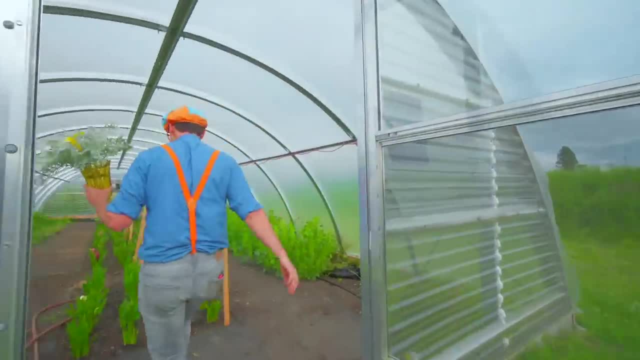 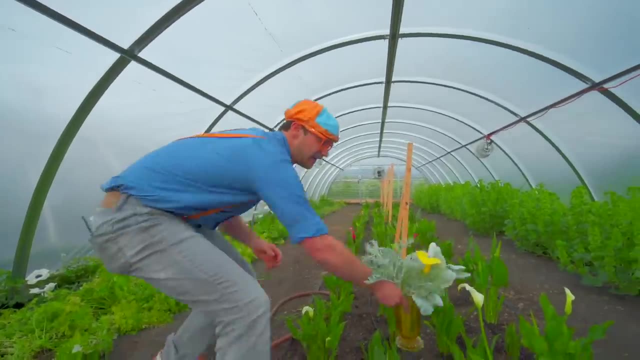 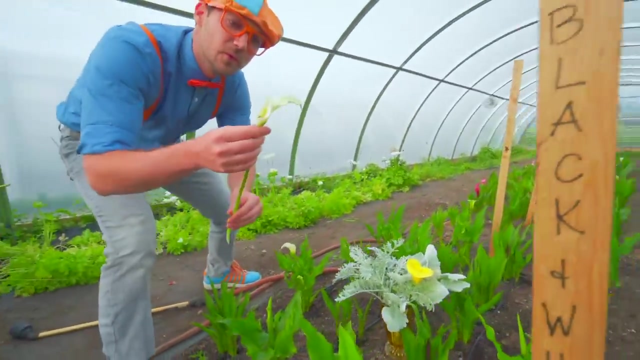 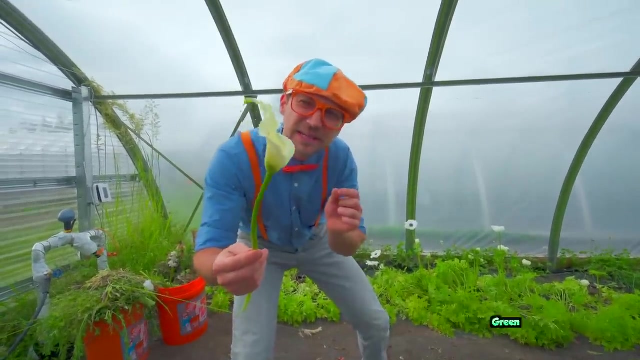 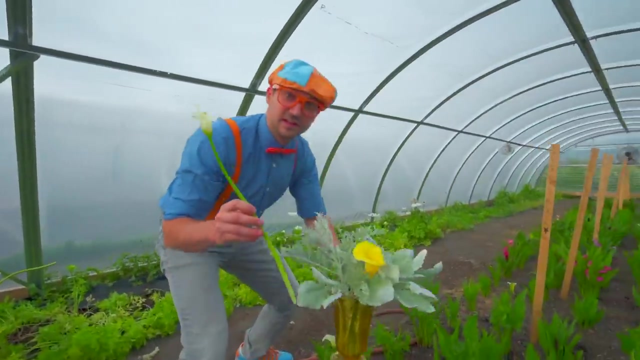 Oh, and more flowers. perfect, just what we're after. all right, look at this one. huh, all right, pull it up. whoo, it's kinda white. yeah, it also has a little bit of green and a little bit of yellow. yeah, and it makes that color. all right, let's put it. 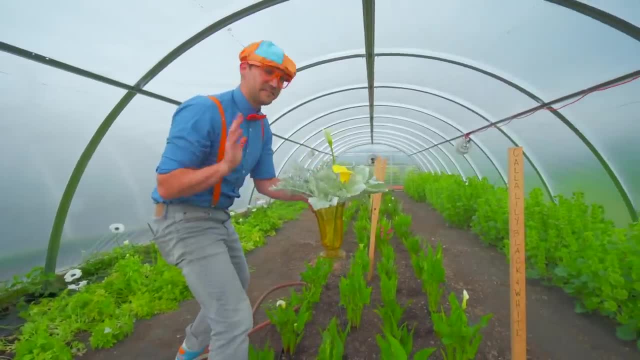 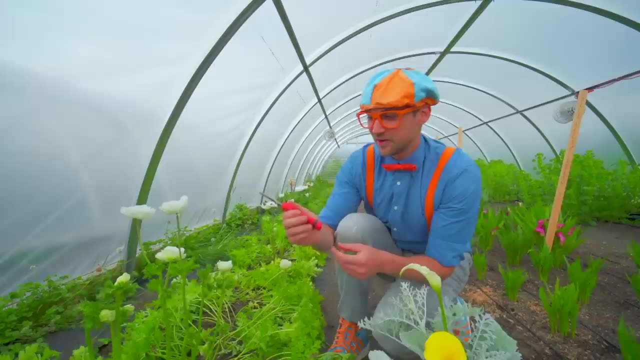 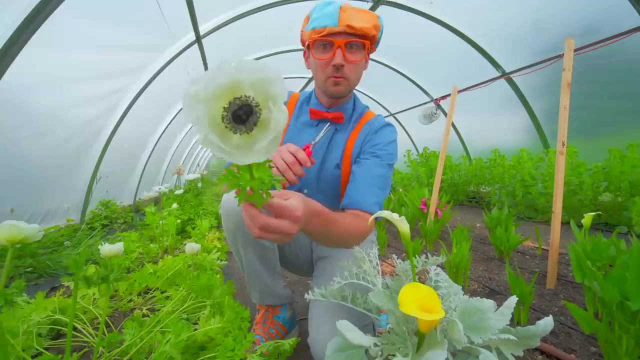 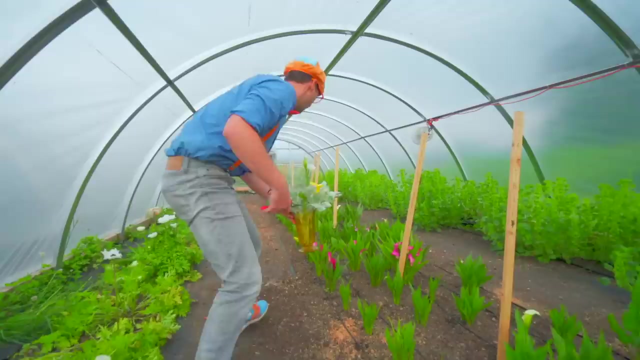 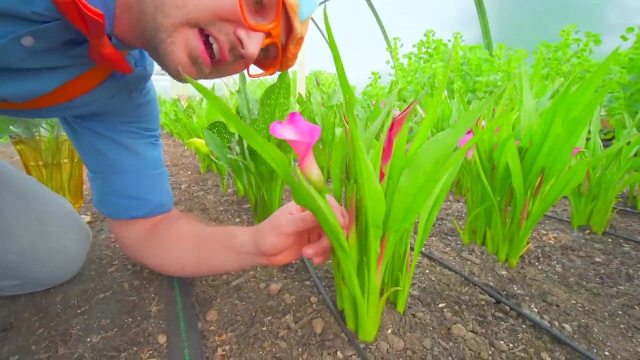 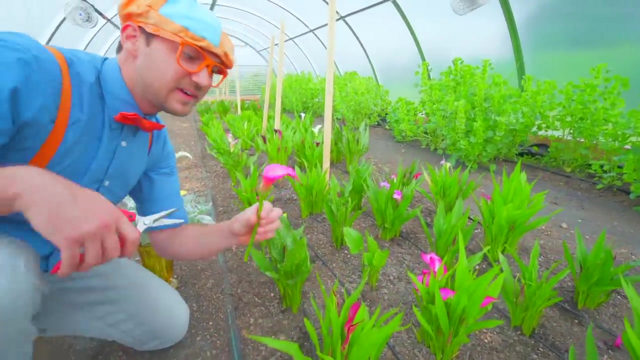 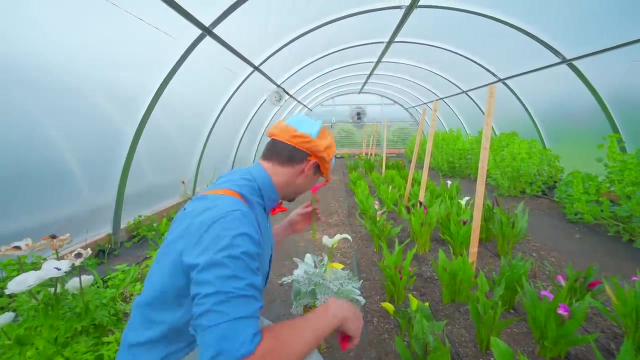 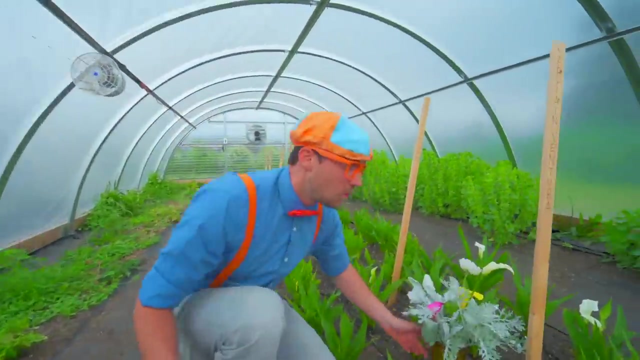 right there, yep, perfect. oh, look, take out our scissors. gotta be careful, okay, whoo, that one's the color white right there, whoa. look at this one. yeah, this color is the color pink. wow, so beautiful. ah, it smells so fresh. one more over here, whoa. 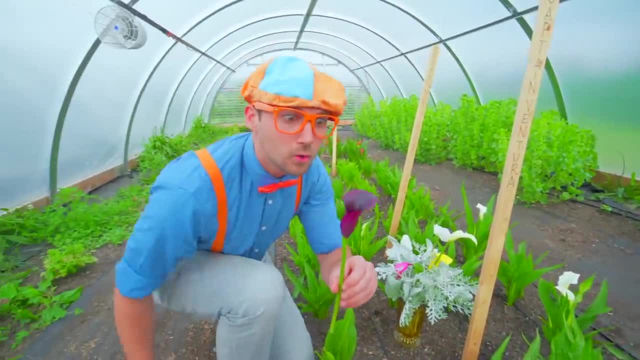 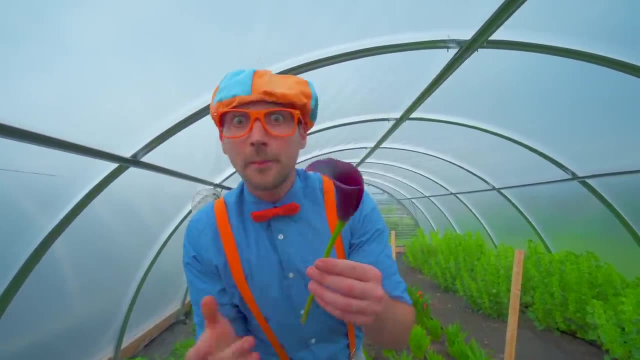 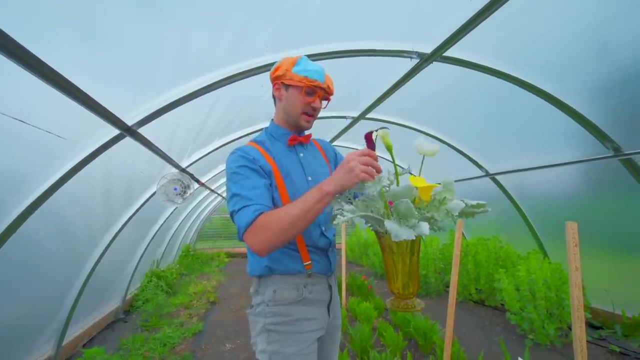 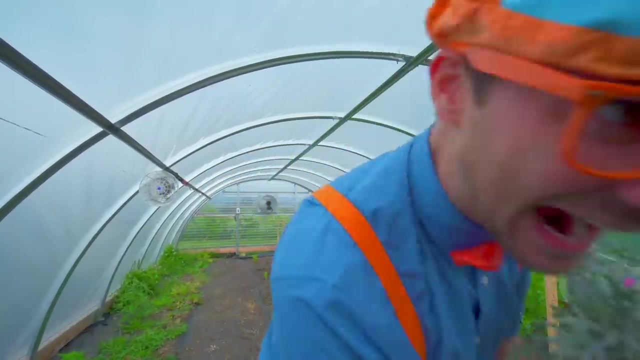 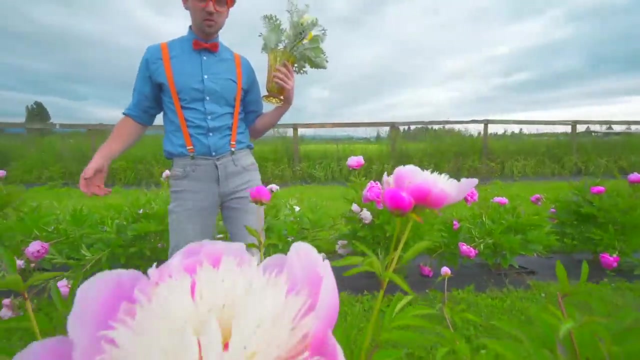 whoa, look at that color. whoa, whoa, it's a really deep, deep, dark purple. whoa, that will look beautiful in the bouquet. let's put it right there. all right, let's go find some more flowers. ah, whoa, here's some more beautiful flowers for a bouquet. all right, let's take our scissors. 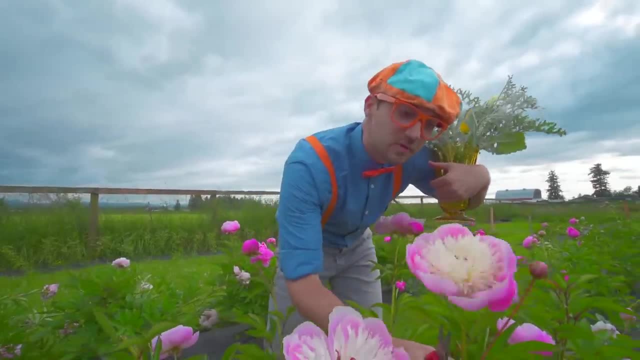 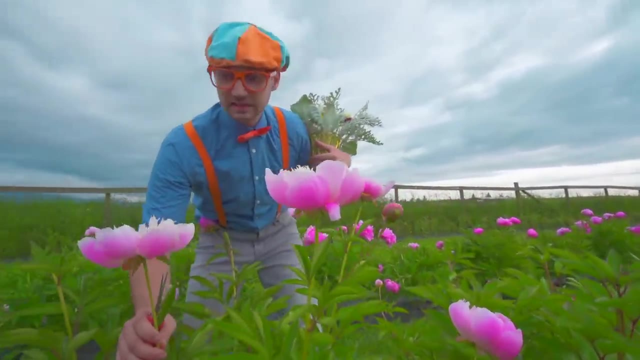 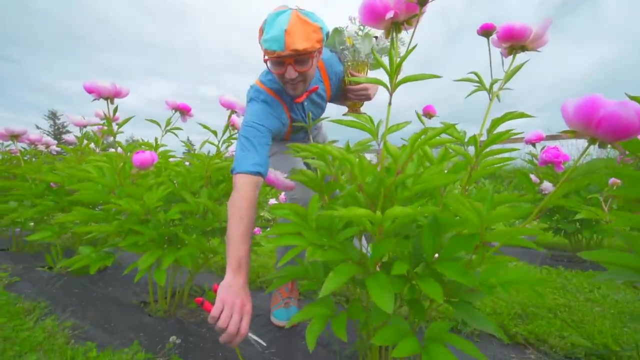 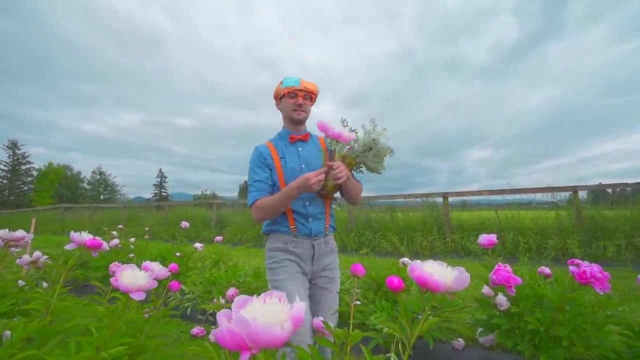 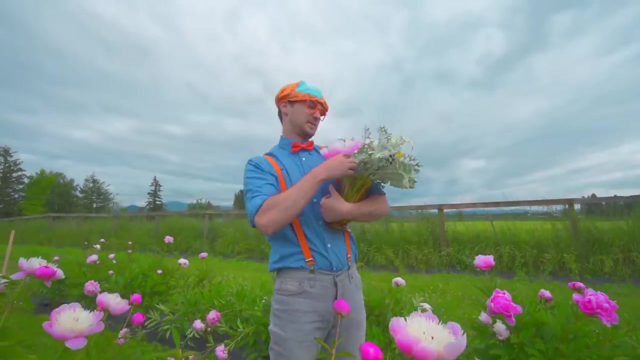 be very careful. this one looks perfect. actually, this one looks perfect. see the color. it's the color light pink. all right, oh, it fell. all right. all right, my snippers back there, all right. ah, so beautiful. all right, put it right there. whoa? look at it now. 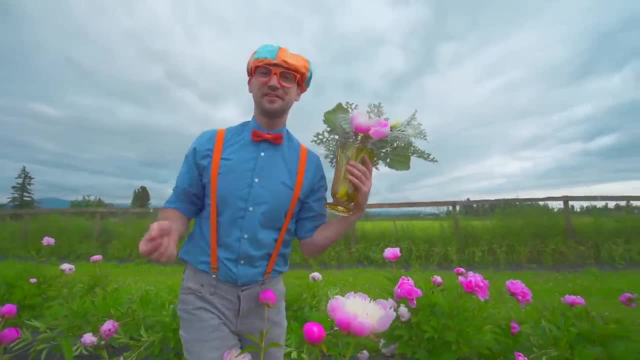 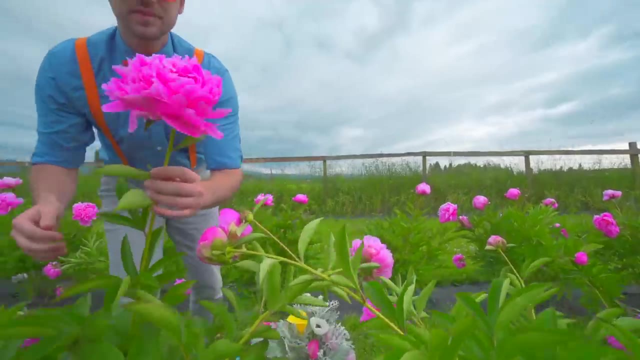 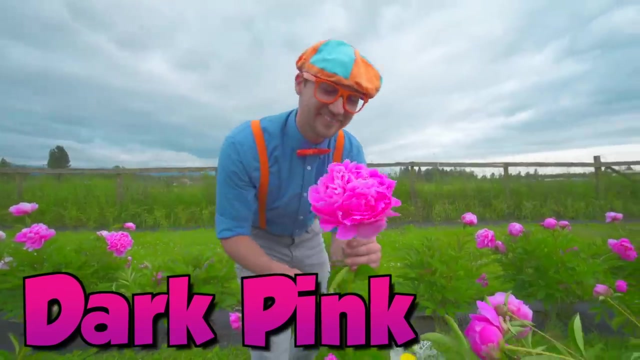 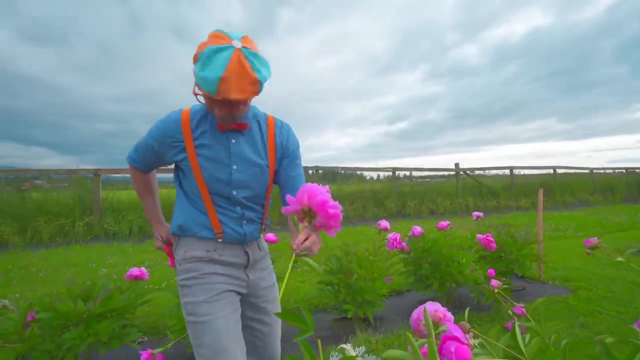 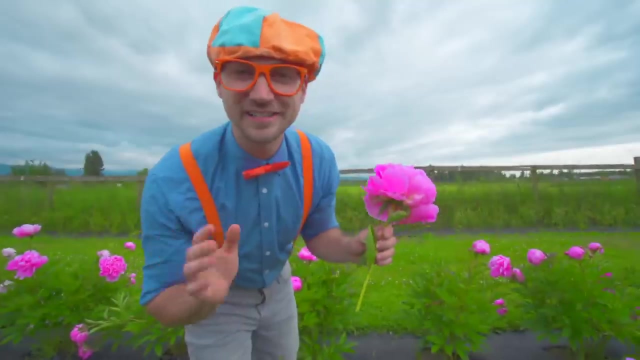 and it smells even more beautiful. okay, whoo, some more flowers. all right, this one looks ready and this one is dark pink. wow, all right, let's take the scissors, give it a snip, give it a smell. hmm, ah, so fresh. all right, here we go, let's put it right here. 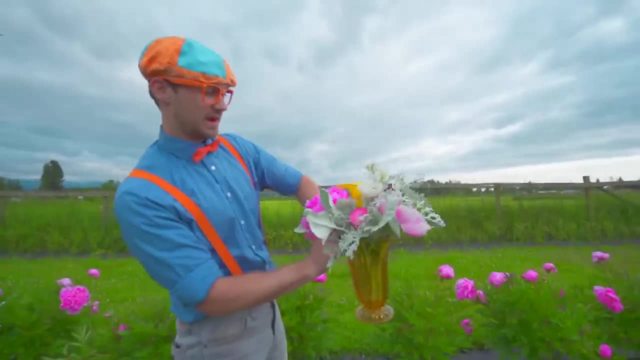 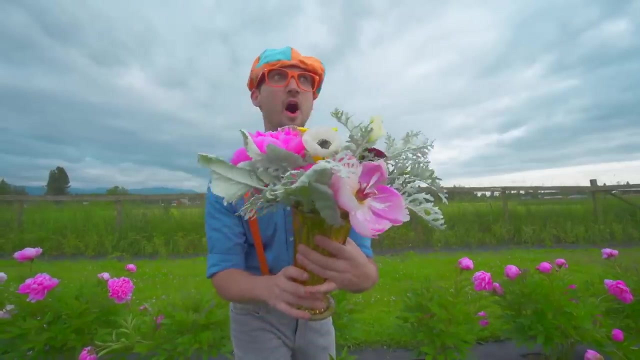 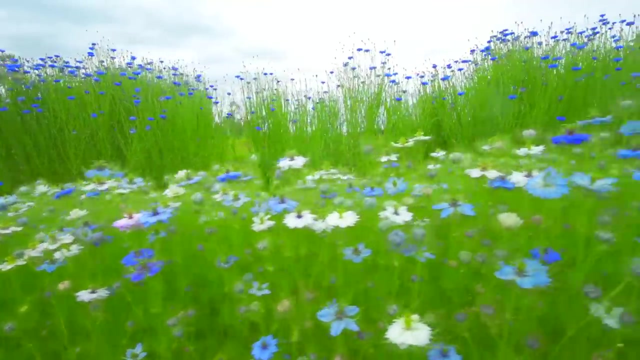 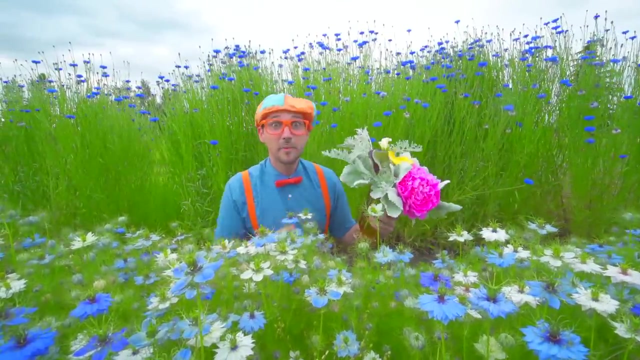 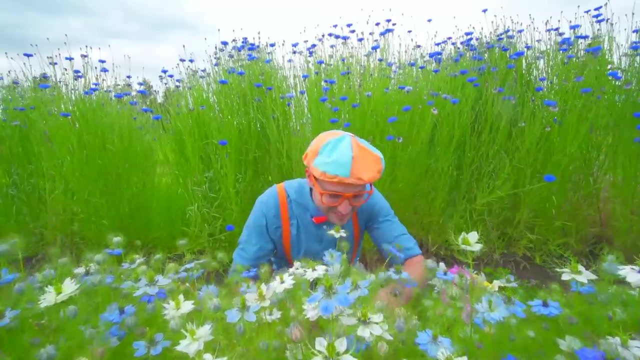 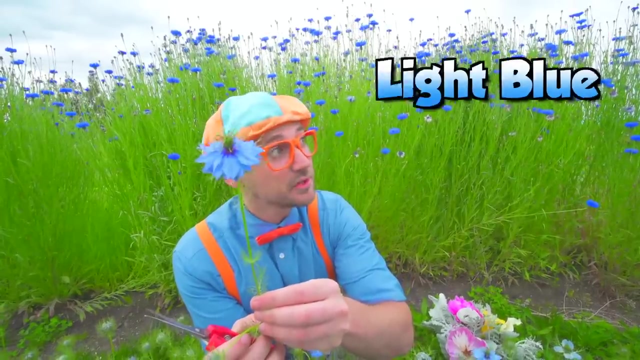 let's put it right there. whoa, that's a big flower. whoa, it's so colorful. oh, i see some more over there, more beautiful flowers for our bouquet. all right, let's cut some flowers too. all right, ooh, see this flower. this flower is the color light blue, wow, beautiful. all right, let's put it in here. 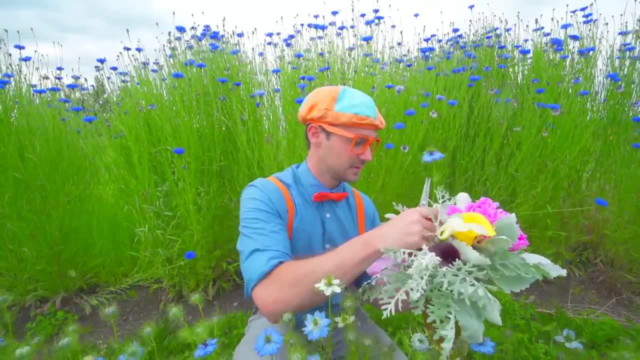 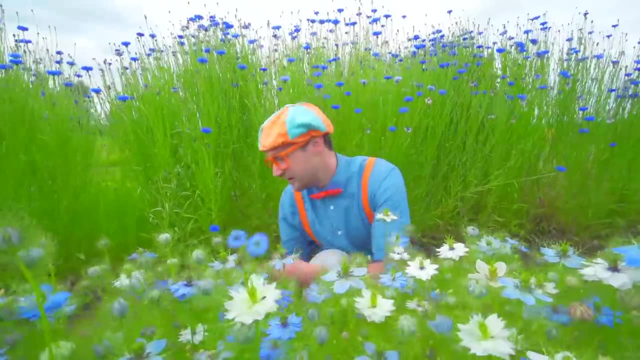 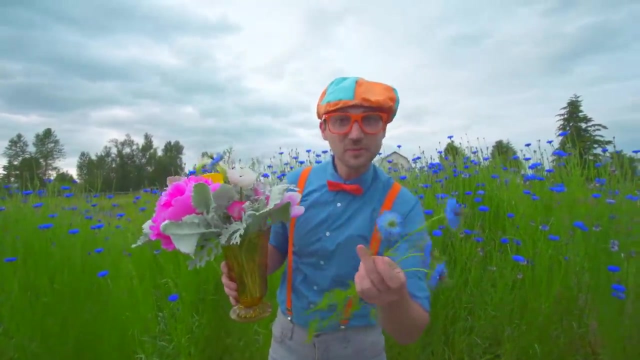 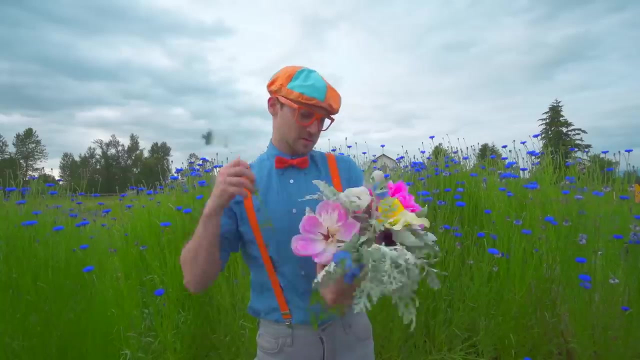 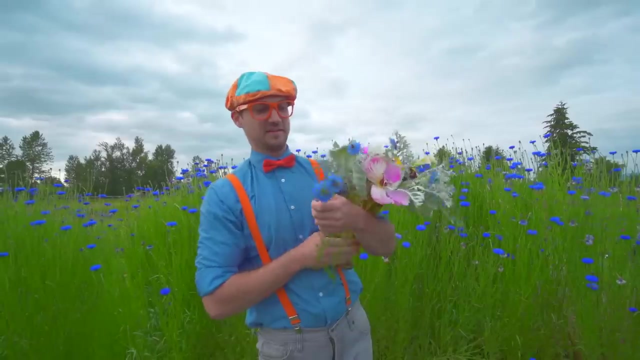 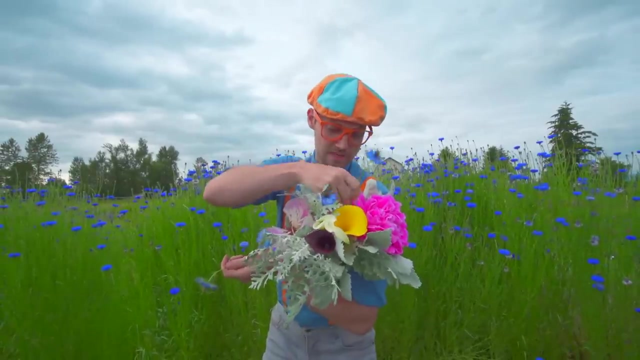 all right, perfect. all right, let's cut some more here. we go: all right, all right, all right. look, we have some more to place in here. uh, how about one right there? how about one right here? okay, and we have two more, one, two. let's put one right there, perfect. and let's put the last one right next to this big one. 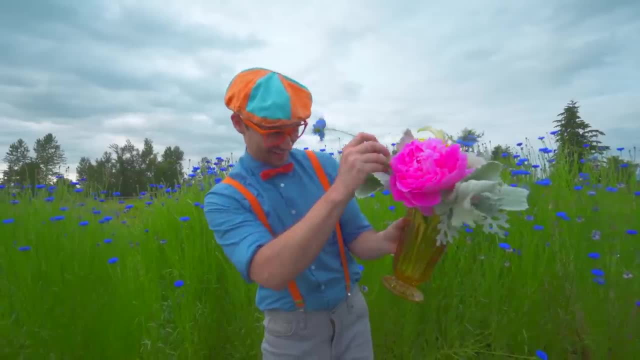 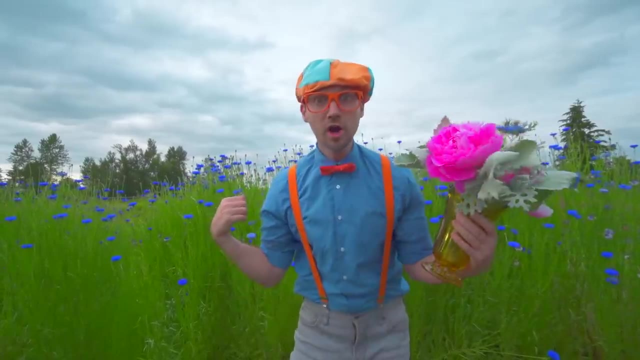 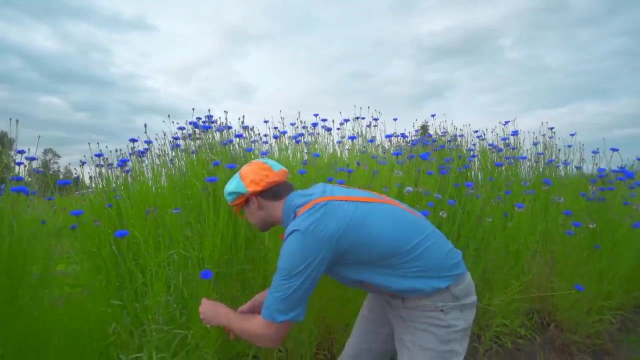 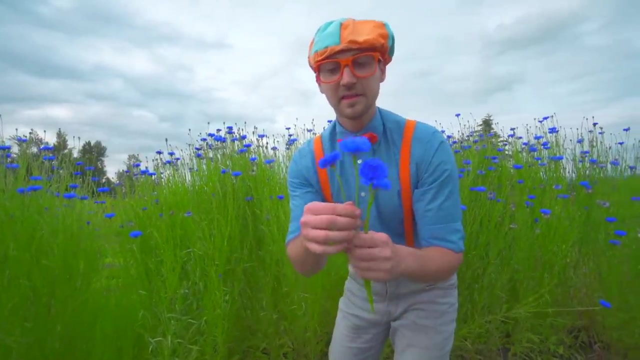 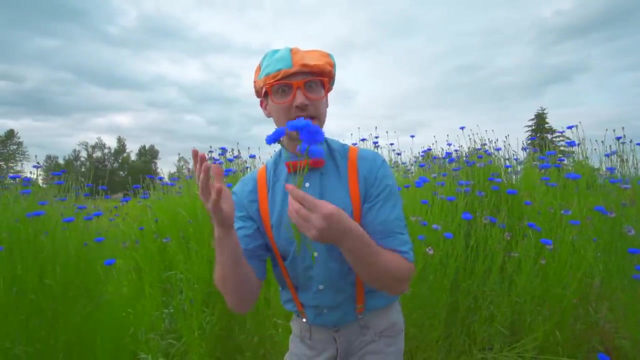 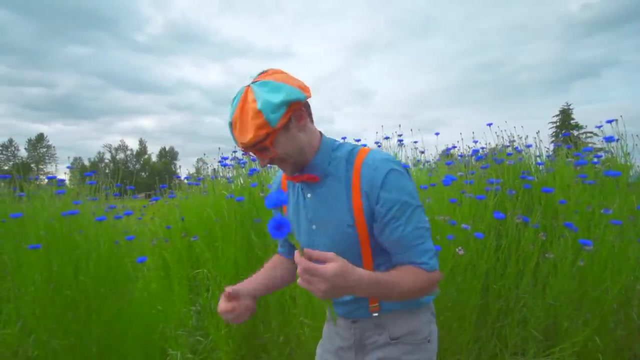 all right, there we go. perfect, so beautiful. oh, look more blue flowers. all right, let me snip some of these. huh, these are the color blue as well, but remember the last flower was a little bit darker than this one right here, but remember the last flowers, they were light blue. but these flowers are dark blue. let's put them in the bouquet. 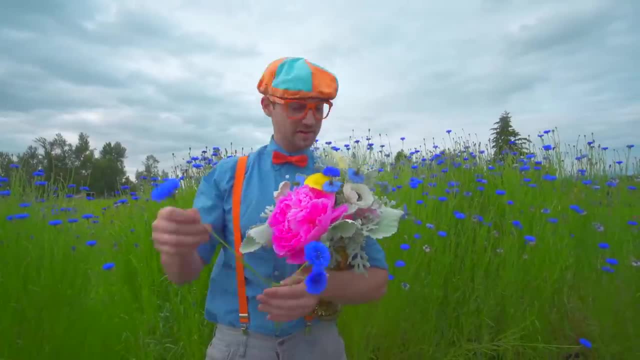 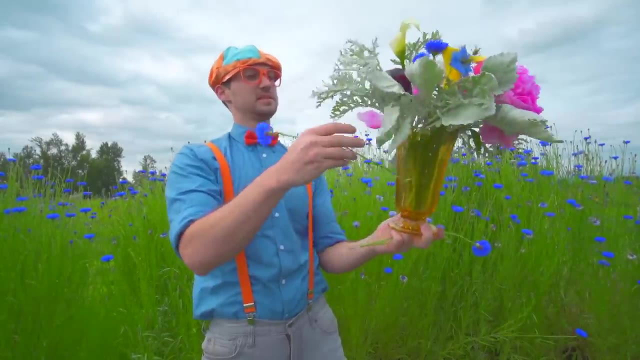 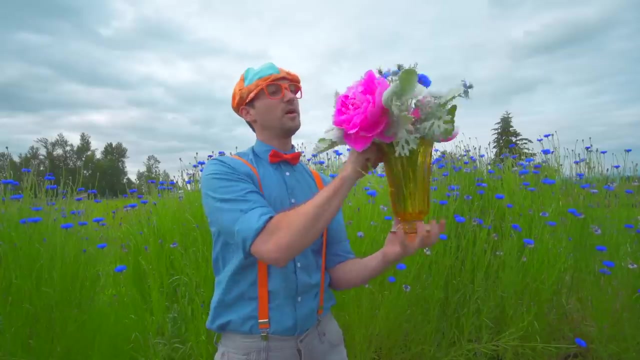 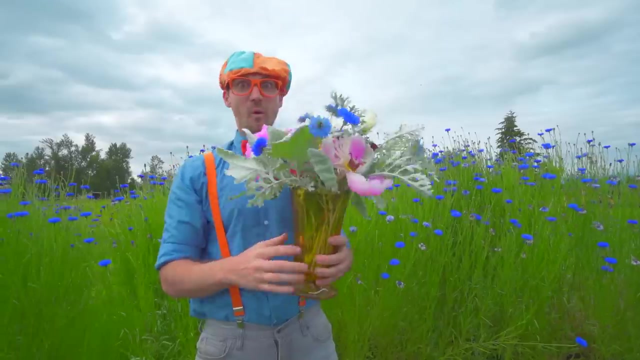 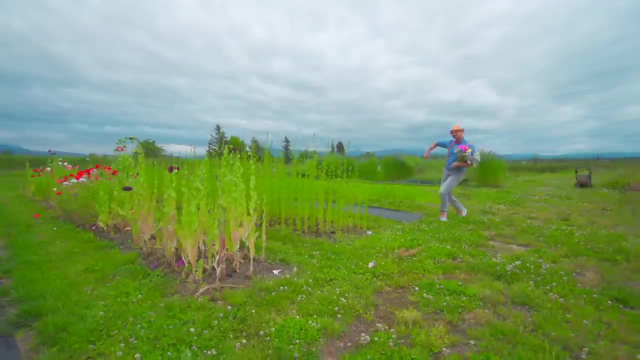 all right, here we go. how about one right there? how about one over here? how about one? let's see, right There looks beautiful, And one Right there, Whoa, What a beautiful bouquet. Let's go get some more flowers. Ooh, some more flowers.